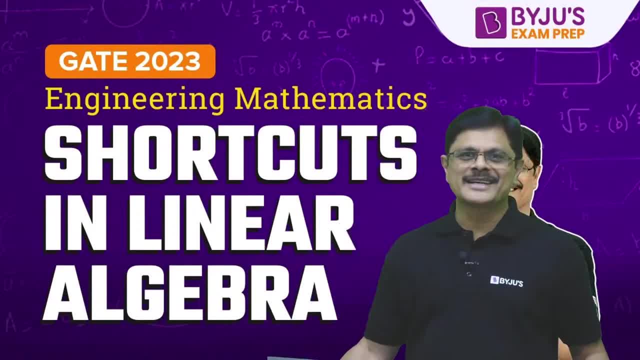 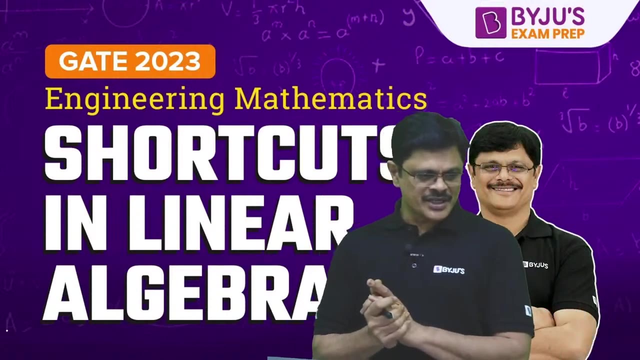 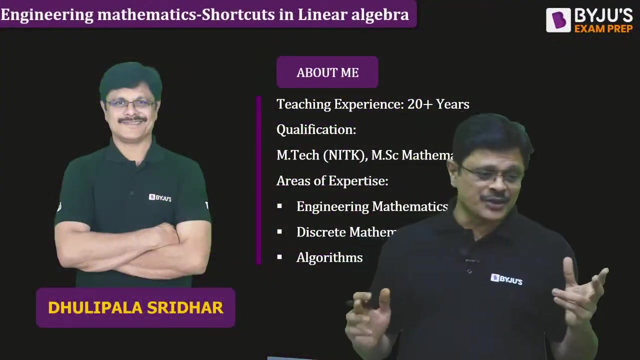 Hello, dear friends, Welcome to Baiju's exam prep And I welcome all for this special session of engineering mathematics where I'll be discussing the shortcuts in linear algebra. Hello friends, Good morning to one and all. Hope you're all doing well. So let us start the session, today's session, with shortcuts in linear algebra. my dear friends, And before that, this is about me myself, Sridhar Dhulipala. I'm having very good morning, sir. Very good morning. Ashok Pranab Paul, Very, very good morning. Okay, So, myself, Sridhar Dhulipala, I'm having 20 plus years of teaching experience and I'm associated with Baiju's 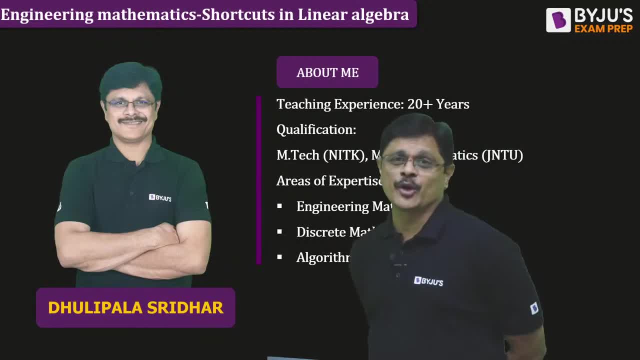 From past one and a half year, we were working on this particular project called Recorded Gate Content. We created visualized animated content for you. Hi sir, Very good morning Narsimha. It is first of its kind And under Baiju's exam prep app, the category name, note down: learn with video lessons. Very good morning. Love from Hyderabad. Same here. Okay, Good morning Payans Kumari. Very good morning sir. 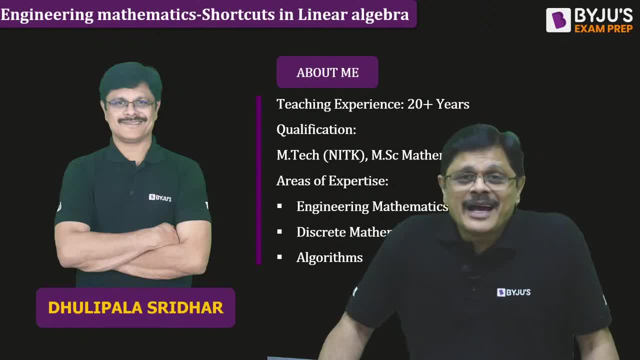 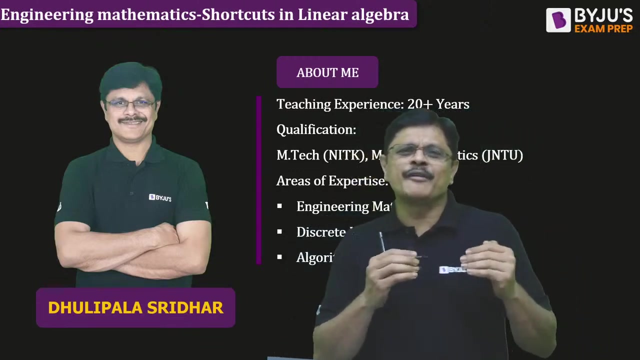 Okay, Under Baiju's exam prep app, the category name is learn with video lessons. You can find the subjects which were recorded by me: Engineering, mathematics, for all the branches. my dear friends, It was done in a very, very detailed manner, Okay, And we divided topics into subtopics, subtopics into small subtopics, like each half an hour to 45 minutes lectures. Okay, So you can go through those lectures under Baiju's exam prep app, my dear friends. 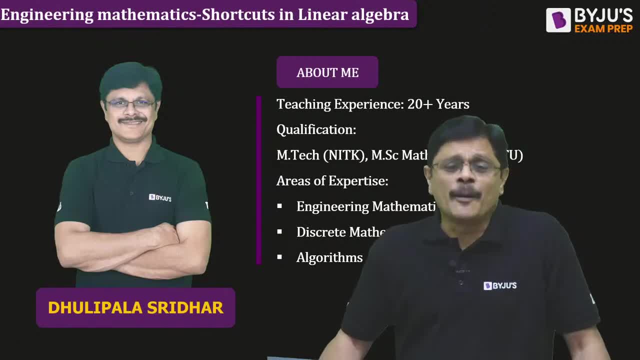 And not only that. I also recorded computer science subjects like discrete mathematics, algorithm C programming and data structures. Hi, sir, We'll plan. sir, It depends on your interaction or your regular attendance. Okay, If you are interested, definitely, Why not? I'll definitely come up with more such sessions. Yes, yes, I'm from Hyderabad. Yeah, you can attend everywhere, sir, Okay. 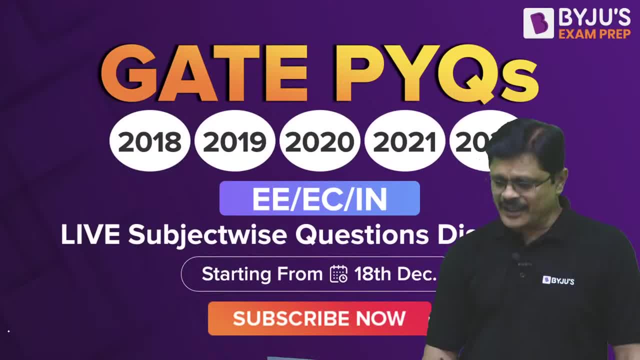 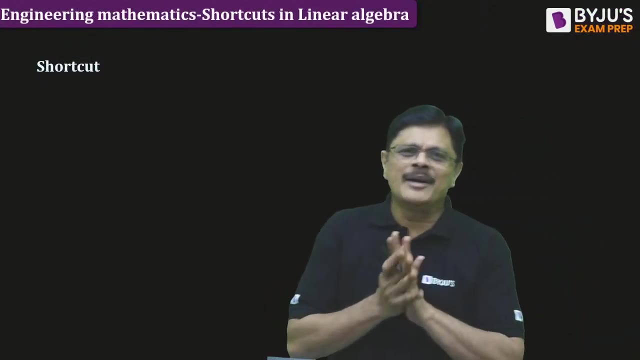 Right, sir. And there is one beautiful gate PYQ series happening for EEC and IN Last five years, previous gate questions for all branches will be. I mean, for these branches will be covered, Okay, Live subject: wise question discussions will be happening. Please do attend, my dear friends. Yes, yes, sir, Okay, So let us not waste our time. I'll be dealing with some very, very interesting shortcuts, Some of them you might be knowing. 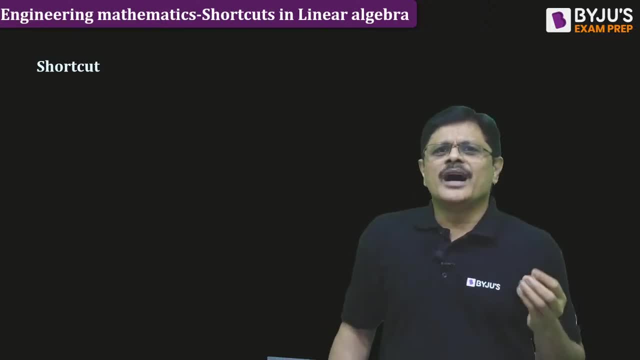 Some of them, some of them are new to you, but let us quickly do it so that you can revise the idea. my difference, suppose: if you already know it, you can revise it. if you do not know, you can learn it. so anyhow, it would be useful for everyone. see, for cs also will be coming up, sir. first let us have that for other. 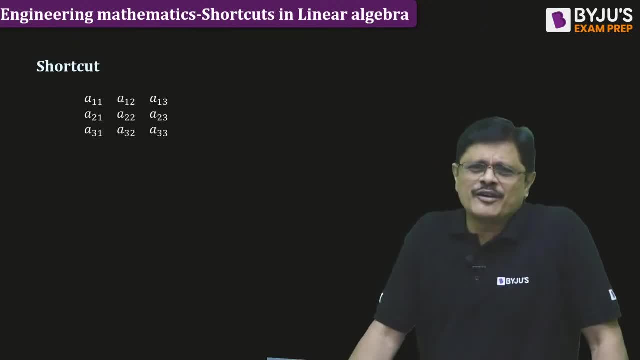 branches right. so the shortcut, the first one, very famous, determinant. now you are having a three by three matrix. actually, this shortcut is for three by three matrix only. this shortcut is for only three by three matrix only. but for other matrices of order higher than three by three we can use. 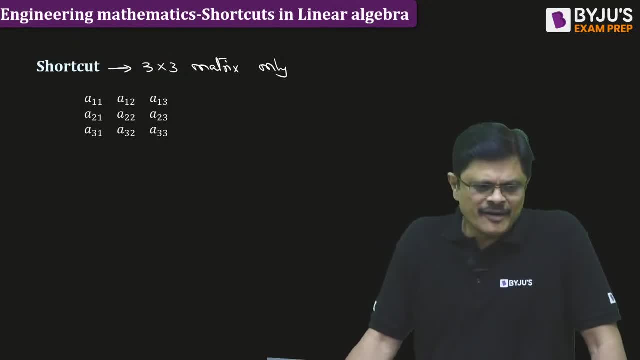 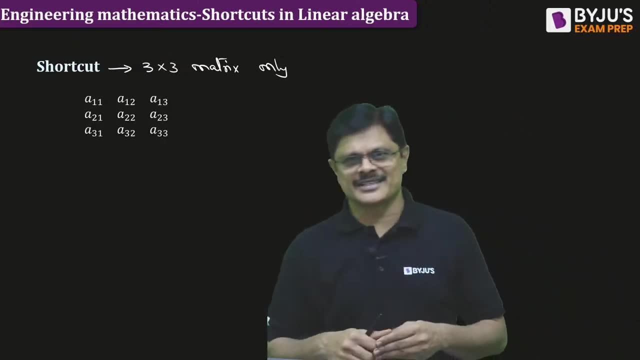 one more row operation technique that also i discuss in a while. first let us see the standard, very famous, well-known shortcut. there are two versions for this, both the versions i'll discuss, both the shortcut versions i'll discuss. okay, so whenever they give you three by three matrix, you can use one more row operation technique that also i discuss in a while. 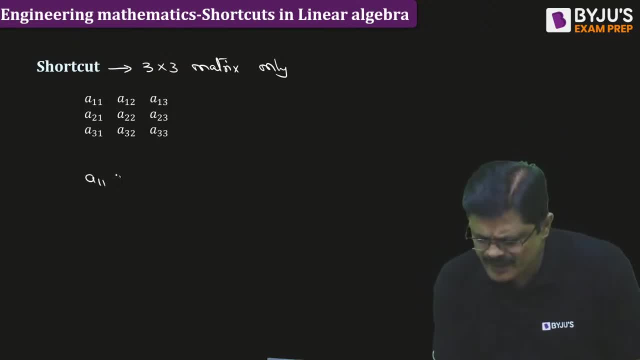 three matrix- first version is what you need to do is write down the matrix. as it is. what you need to do is. you all know, copy paste right, we are all experts in that. copy first two columns, paste after third column. copy first two columns, paste after third column. just do that. so how to do it? just write. 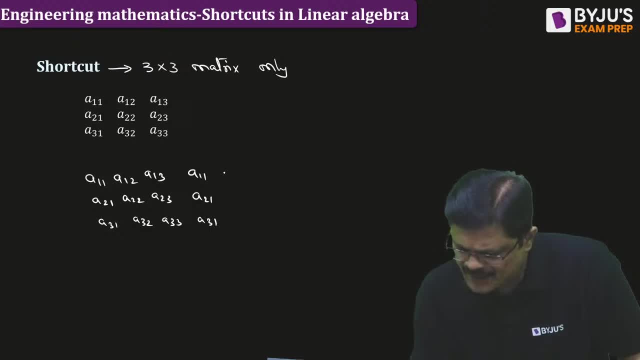 a11, a21, a31, a12, a22, a32. so then see. the shortcut technique starts here. what we need to do is we need to start with first diagonal. multiply the elements. the result will be having a plus sign. adjacent to that, there is one more diagonal again. multiply the diagonal elements, the next diagonal. 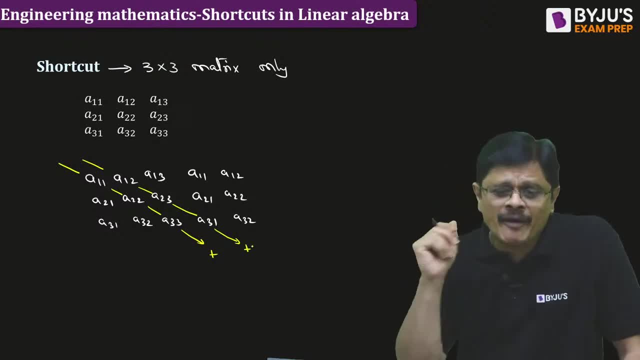 elements and the answer you have to give a positive sign. similarly, next diagonal is there. multiply the elements with a plus sign. now we do for reverse diagonal. for reverse diagonal the sign will be negative. so you have to go for reverse diagonal. you multiply them. whatever answer you get minus of the answer you have to take. 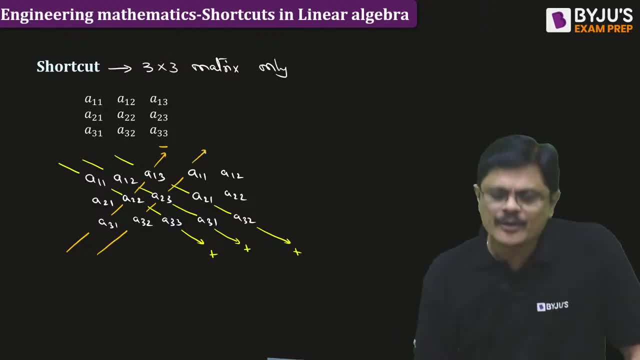 again. multiply these three elements. whatever answer you get, minus of the answer, you have to take it again. multiply these three elements after that, represented as straight, like this, from the answer you are taking. I think this is the easiest method. am I clear? no need of thinking, just blindly follow the procedure. you'll get the answer. 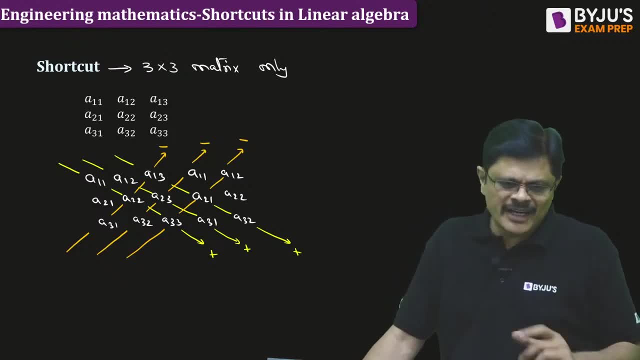 there is a small variant of this. there is a small variant of this. both will do the same work. said, the work is not different, only thing is the way it is written is slightly different. so next stage, there are three elements. you do the same work, slightly different. let me tell you the second version. you have to tell me which version you. 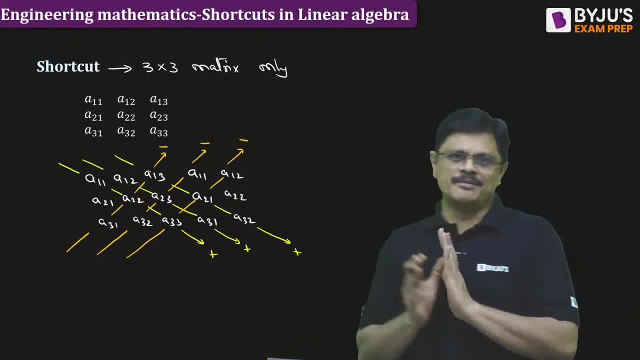 like I use that version to solve the problem. okay, this is first version. there is a second version of the same. what they do here is a11, a12, a13, a21, a22, a23, a31, a32, a33. so in this version, what they do is they just write this a11 after a1, three and this a month. 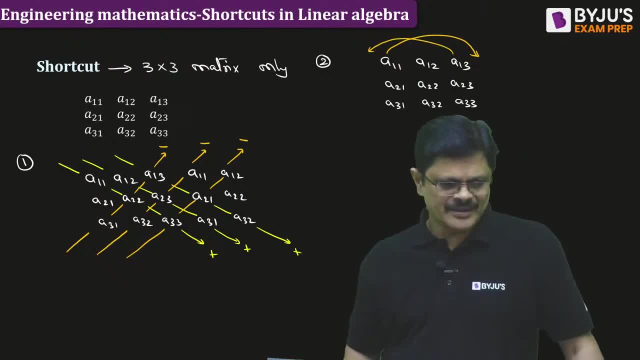 after, I mean before. even okay, Pradha, you already fix it, then no one can help it. you can follow it. so what happens? here is this: a1, 1 is written in here, a 1, 3 is written here and here a three. one is written after a three. 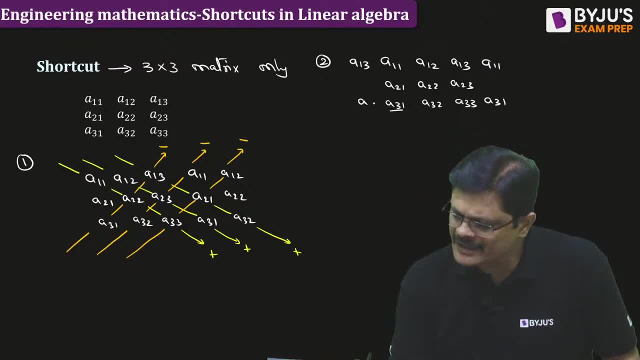 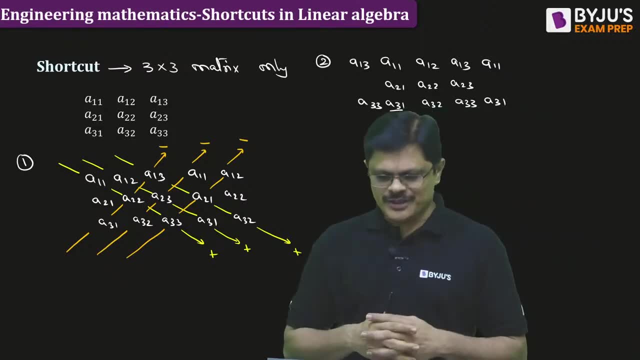 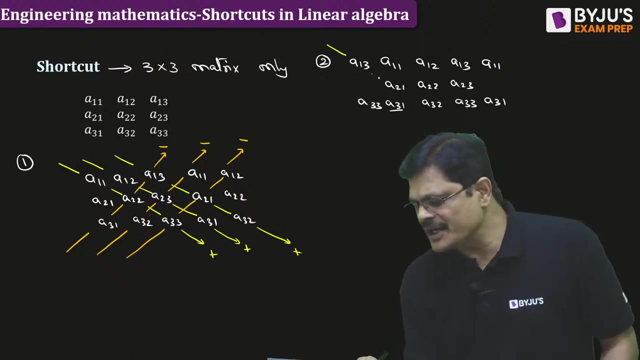 3, 3 and a 3, 3 is written before a, 3, 1, babu. so that is the simple story. now what we need to do, sir, again diagonals, same diagonals. you have to start from the leftmost: a 1, 3, a 2, 1, a, 3, 2. 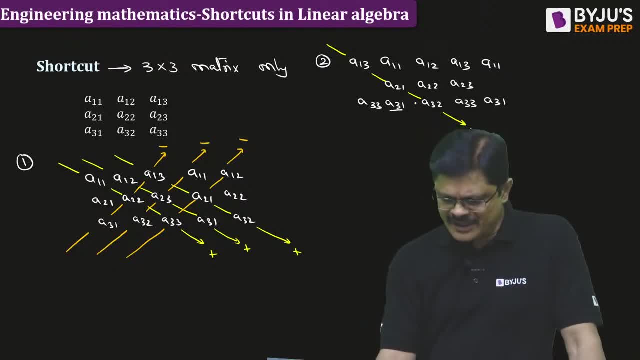 multiply them with plus sign. actually, if you observe a 1, 3, a 2, 1 a 1, 3 a 2, 1, a, 3, 2, same thing: the last one become the first one. that's it this: a 1, 1, a, 2, 2, a, 3, 3. earlier also you've done it. 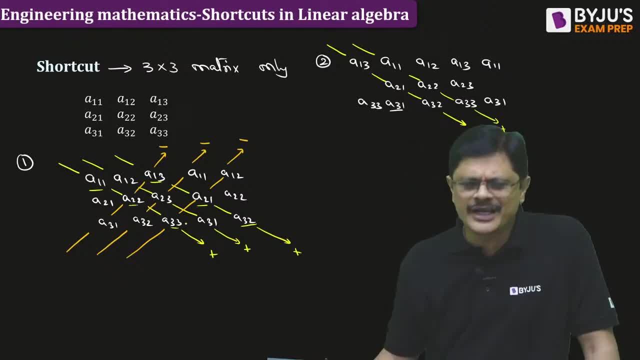 see the same one: a 1, 1, a, 2, 2, a, 3, 3. that also, you've done it. next one is: multiply. this hope you understand. wonderful, sir, that is very, very good. yes, babu, now when you go for reverse diagonals. 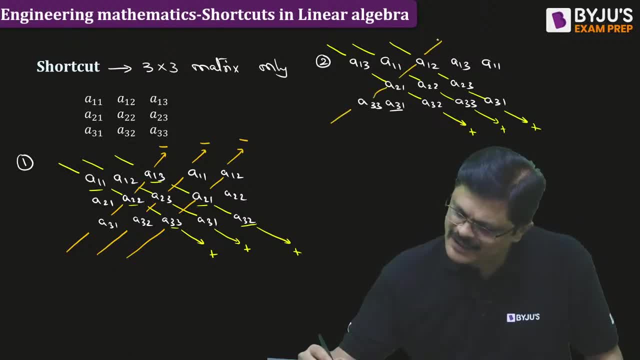 when you go for reverse diagonals, this with a minus sign. multiply these three fellows with a minus sign. multiply these three fellows with a minus sign. so these are the two versions of the same shortcut, but unfortunately this is only for three by three. see, most of the people are worried about the shortcuts, so that's. 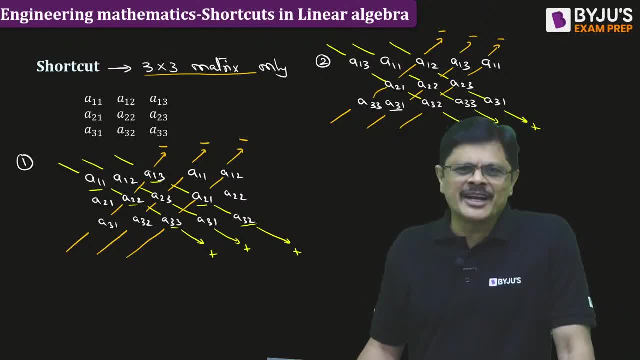 why today i just come up with the shortcuts. i'll be discussing some very interesting shortcuts, starting from determinant adjoint, then some more determinant shortcuts, then eigenvectors, eigenvalue shortcuts, LU, decomposition shortcut- everything within one hour. let us try to see shortcut should be done faster. no, so this session will go in a very, very rapid, fast manner. my dear 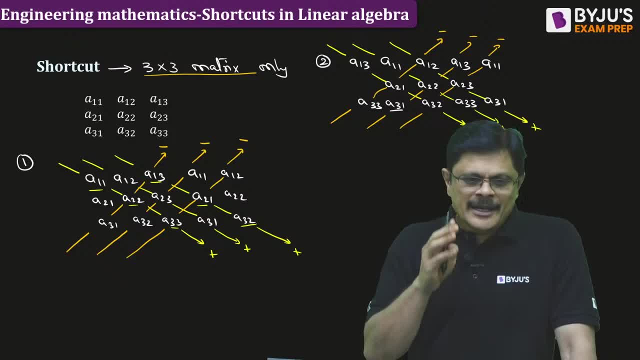 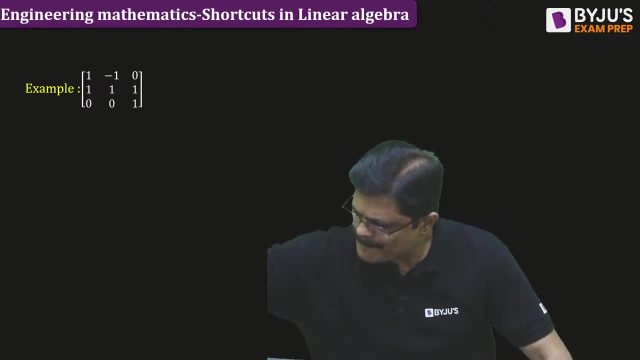 friends. so you are all ready for that. okay, be till end in one hour or so. we try to complete as many shortcut techniques as possible, so let us start this one second. ok, sorry, now look at this. if you want to apply this, what happens? so, according to this technique, 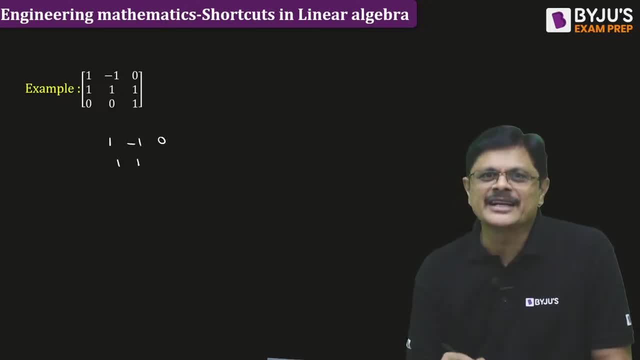 one minus one zero. of course there is a much better technique than this. just to understand the technique, you can take any numbers, you can do your own. you have to do it faster. shortcut trick. don't worry about how and all, you just apply. ok, don't think too much, it happens all. 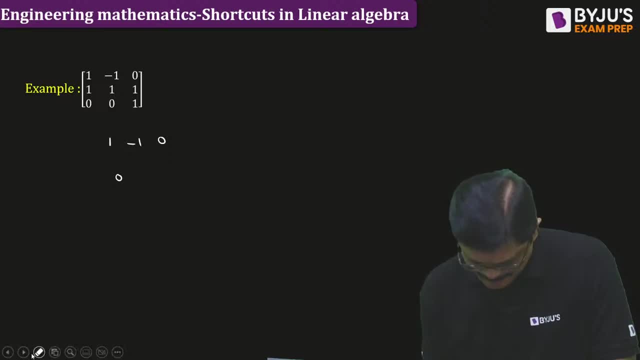 it will be completed: 1, 1, 1, 0, 0, 1. so here, first column, copy and paste. after third column, second column, also you copy and paste. so what happens? you multiply them 1 into 1 into 1 with plus sign, that is, plus 1, minus 1, into minus 1, minus 1 into 1, into 0, that is 0, then 0 into whatever it is. it. 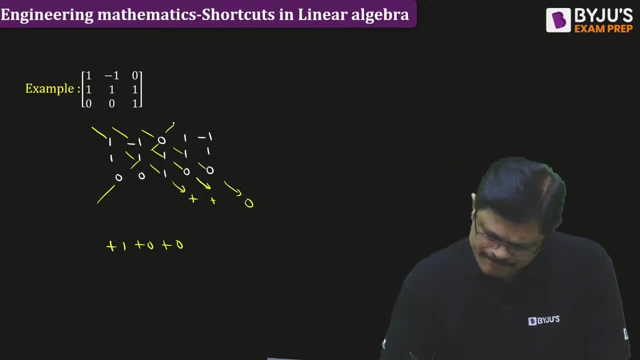 is 0, any home. reverse diagonal 0 with a minus sign. reverse diagonal 0 is there. so 0 is the answer and reverse diagonal there is a minus sign. actually product is minus 1, minus of minus plus. so here the answer would be 2. here the answer would be 2, of course, if you use the cofactor. 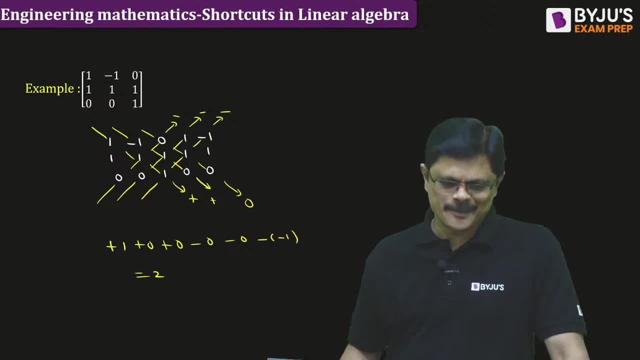 expansion. you get the answer much faster than this. okay, you can get the answer much faster than this. fine, we will discuss that in a while. now let us see the shortcut which is discussed, for it is not applicable for higher order matrices. remember now, there is adjoint. 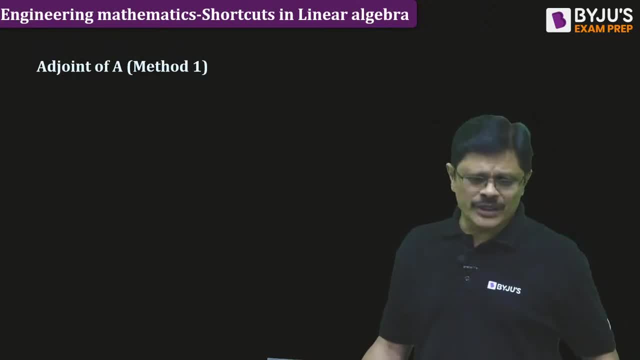 adjoint. adjoint also has 2 versions. let me give you both the versions. of course, both ultimately will do the same story. first version: matrices have been given very easily. write down the matrix and then first 2 columns, copy and paste after third column. copy first two columns and paste after third column. what else we do now in the new matrix? 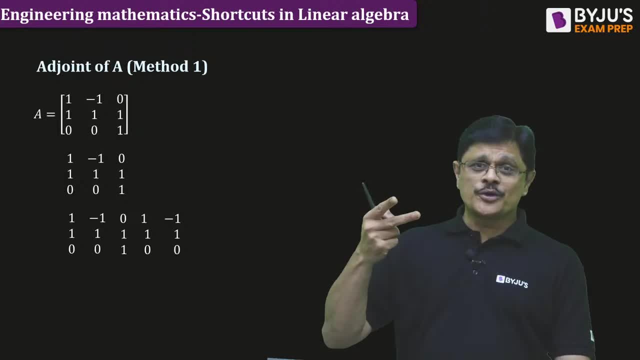 copy first two rows and paste in the third columns. it is text match new first column. always remember he has shown that he will copy and paste in the first column first two columns- he has rows and paste after third row. Hope you understand: Copy first two columns, paste after third. 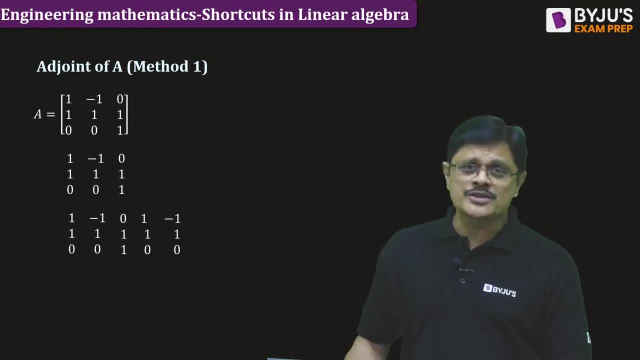 column In the new matrix. copy first two rows, paste after third row. This is your new matrix, Got it? Now what you do? Cancel out the first column. cancel out the first column. Now, here we have four columns. We manage these four columns to get adjoint. my 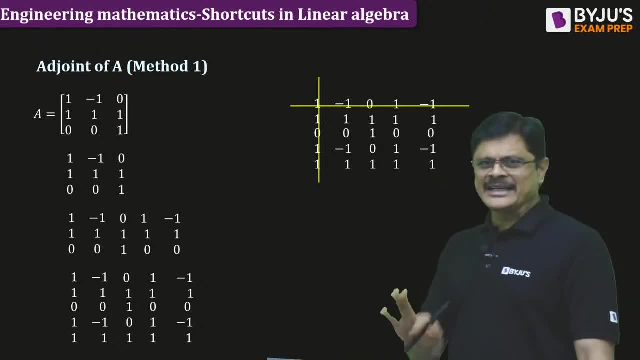 difference. To get adjoint, we have to manage these columns. I'll tell you, because let us see the second method also. Ultimately, the same thing you are going to get with second method also. So whatever method you like, you can use it. Yeah, it is also for three. 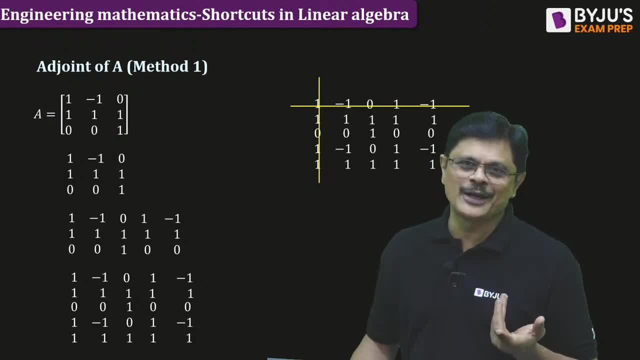 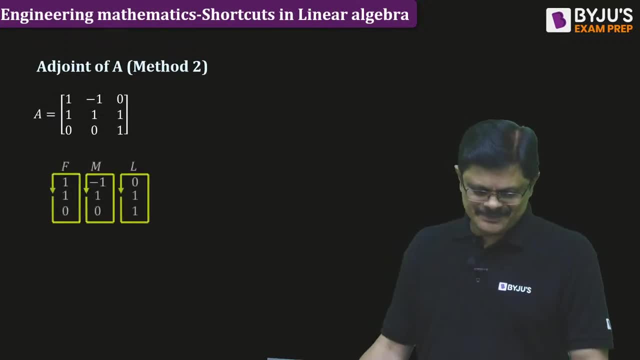 by three only. It is also for three by three. only my difference. Okay, So what we need to do, Take the matrix Now here, middle to middle. The story goes from middle to middle, my difference. Let me explain that middle to middle technique. So here, what they do, This is, you know. first, 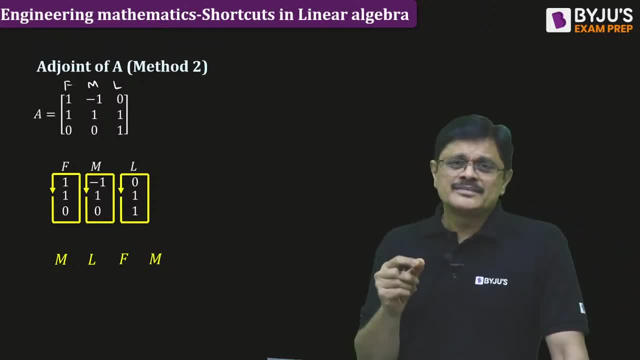 middle and last, See middle column from middle element. you have to start and you have to fill up to middle element, middle to middle. That is middle element. last element, first element, Then middle, middle to middle, circularly, from here to here, circularly. how to fill? 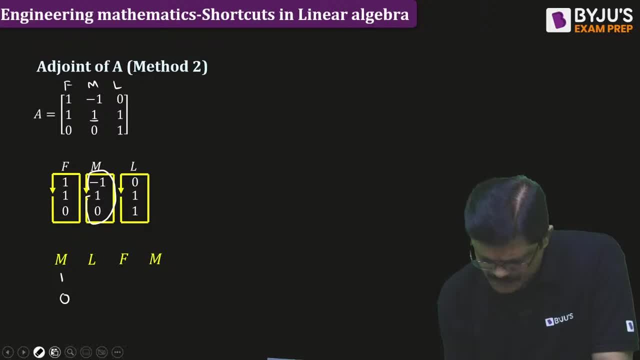 the blanks. Hope you can do it. Hope you can do it. Correct Now. last, also middle to middle, Everything middle to middle. Last also middle to middle. One, one sunya one First, also middle to middle. What is it One sunya one? one Now middle, already done, You can copy. 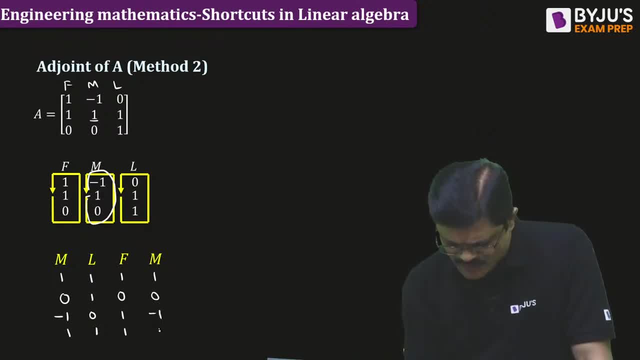 the first column again One sunya minus one one. So actually, if you observe, after removing the first row and first column in the previous one, in the previous example, whatever you seen, you have seen this. no Previous slide. I will show you previous slide. 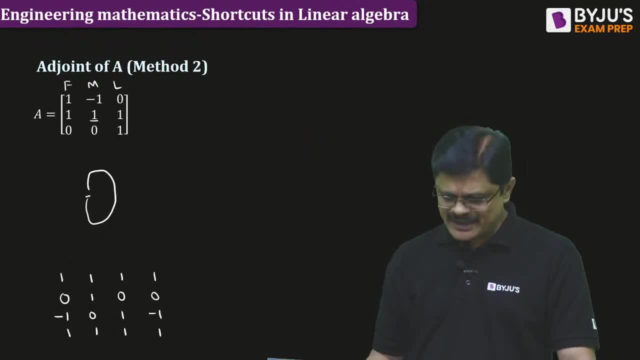 Method one, Method one. whatever you get it here, the same thing by this method directly, you will get it Directly. you get this form Directly. this form, if you observe, without removing any row and column, you can directly get it. That is the advantage of this method. 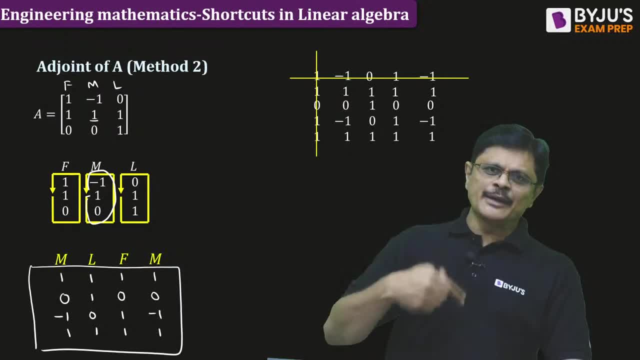 Middle to middle method. Okay, You can start from middle. Everything we are going to write from middle to middle, Middle to middle. That is first. we start with middle. Middle element to middle element. Last middle element to middle element. First, middle to middle Middle. 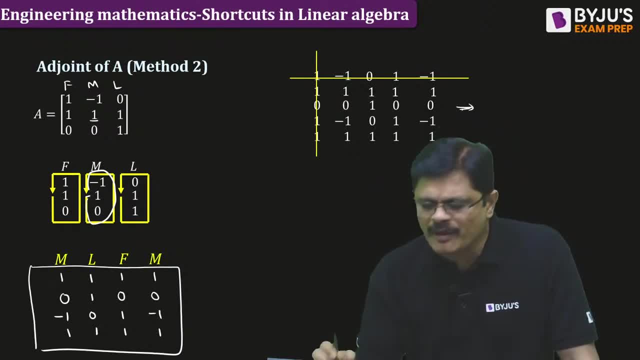 middle to middle. So by this, what happens? Automatically, you get this four by four form and you can manipulate this. Yes, yes, You can manipulate this to get the adjoint by difference. Let us see how to write the adjoint. Let us see how to write the adjoint: See by both. 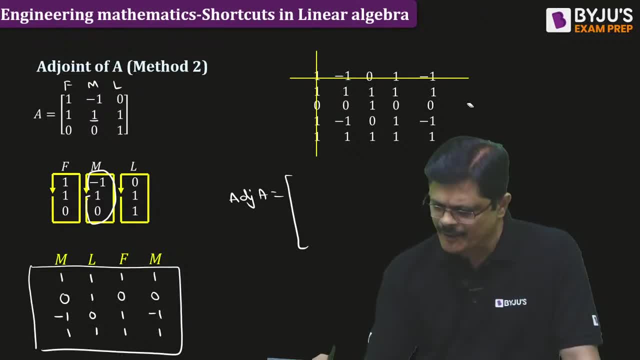 the methods. this form, you are going to get it. By both the methods, you will get the same form. By both the methods, you will get the same form. Okay, Now let us see how to apply this method. Let us see how to apply this particular method. my dear friends, Now 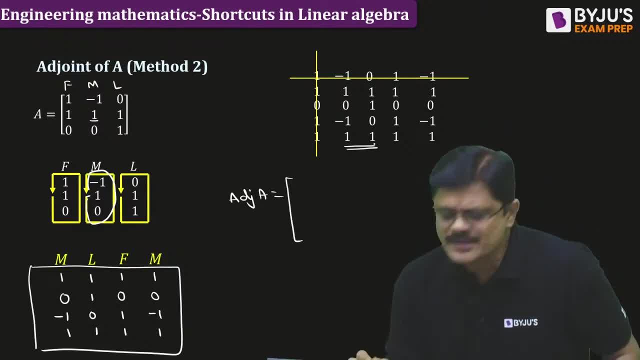 look here What we do Here you see first two columns. You can make two by two determinants. See here we can create Two by two determinants. See clearly, You can make two by two determinant, Two by two determinant, Two by two determinant. So find these two by two determinants from the first. 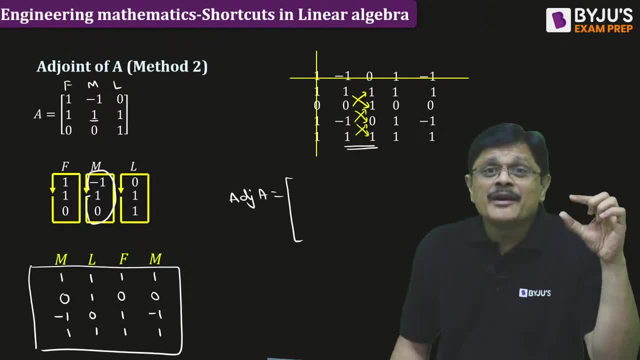 two columns Column wise, Then paste the values or write the results row wise, That is, calculate column wise, but write row wise to get adjoint. So you calculate: one minus zero, That is one Zero. Zero minus zero, That is zero Minus one. Minus zero, That is minus one. So you calculate: 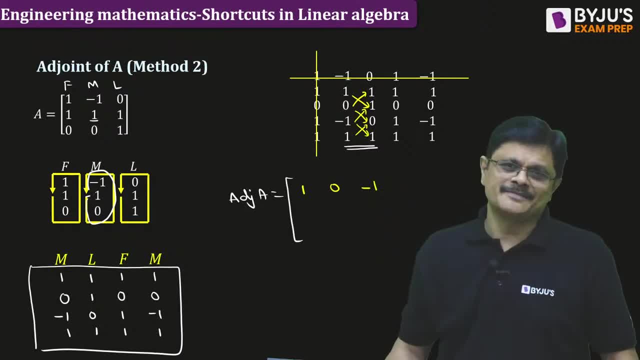 column wise but paste the results row wise But paste the results row wise. Suppose if you calculate column wise and paste column wise only, you get cofactor. If you write in the same order, you get cofactor. Suppose you want cofactor, you write in the same order. 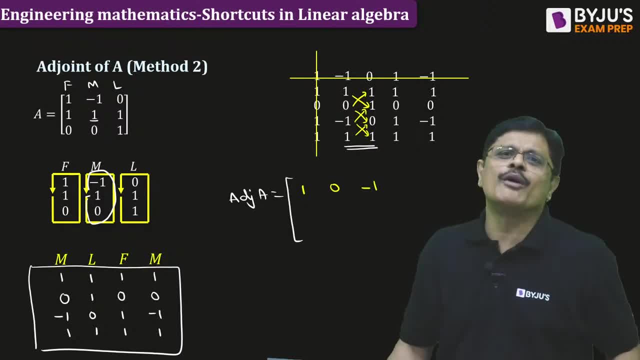 But if you calculate column wise but put it in row wise, what happens? You get adjoint, Because we are interested in adjoint directly. So we do this. So we do this. Hope you understand. Same story again. we will continue, sir Column. 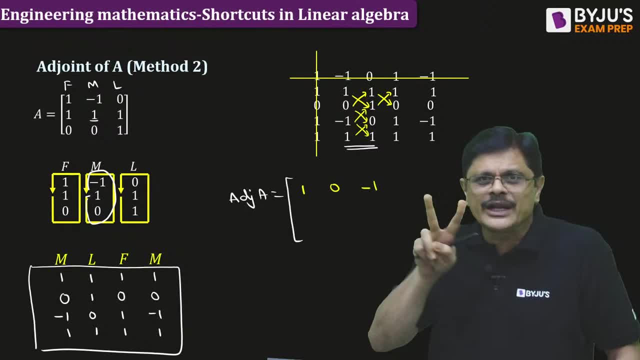 wise for the second two columns, That is one, two completed. Now take two, three columns: Zero minus one, That is minus one. One minus zero, That is one. Soon you minus one Minus one, Done. Now third and fourth columns: Story the same. 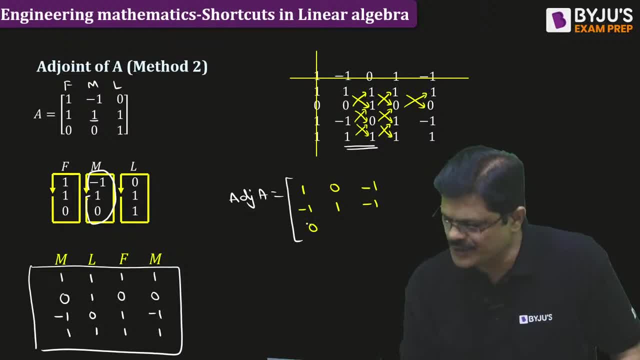 Schoen minus schoen, Schoen, Absent days. Schoen minus schoen, Schoen, Absent days. One minus of minus plus one, That is two. And this is how we get the adjoint, my dear friends. So this is a. 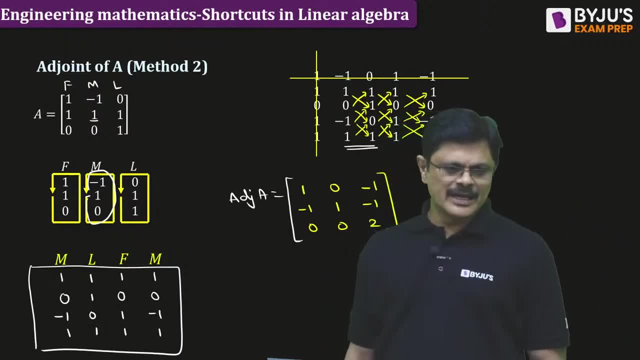 shortcut for adjoint. Hopefully you understand the adjoint shortcut Is the idea clear, But one should always understand: Adjoint meanstranspose of the cofactor. Adjoint means what sir Transpose of the cofactor factor. that is very, very important. adjoint means what sir transpose of the cofactor and if you know, 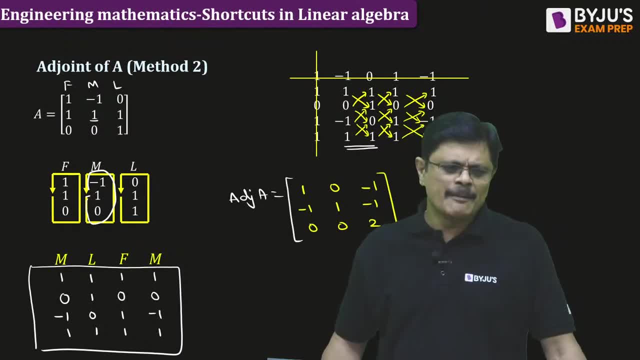 how to find cofactors. you can do much faster than this, but people are interested in what is the first row, middle one. any mistake? 0 minus okay. it is 1 minus 0 minus 0. sorry, 0 minus. this one is wrong, right, yeah, yeah, it is 0 minus of minus plus 1. yeah plus 1. it is yes, yes, yes, yes, ha, ha, ha ha ha. 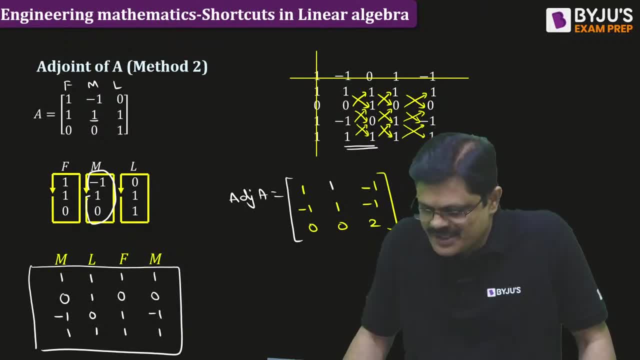 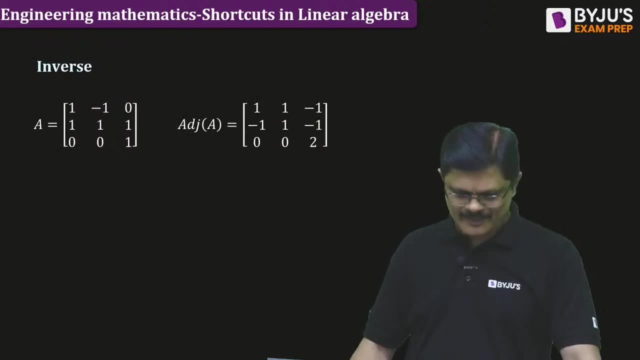 right, correct, you are correct. my dear friends, you are correct. hope you understand. hope you understand, oh god, yes, yes, yes, correct, all nice. now, after finding adjoint and a, you can find a inverse, the formula for a ace versus adjoint: a by detail, adjoint a by data. e is A inverse minus. 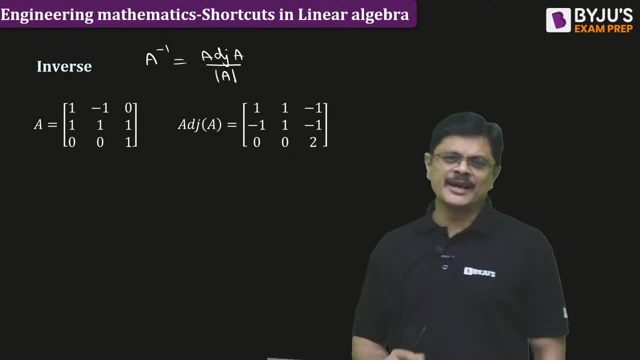 now. now if you are having and adjointy, if you are having a end age on A, can you directly find determinant from this? can you find determine from greater or from greater? I you check, i did a. you can go ahead and think about it from this directly I know A and I know adjoint A. Both are given to me. Can you find determinant? 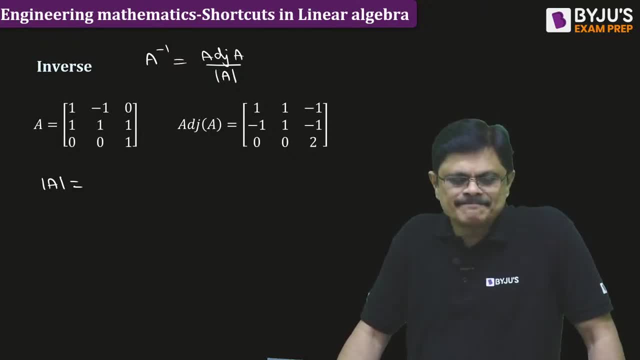 Can you find determinant? if I know A and adjoint A, Can you find determinant? sir, See my difference. If you take the first row of A, the cofactors of first row will be here. These are the cofactors, because adjoint is. 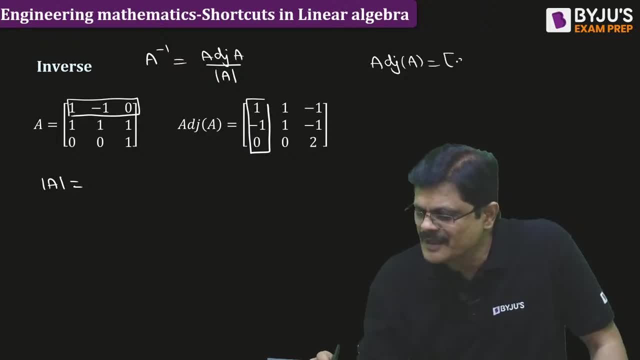 transpose of the cofactor. Adjoint is transpose of the cofactor matrix, So any row elements or any column elements. if you multiply with corresponding cofactors and add, you are going to get determinant. Yes, adjoint A is transpose of cofactor, So any row elements. 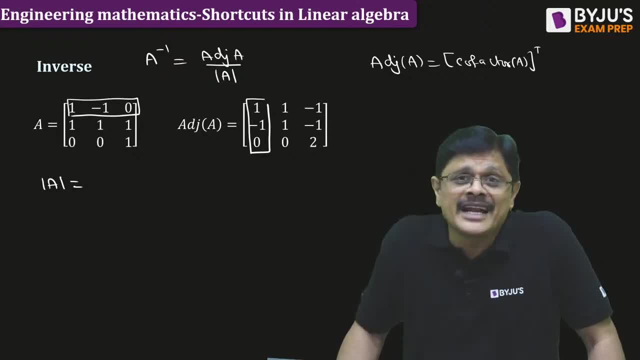 or any column elements. if you multiply with corresponding cofactors and add, you are going to get determinant. That is what we call it as Laplace equation Expansion. So actually, if you want to get determinant in this particular situation, you can directly multiply 1 into 1, minus 1 into minus 1 plus 1, 0 into 0, 0, which is 2.. 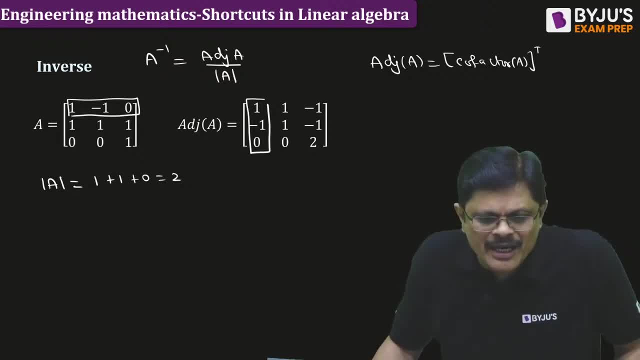 Babu zero kaadu mani Babu Payash Kumar, Not first row with first row, Not first row with first row. First row with first column. First row with first column. Babu, Ah, James Bond, James Bond. 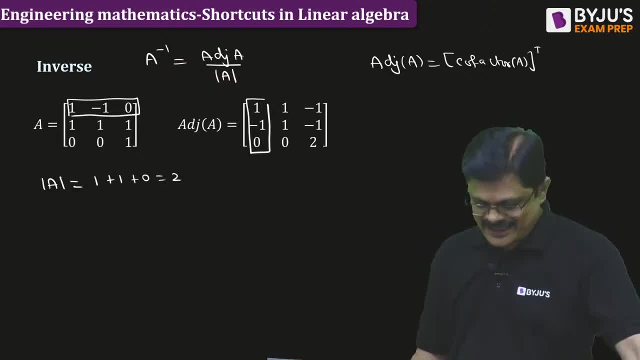 Okay, James Bond given correct answer, Babu, Please remember. So that is it, So you can find determinant. Once you know determinant also, you can find A inverse Babu. What is A inverse? 1 by det A, that is 2, into adjoint A, That is 1, 1, minus 1, minus 1, 1, minus. 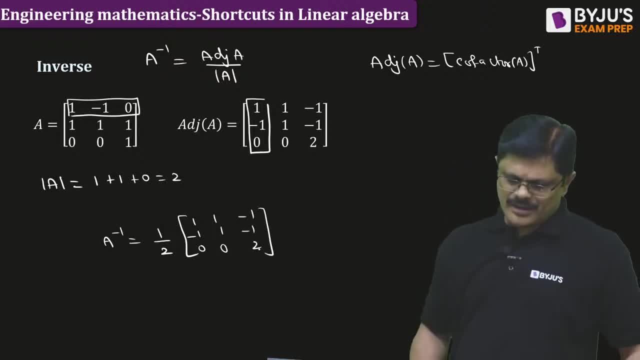 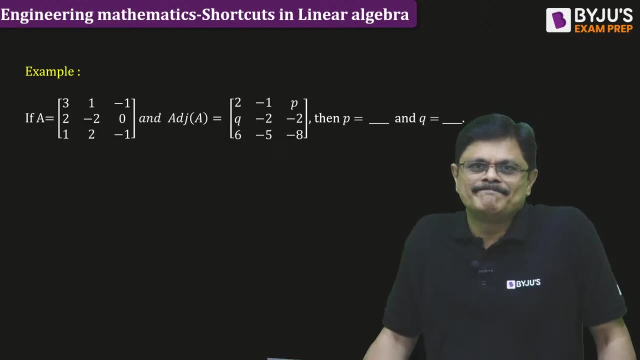 1, 0,, 0,, 2.. So that is A inverse Babu. Now comes the most interesting stories. I gave an A, I gave an adjoint A. I want you to find PQ, That is in adjoint A. only two elements. 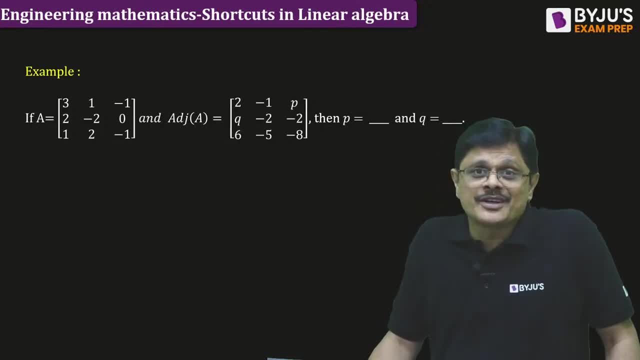 are missing. You need to find them. This was a great question, not my personal question. I need to find P and Q, which are missing. Are you going to use the entire procedure which we done: Copy first two columns after second column, paste first two rows after. Are you going to do that? 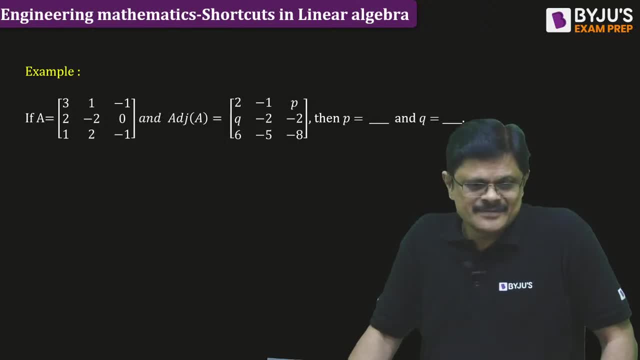 There should be some much easier technique than that. Okay, One is: if you know cofactor idea, that is much easier. or you can use determinant idea. Just now we know one very interesting idea which is determinant. See, it is A and it is adjoint A. It is A and it is adjoint A, Correct or not? Any row multiplied with 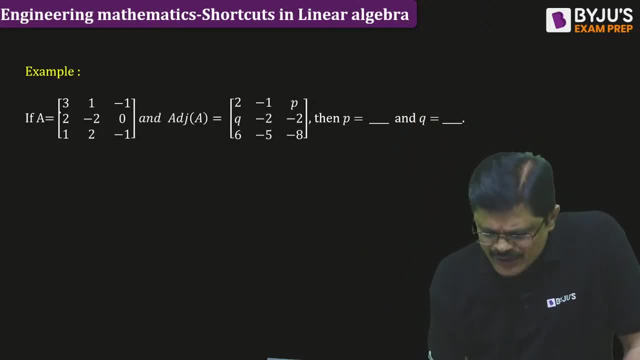 corresponding cofactors will give you determinant. Okay, So here this is second row, multiplied with corresponding cofactor will give you determinant. So what is determinant in this case? what is determinant in this case? 2 into minus 1 minus 2, minus 2 into minus 2 plus 2. 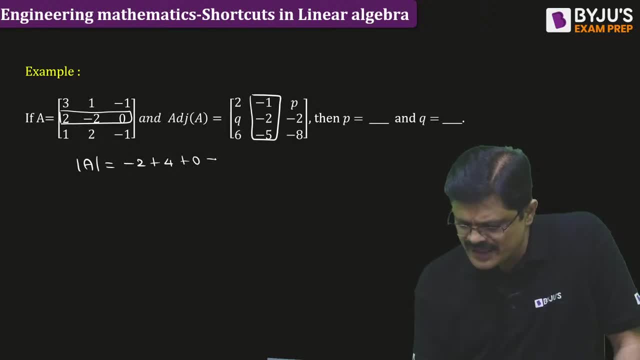 and shun yin. 2 minus y is shun yin, so that is equal to 2. so here determinant is equal to 2 for this matrix. my difference: you can do that, compare determinants. very good, james bond, you are rocking. i'll give you much easier than much easier technique than that. but first let us see. 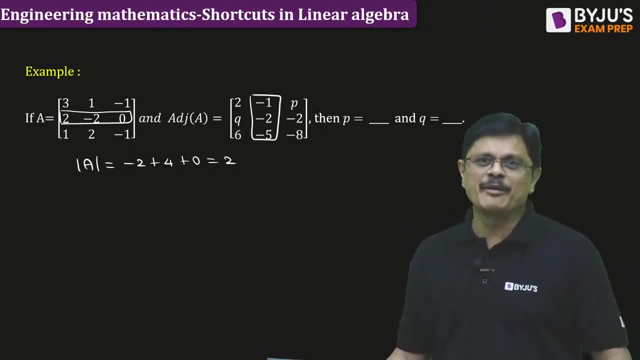 the thing which most of the people follow. most of the people follow this technique, so let us use it now. even if you multiply first row with first column also, you get determinant. so determinant can also be obtained by multiplying first row elements with first column of x joint here that. 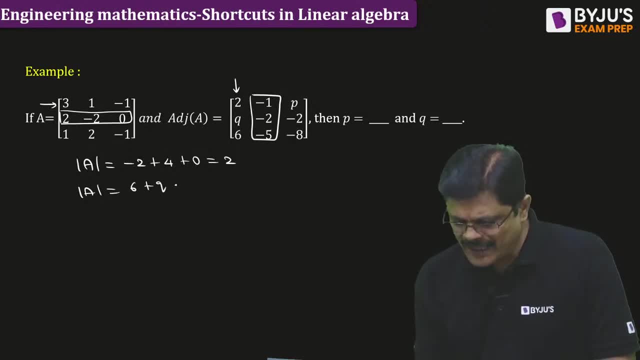 is 3 into 2, 6, 1 into q, q minus 6. that should be equal to 2, because determinant is already fixed. therefore, what should be equal? what should be? the value of q, babu, the value of q is equal to 2. 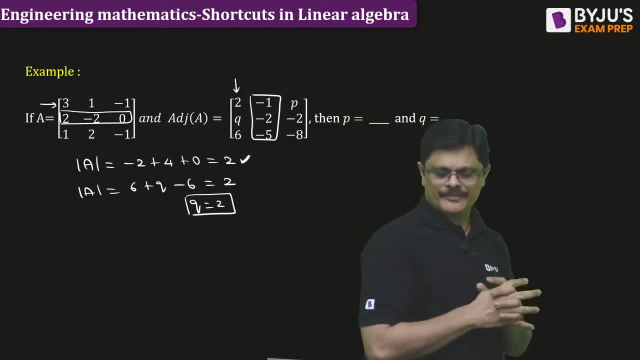 the value of q is equal to 2, we don't even have to use the shortcut. similarly, third column, or sorry, third row multiplied with third column also gives you determinant. third row multiplied with third column also gives you determinant. very good babu, very good sir. so what is it? 1 into p. 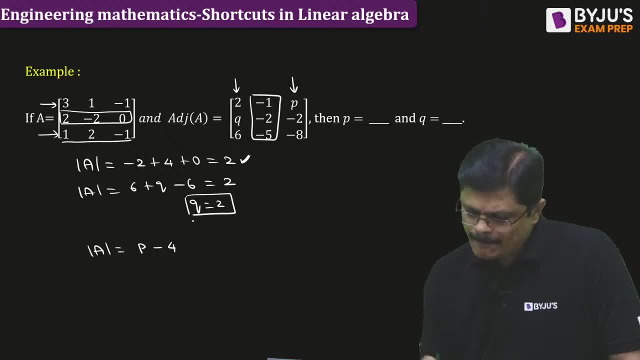 2 into minus 2, minus 4, minus 1 into minus 8 plus 8, and that should be equal to 2. therefore, what is the value of p babu? p value is, i think, minus 2 right. p value is minus 2 because 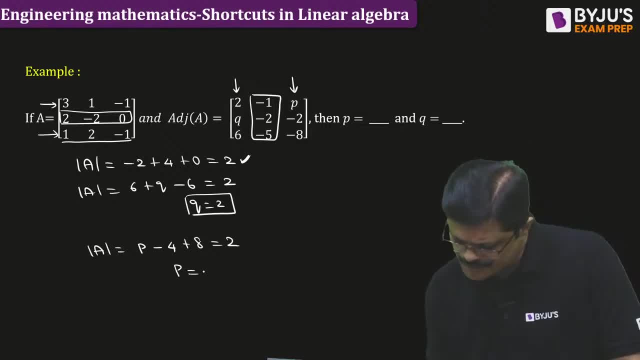 p plus 4 is 2, p is equal to minus 2, but you can do much easier technique than that if you know what is cofactor. of course, if you don't know cofactor, i cannot help you in that. okay, so now look at this: my 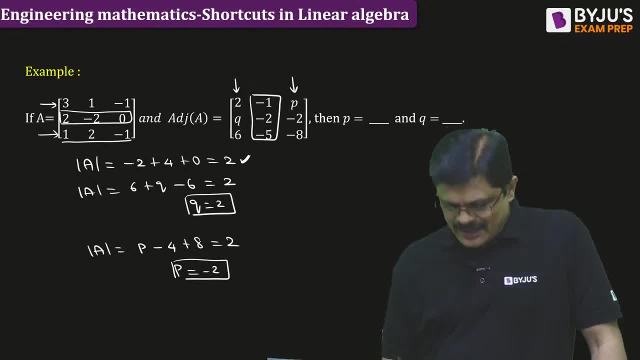 points. look at this: if you know cofactor, see adjoint is what, sir? what is adjoint, sir? adjoint is what transpose of cofactor. adjoint is transpose of cofactor. so the adjoint elements are actually obtained by transposing the cofactors, transposing the cofactor matrix. so this p, which is actually 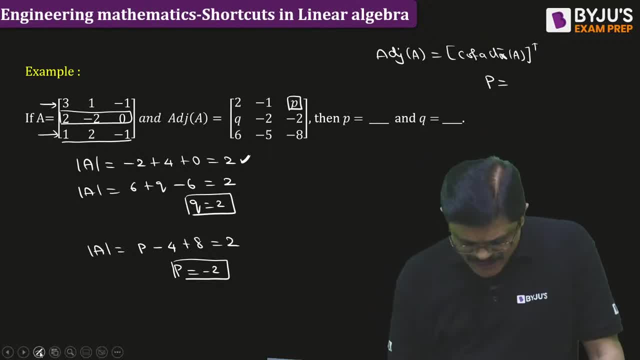 element of adjoint. element of adjoint which is actually what is the row number and column number of P. P is third row, for sorry, first row, third column. P is actually first row, third column element. P is first row, third column element, so it should be actually cofactor of third row, first column. this fellow. 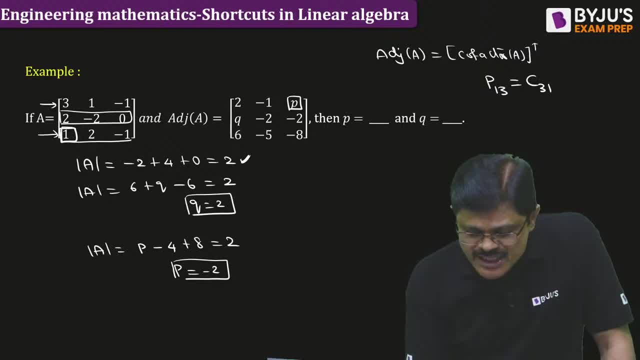 must be cofactor of third row first column element. so just find cofactor of this, you will get the answer. just find cofactor of this fellow, you will get the answer. what is cofactor of that fellow sign will be plus sign and minor of third row first column. remove the third row. remove the. 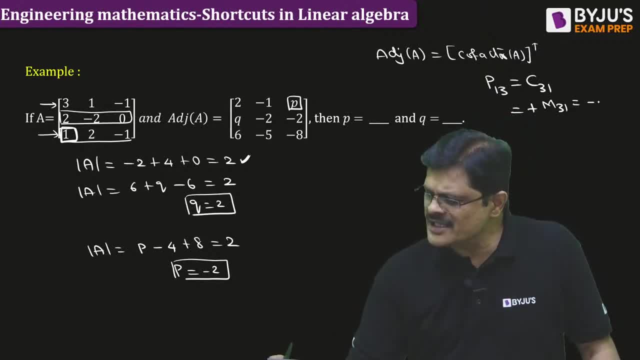 first column one minus two. so the answer is minus two, my difference, and you got the answer by this method. so this is much better than that. that is basic concept. actually, adjoint is transpose of cofactor is much better shortcut than this. similarly, Q is actually second row, first column element. 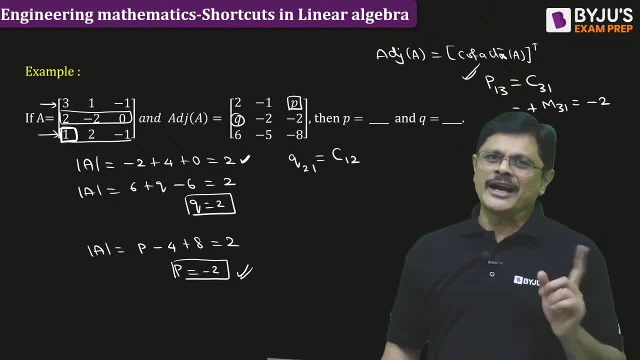 which is actually cofactor of first row, second column element. so this is the cofactor of first row, second column will have minus sign and minor one, two. remove the first, remove the sorry, remove the okay, it is first row, second column. now this fellow's cofactor. 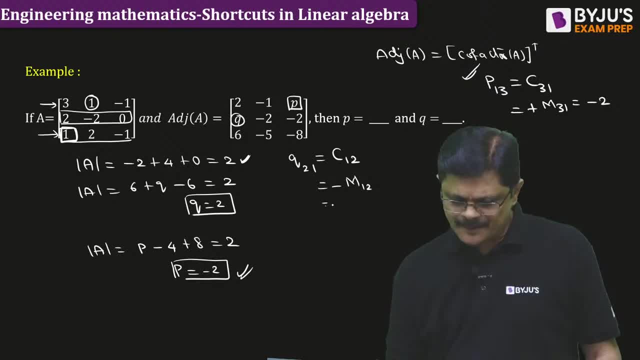 remove the first row and second column. determinant is what, sir? it is minus two. minus of minus two is plus two. so like this also, you can solve it. this is much easier technique than that, but mostly I think people follow this: your wish. anything is fine for me. 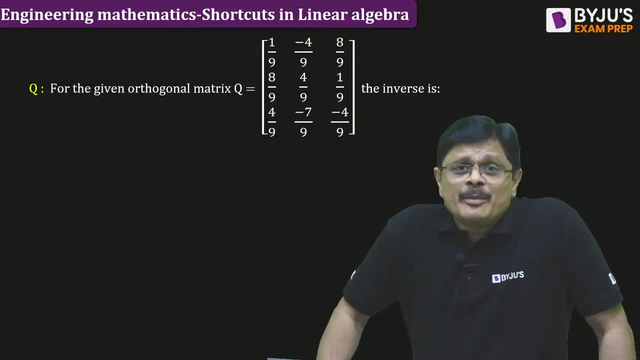 now one more very interesting question. this question was asked in gate many times. at least three, four times this question was asked in different ways. same question was asked different ways in gates. that is, if a orthogonal matrix is given, you need to find inverse of this. you need to find inverse of the matrix. 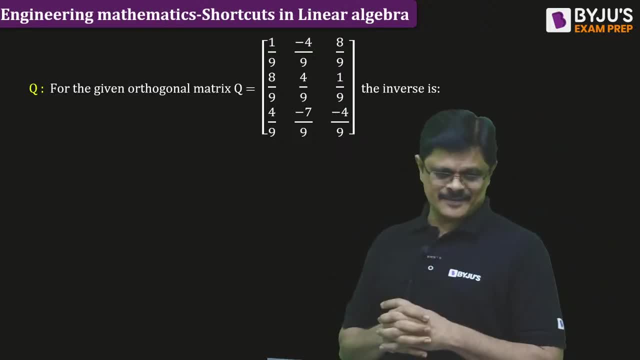 if orthogonal matrix is given, you need to find inverse of the matrix. so are you going to do adjoint Q by dead Q? are you going to do for Q inverse? actually, Q inverse means adjoint Q by dead Q. if you do this method tomorrow morning, you will get the answer. but those who know that orthogonal matrix is a matrix- 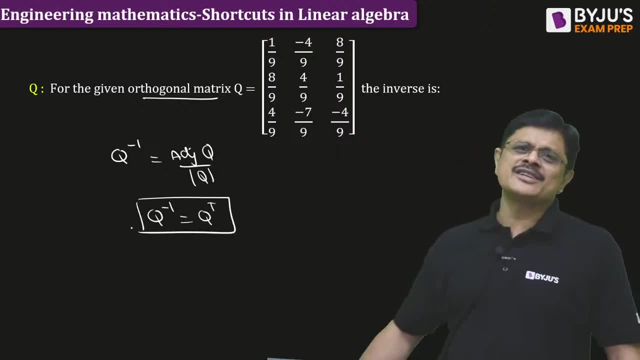 which is defined in such a way that the inverse of the matrix is equal to transpose of the matrix. so you just need to find transpose of the matrix. this was a gate question. please see this. my def: just find transpose rows converted to columns. columns converted to rows. 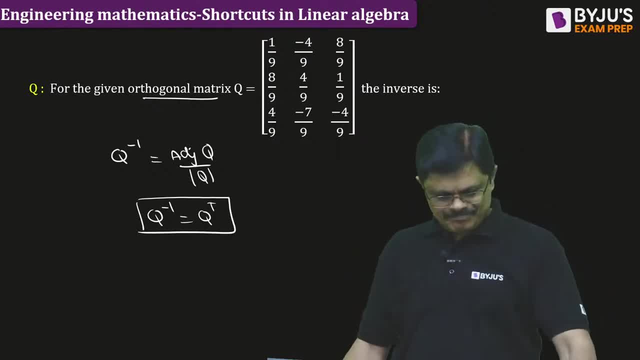 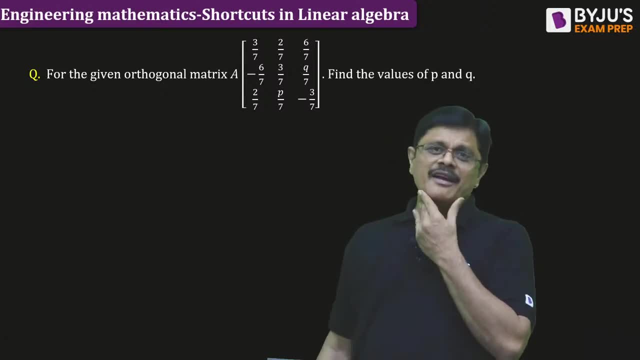 you will get the answer within no time by defects. one more question. even this is wonderful. result: we are having an orthogonal matrix. matrix is given and it is saying that he is saying that it is orthogonal matrix. in this there are some numbers missing: P, Q, something like this. they are missing some. 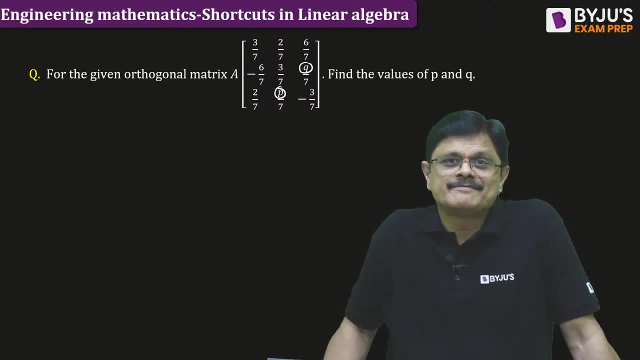 Now you have to find what is p, what is q. Now there is a wonderful property about orthogonal matrix: The columns or rows. columns or rows form orthonormal. set What they form, sir, They are orthonormal. The columns are orthonormal, See. orthonormal means length of each vector. 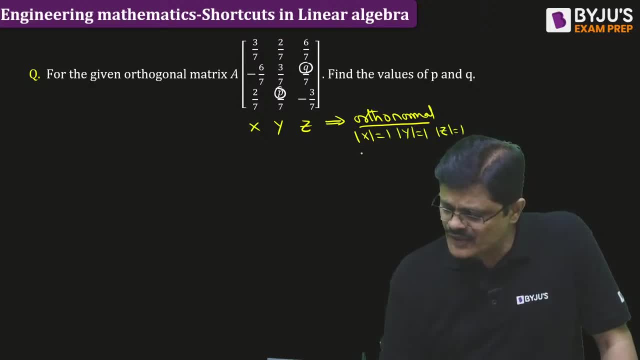 is 1.. Length of each vector is 1.. And dot product of any two different fellows is equal to 0.. Dot product of any two different column vectors is equal to 0.. Those who know this property. this problem can be solved within no time. Am I clear? So I just use this idea. 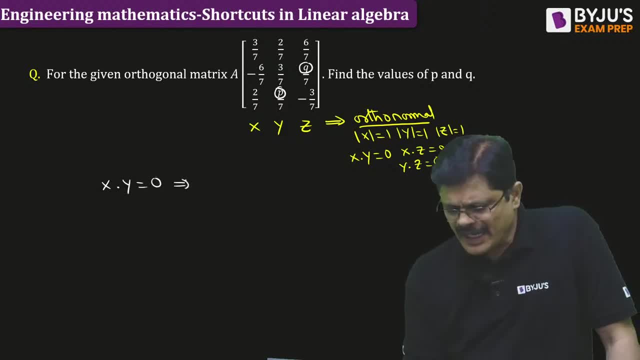 because x dot y is equal to 0.. I just find dot product of these two fellows and I am going to solve this problem. So I am going to solve this problem. So I am, And equate it to 0.. 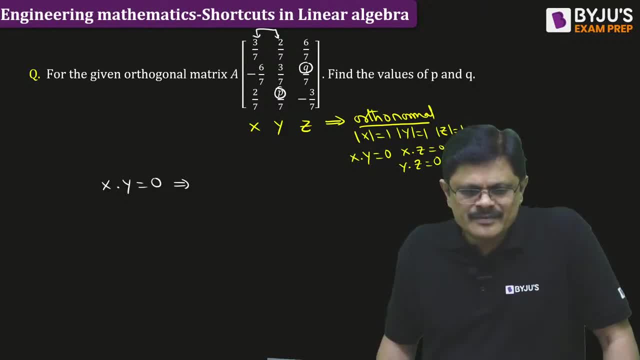 From that I get the value of P 7.. Yes, Pranab Paul, See this. Pranab Paul, always, you know. You can just read the comments of Pranab Paul And you can understand what I am saying. So what I take for 10 minutes or 20 minutes, 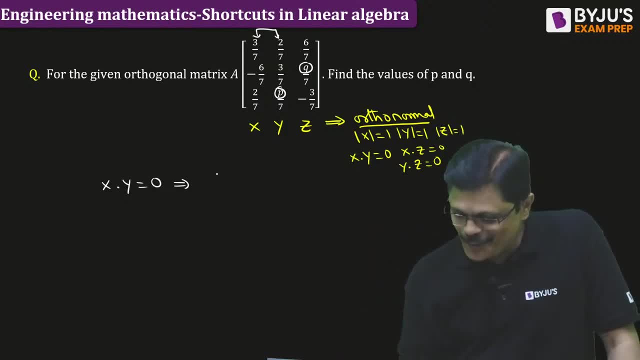 He will write within no time. So what happens? Denominator 7 into 7, it is 49, always Numerator 3 to 6 minus 18 plus 2 P, And that is equal to 0.. So the value of P is what sir? 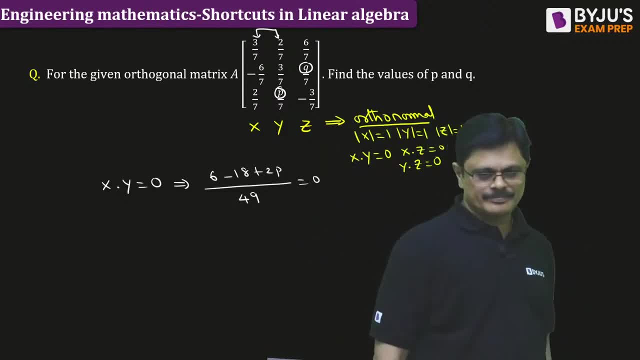 What is the value of P? What is the value of P? I think you can solve it now: 2 P plus 2, P minus 12 is equal to 0. Therefore, P value is equal to 6.. Where, Similarly, find out Q value? 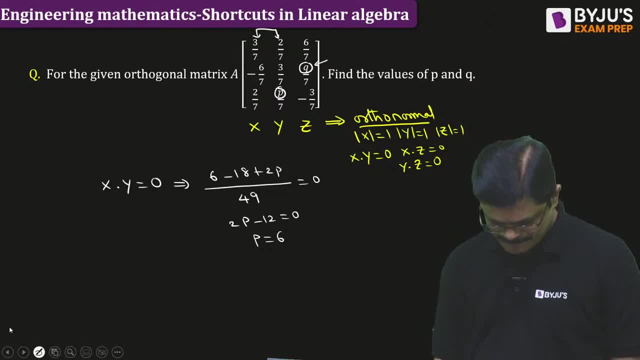 Q value. you have to find. You have to find Q value. What is the value of Q, my dear friends? 6 or minus 6.. Check carefully, Please check carefully. Maybe May not be, But whether my student or not, 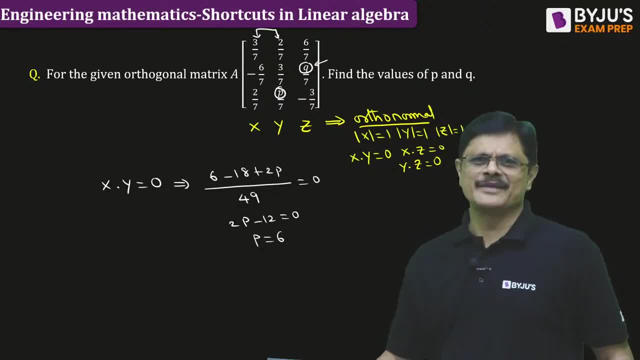 If someone do well, he is doing well. That is it right. They can learn from anywhere. They can do well. What is wrong in that? Okay, See, here I can use X dot Z again. I use X dot Z, my dear friends. 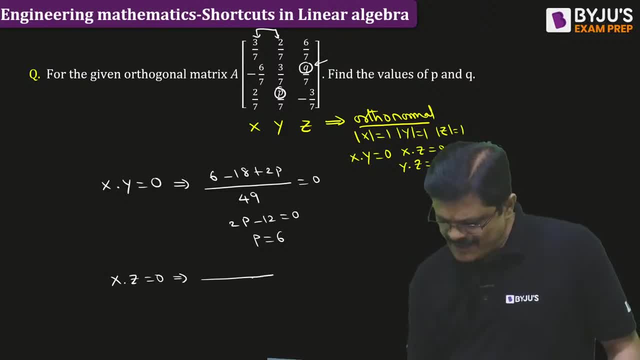 Is equal to 0. So it is denominator 7 into 7, 49.. Numerator 3: 6, 18 minus 6, Q minus 6. Is equal to 0. That means 18 minus 6 is 12,, 6, Q is 12,, Q is 2.. 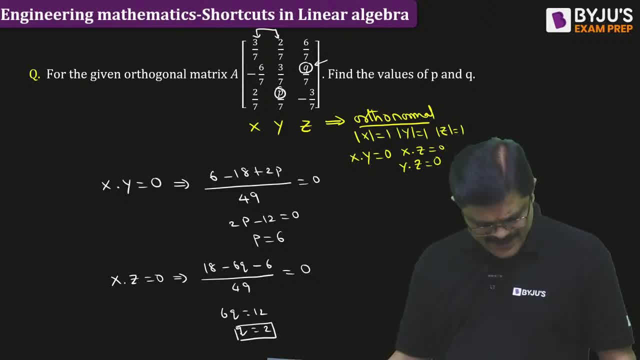 What is this? You people are saying: 6, is it minus 2 or plus 2, sir? Is it minus 2 or plus 2?? 18 minus 6, Q minus 6.. So 6- Q is equal to 12.. 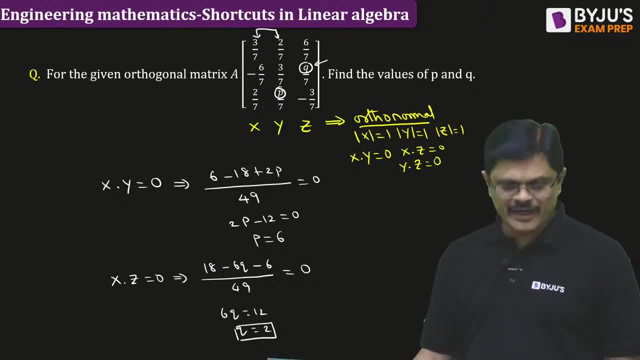 Q is equal to 2.. You people are giving different, different answers. Why? Why you are troubling me, Why you are troubling me, Why you are troubling that answer differently. Very good, Very good, Nice, Nice, Nice, to see that 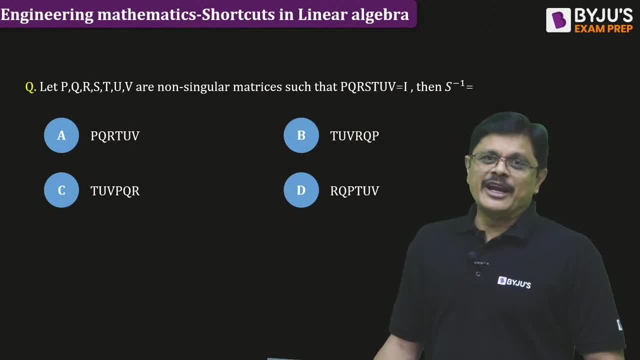 Now comes the very popular shortcut. This is also asked in gate. We are having some non singular matrices whose product is equal to identity matrix And is have. is asking inverse of one of the, inverse of one of the. So for this, if you want inverse for this, whenever you are having product of non singular, 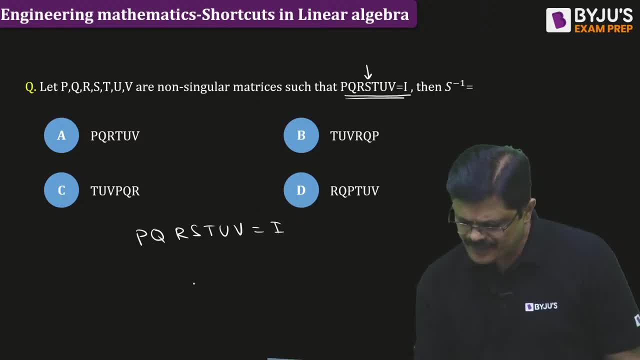 matrices is equal to identity and you want inverse of any one of them. use this circular idea Directly after S, you start: write down these matrices circularly up to here. Write down these matrices circularly up to here. That is T? U. 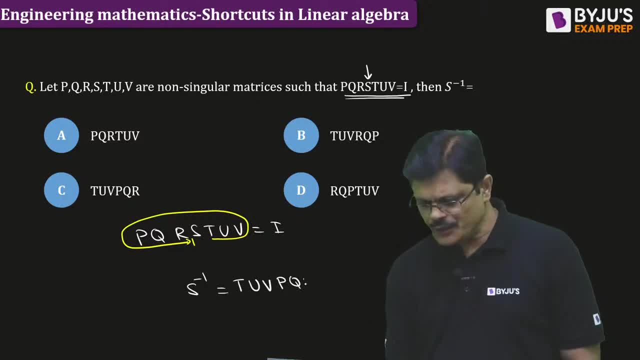 That is T? U. You can apply the linearüreX and you can solve the denominator. If you want to solve the denominator, you do that. But there is a very interesting different formula. I am going to give you this formula, which is called as this formula. 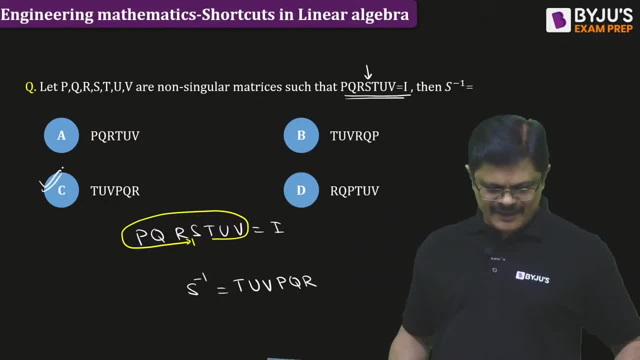 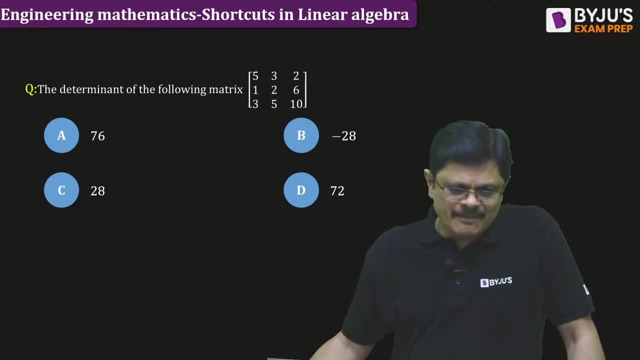 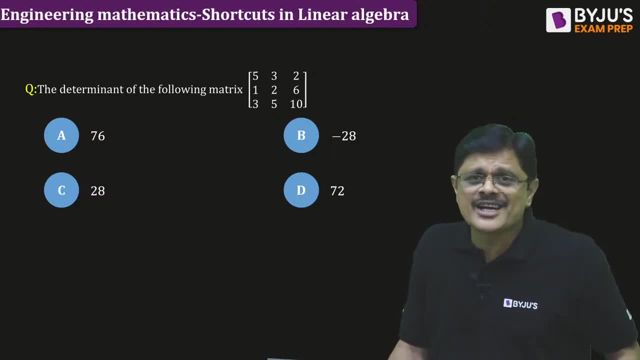 for 4 by 4, 5 by 5, 6 by 6, matrices also. so let me give you that particular idea, sir. remember third type of row operation, your third type of column operation. do not change determinant of the matrix. see, this is called third type of row operation. ri is ri plus k times of rg. see, you do. 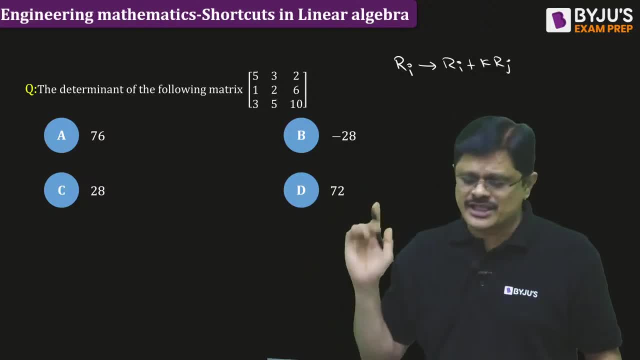 this operation, any number of times determinant, is not going to change. similarly, column operation ci, ci plus k times cj, some constant times of other column or other row, some constant times of other column is added to some other column or this column determinant is not going to change. similarly, 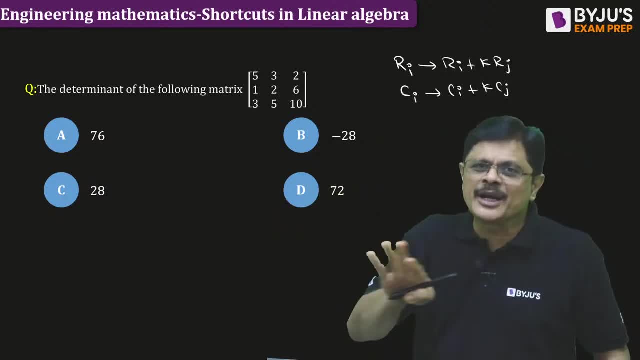 some constant time of other row is added to this row, determinant is not going to change. please remember this. okay, so using that we can make the determinant. determinant is not going to change. so using that we can make the determinant simpler. my dear friends, james bond, please check your answer. babu, okay, please check your answer now. look here all of. 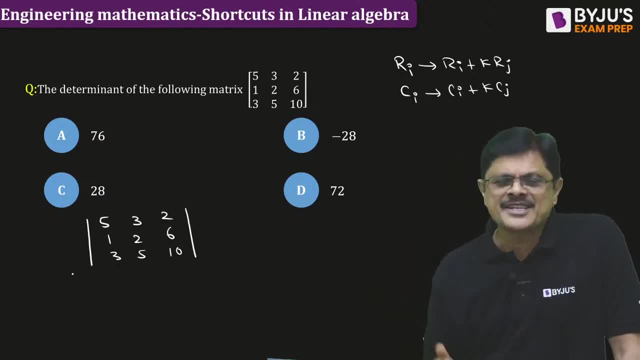 you look here, what i do is, of course, direct expansion can be done along any row, but what i do is i do: r1 is r1 minus 5 times of r2 and r3 is r3 minus 3 times of r2. so right here. what is the determinant of 1? the determinant of 1 is going to change. 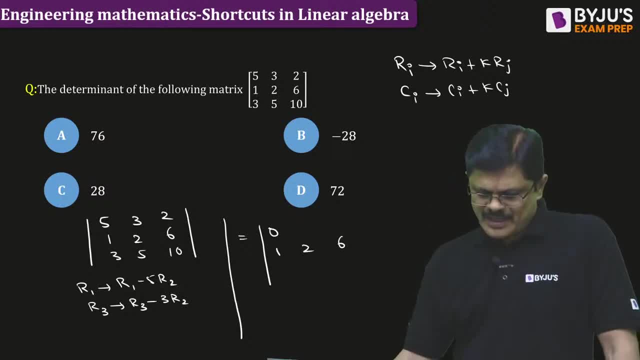 because will be the first row with thecетр a, 2 is going to be the second row of the which get the direction equals to square root of square root of square root of thisettenation, and we are going to calculate the root of square root of 1 with this, the determinate. 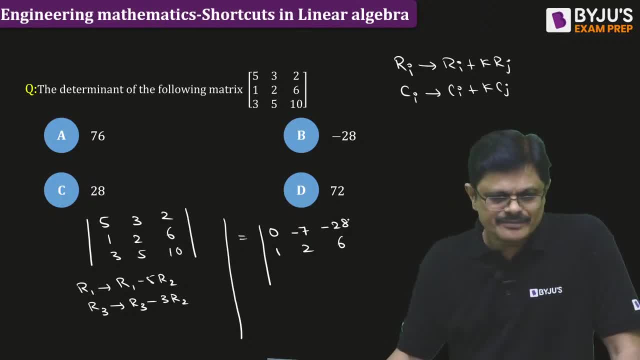 is not going to change. so you get the determinant, which is equal to see. second row remains the same: 5 minus 5 is 0. 3 minus 10 is minus 7. 2 minus 30 to minus 30 is minus 28. ok, then what about the next one? 3 minus 3 is 0. 5 minus 6 is minus 8, murdered at 40 and. 1 is equal to square root of persecutor, and so quantity, you get your total in the last excitation andcade- this is what we are going to calculate of capture. your this the conclusion. always, we're just saying the beginning, and stop before start can be done approximately. 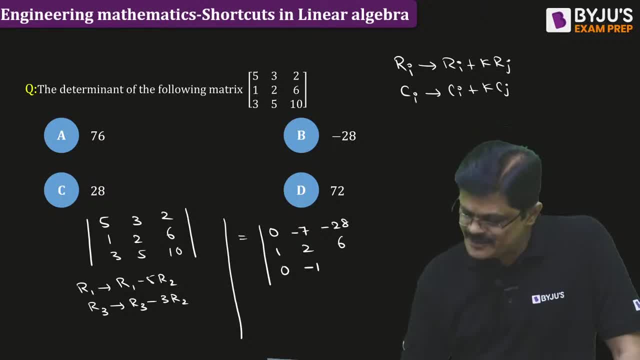 is minus 1. 10 minus 18 is minus 8.. See, my dear friends, you are expanding along the first column to find determinant. So when you expand along the first column, it would be 0 into cofactor. 0 for this element because it is second row, first column, element. minus sign will be there for the 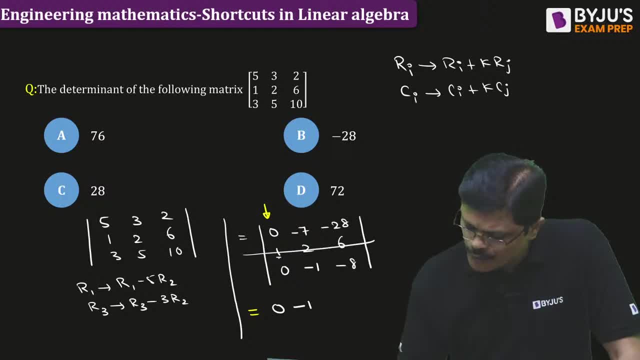 cofactor, So minus 1, into remove the row and remove the column. So what is the remaining determinant? you are going to get This fellow that is minus 7 into minus 8, which is 56 minus 28, and this fellow 0. This fellow is 0. So 0 into cofactor will be 0. So the answer for this would: 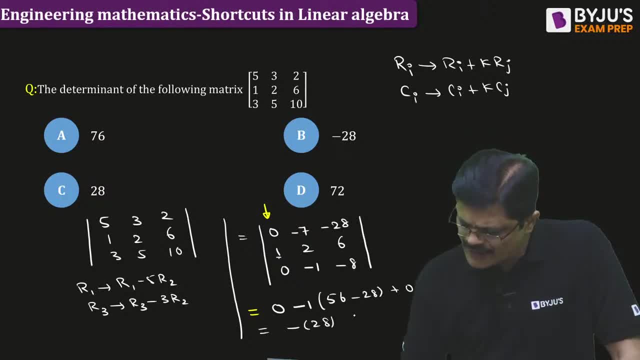 be minus 56. minus 28 is 28.. So the answer for this is minus 28.. I am from Hyderabad. Why it is 28?? Sir, it is minus 28. Babu, It is minus 28, Payas Kumari, It is minus 28.. Okay, 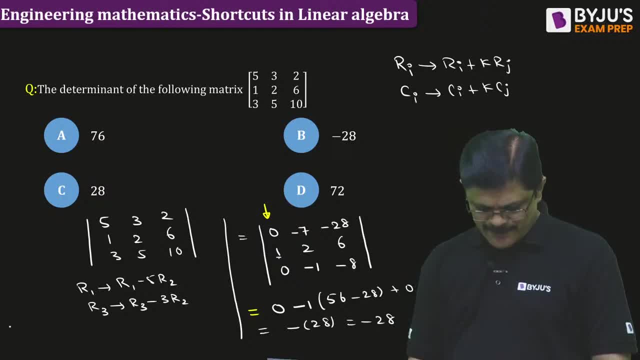 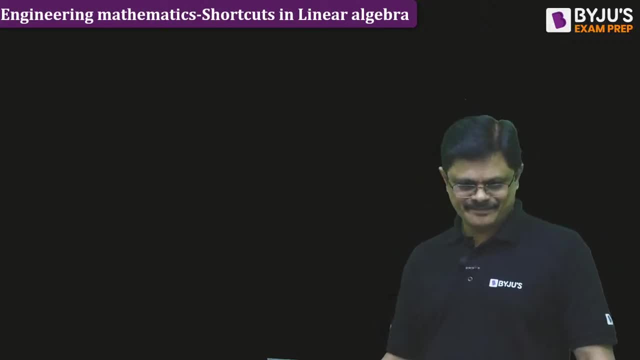 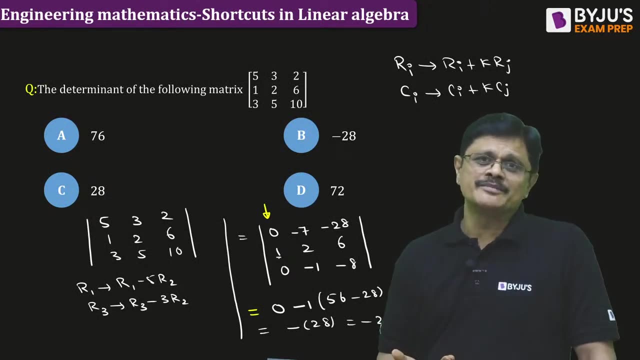 Okay, Welcome to Karnool people. Very good to see new people joining this, Very nice. See, my dear friends. you want, you can expand along this, making these changes, you can solve the problem or you can directly expand and you can get the answer. my dear friends, You can. 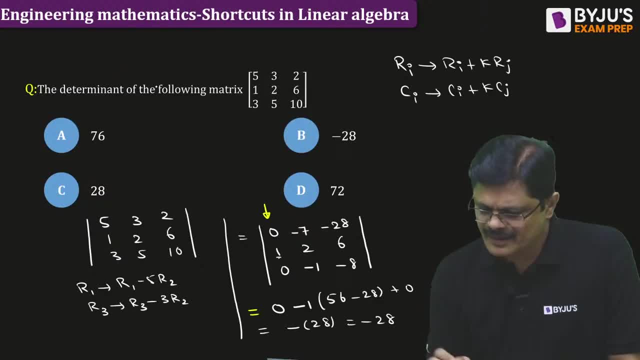 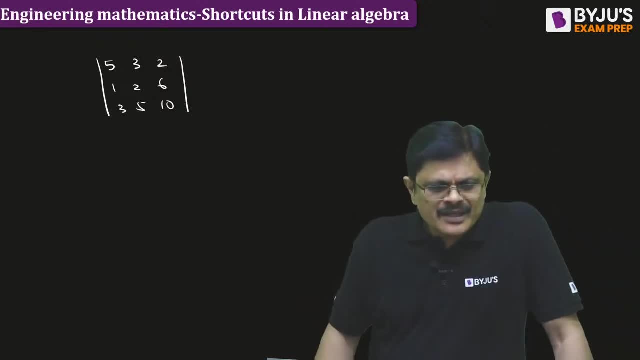 directly expand and you can get the answer: 1, 2, 6, 3, 5, 10.. See: generally, we expand along the row or row or column having more number of zeros. The row or column having more number of zeros. The row or column having more number of zeros. 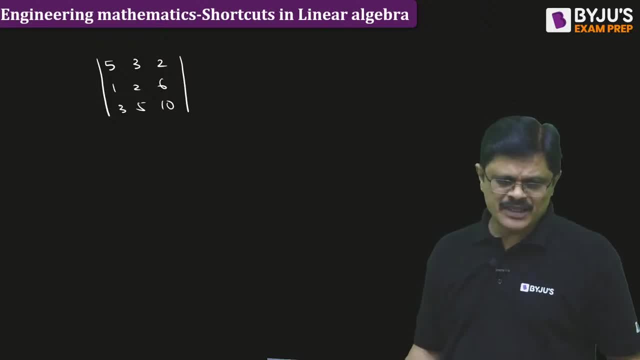 Along that you expand, you'll get the answer faster. Okay, Suppose there are no zeros, Any row or any column is same, So I can expand along the first row. So it would be what, sir? Determinant is what? 5 into 20 minus 30, that is, minus 10.. 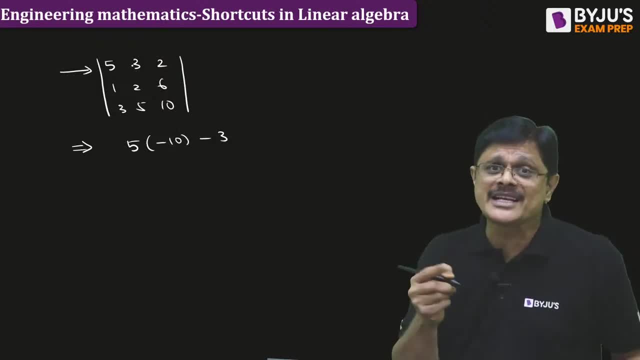 There is a minus 3 here because cofactor will have minus sign. So I am using minus 3 into 10 minus 18, that is minus 8 plus 2, into 5 minus 6, that is minus 1.. So what is it? 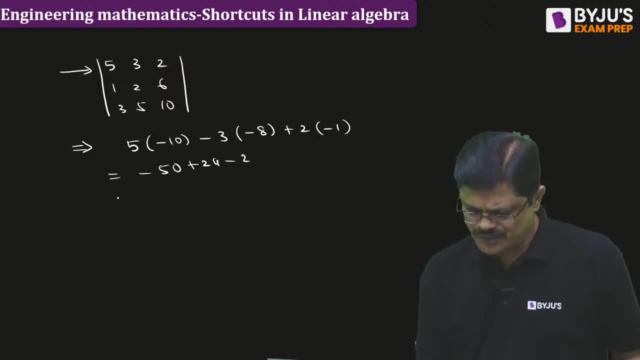 Minus 5.. 50 plus 24, minus 2,, which is correct only now. minus 50 to 24, correct only 28, minus 28,. that is answer. See, it is not lengthy processor, it is actually. problem is most. 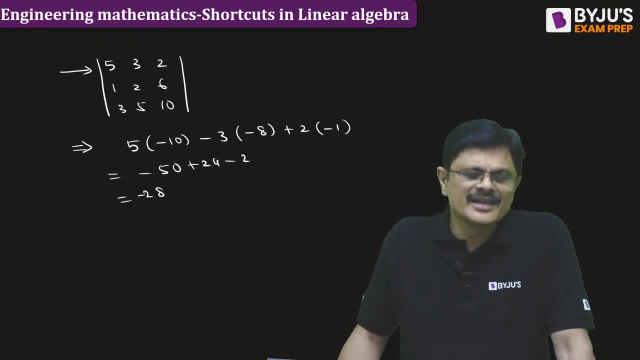 of the people do not know the co-factors. The problem is okay, you do not know the co-factors. that is the problem. but sometimes they ask any question about co-factor. you cannot answer that. Those who know co-factor. they always say this is the best method. 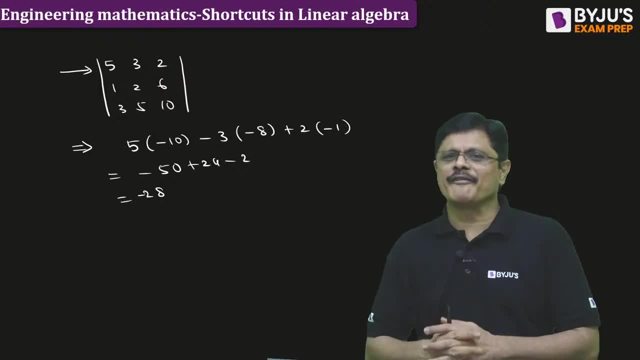 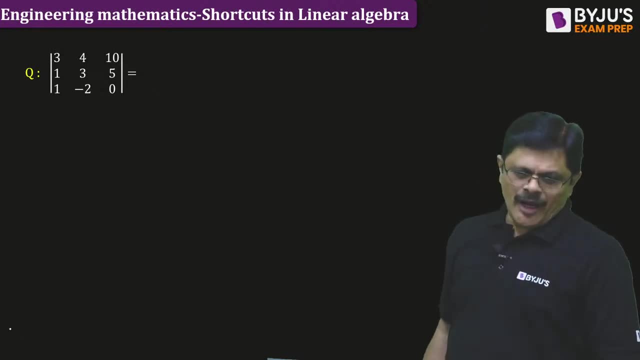 then that you know diagonal method. Okay, fine, you are fine with that method, happy to do it Now. look at this problem. Now I will give you one very interesting story, Babu, I will tell you one very interesting story. See here if you can make some observation. 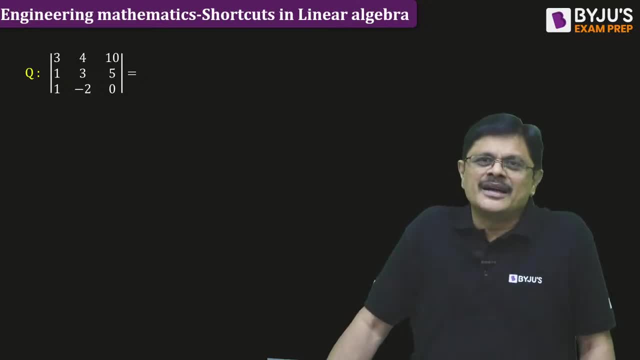 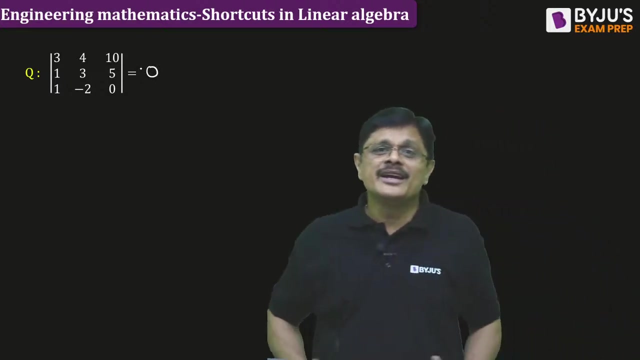 if you can make some observation like relation between rows or columns. if you can find some relation between rows or columns, then determinant will be 0, determinant will be 0, but for that you have to show some relation between rows or 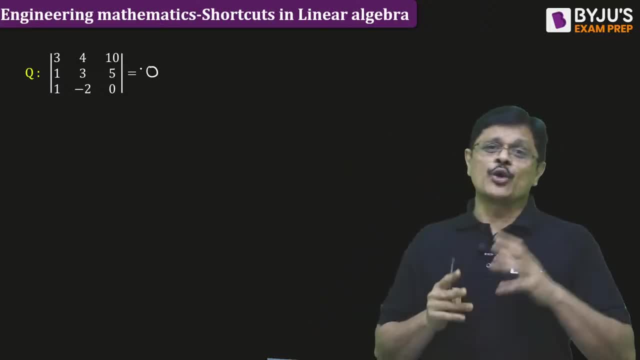 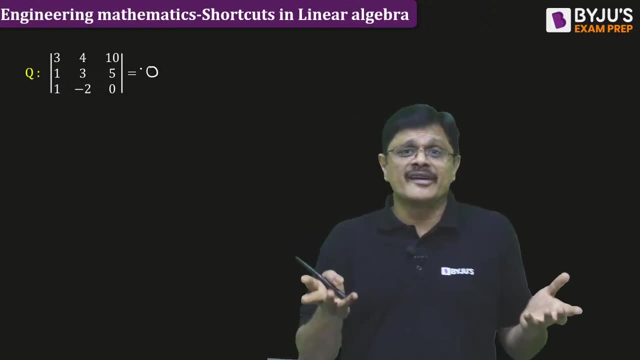 columns. but whenever determinant is 0, the rows are dependent. proportional columns are also proportional, 100%. sure, You just need to find that relationship. my difference Here you see 2 times of row 1 plus row 2 is equal to row 3, correct or not? 2 times? okay, sorry, column. 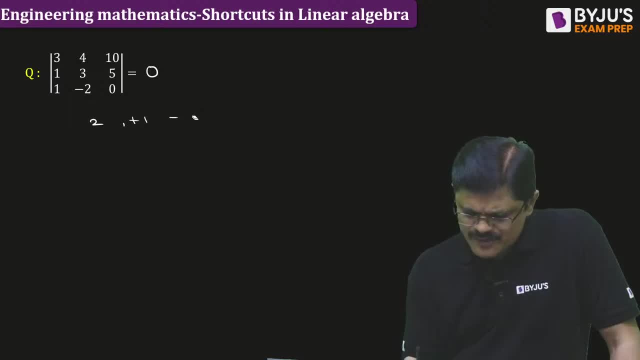 also. okay, rows are different. sorry, let us do it for columns: columns. it is yeah sorry, I am sorry. 2 times of column 1 plus column 2 is equal to column 3.. See not only. 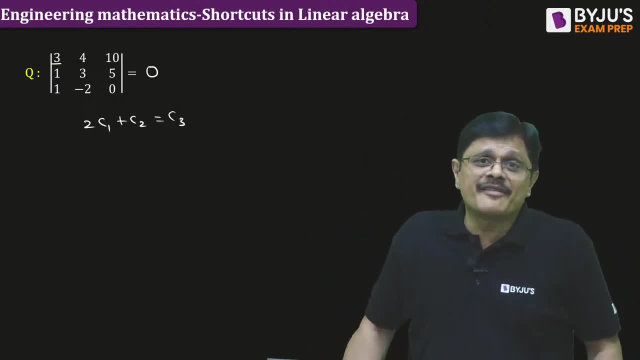 relation between columns. you can also find relation between rows- my difference. you can also find relation between rows here. you can also find relation between columns, rows here, also pulling out heading. yeah, this is also the relation between column 1. 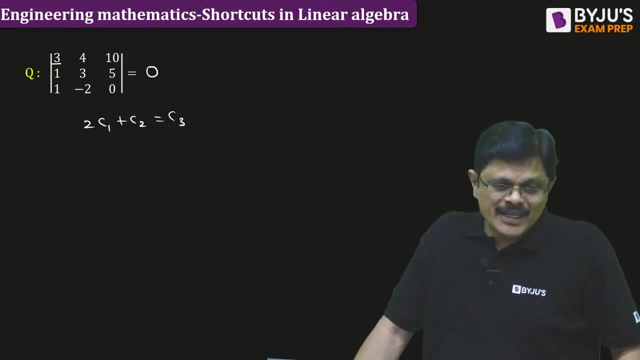 and column 2, okay, and we will see here. okay. last example: row 1 plus column 2 is equal to row 3, right, yes, So let us divide this equationéesris divided. this we can call echelons and eighty. 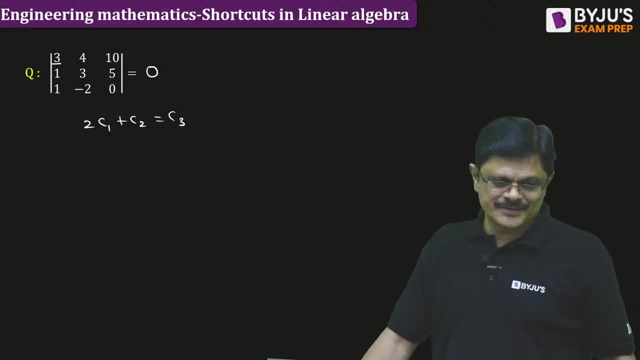 tons. even if, if you can't figure out because row 1 and column 2 are independent companys, we can say: actually I have variety elements here, so that the multiplication variance right, for example, So I can Learning, think, Pray in class I. 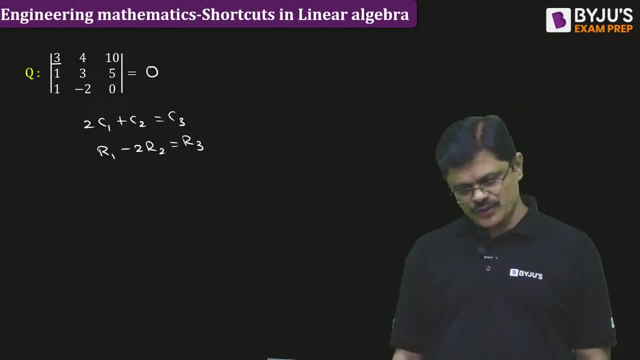 mean I can teach, okay, I've, I've saved, I've stopped. I can have all this Yes空 English 2 times row 2 plus row 3. that also is fine, that also is yeah, that also is fine. see when. 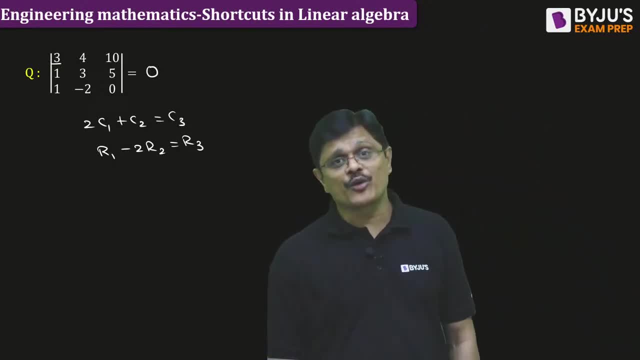 our determinant is 0, there, finitely, there will be some relation between rows as well as columns. definitely there is some relation between rows as well as columns. see, whenever they give you problem, first check whether there is a relation between rows or columns. when our determinant is 0, relation will be there, but sometimes the relation may be something. 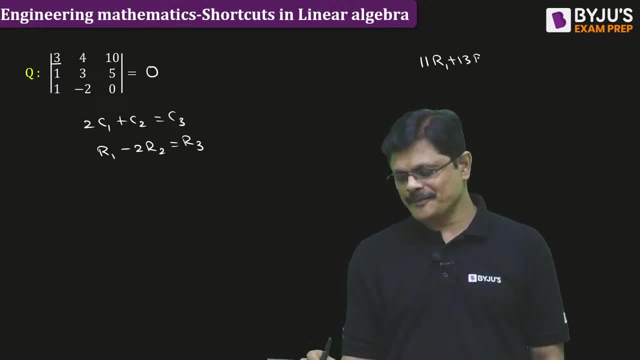 like this: can you find such relations? can you find such relations easily? can you find such relation easily, Babu? can you find such relation easily, Babu? so that is the problem. so you have to be very careful. see relation or observation generally happens within 10 to 26.. 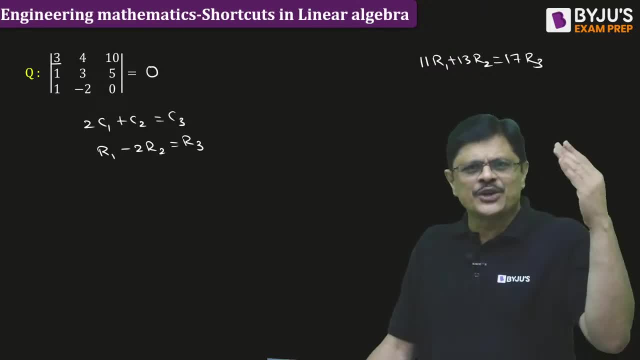 If you don't get that within 10 to 20 seconds, you can use your regular procedure to find determinant by default. yes, yeah, this pdf will be provided. it is a password protected pdf because you asked the pdf, this will be provided with a password, and the password I'll share. 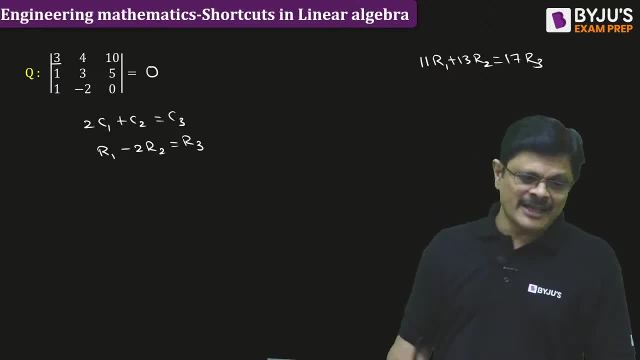 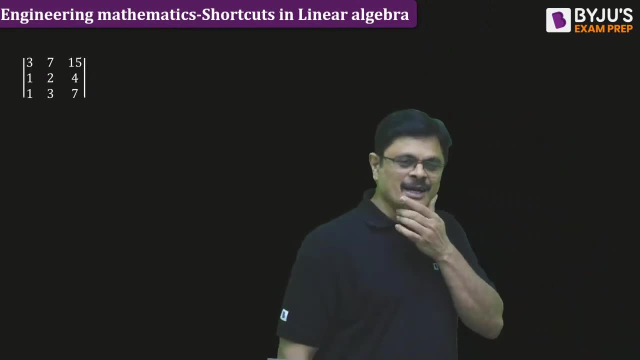 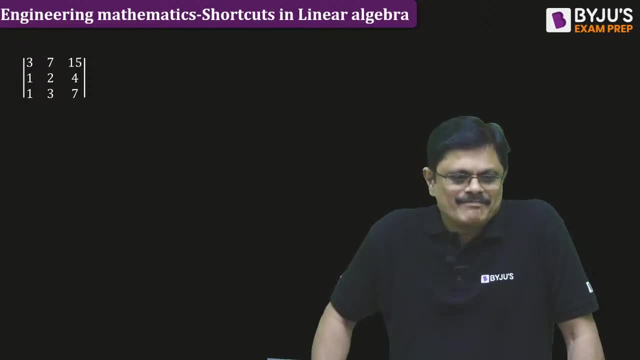 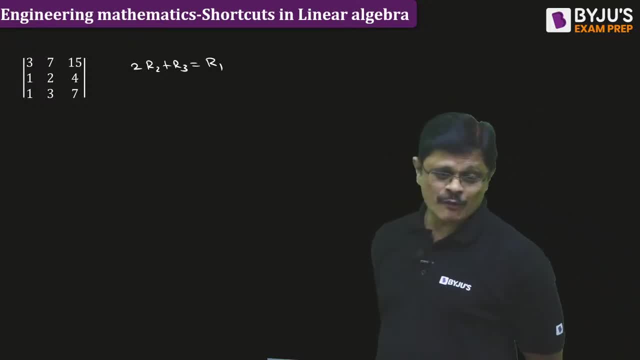 hmmmmm, hmmmmmm, hmmm, hmmmmm, hmmm, hmmmmmm, it's something. hmmmmmmmmm, hmmm, hmmmmmmmph, cmmmmmmmmmmmmmmmm, times of C1 plus C1.. You can't do such kind of thing, sir. You can't just add 1s That. 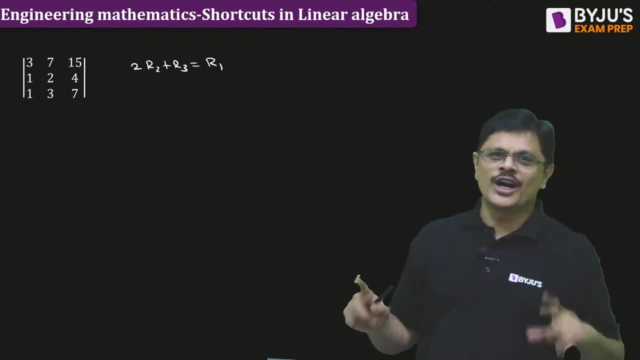 cannot be done. That is not allowed. money That is not allowed. Wrong, That is not allowed. I given a hint: Continue. Complete this 3 times of column 2.. I given a hint: Complete that now. Complete that relation 2 times of column 1.. 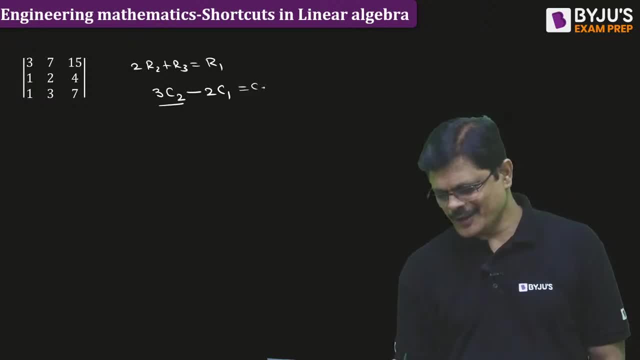 Is equal to column. See whenever you can able to find such a relation between. this is called dependency relationship. If the rows are dependent, proportional columns are dependent. yeah, proportional determinant will be 0.. Okay, Nice, Now there are some. 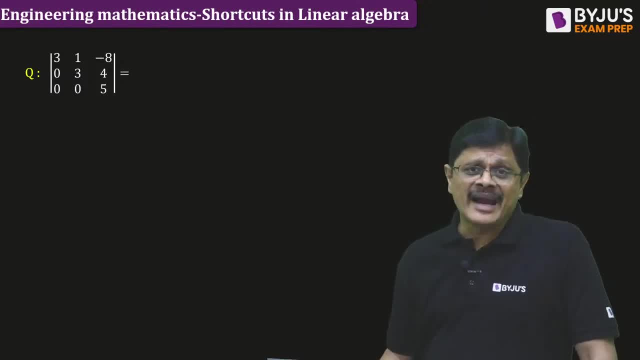 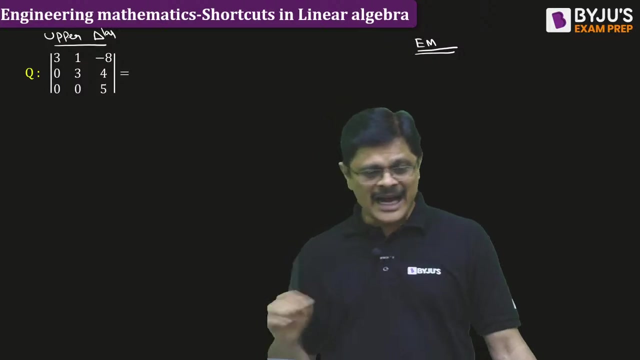 more interesting things. like you know, This is called upper triangular matrix. What is determinant for upper triangular matrix? What is determinant for upper triangular matrix E m? the answer for this this is the password for pdf E m and answer for this result is password for your pdf E m and. 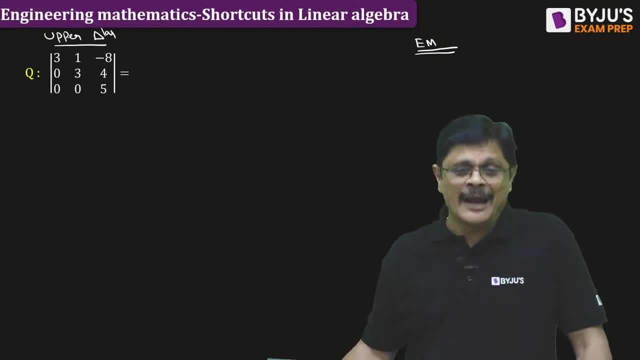 password for this is answer for your pdf. I am not giving answer. Answer is: product of main diagonal elements. Don't write in pranab. Remove that from there. Ha E m and answer for this E m, followed by answer, is the password for this pdf, my dear friends. Okay, The pdf will be available. 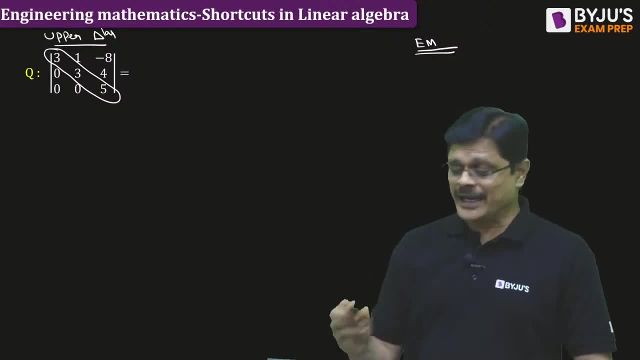 in my telegram group. Okay, That is cs underscore, sridhar. It is available only in this telegram. It is available only in my telegram group. Babu, Am I clear? You have to join my telegram group. See, so much problems, So many problems, Right, Nice, Nice, Next one. What is determinant? 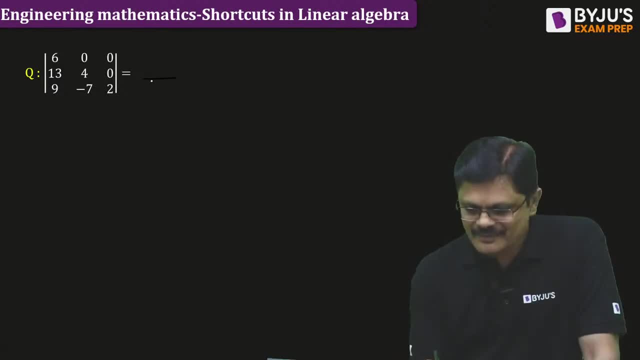 of this. See, it is called lower triangular matrix. See, whether it is upper triangular or lower triangular matrix. Determinant is product of main diagonal elements, That is, 6 into 4x3.. Okay, Now, this is the determinant for the lower triangular matrix. This is the 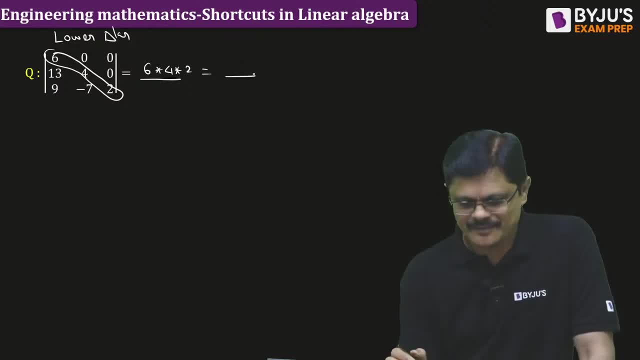 4 into 2.. What is it? 48. Very good MK Entertainment. Very good James Bond. Nice, nice. Ashok Payash, Shashi, Pranap Paul, Very, very good. my dear friends, You are doing great. What is this? This is called diagonal matrix. 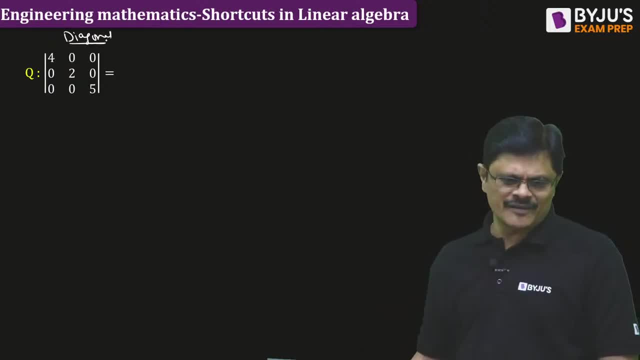 This is called diagonal matrix. What is determinant of this? What is, Oh, next one. you answered Very good Pranap. You are rocking my dear friends. What is determinant of this? Even if it is diagonal, product of main diagonal elements is determinant 4, 2,, 8,, 8,, 5,, 40. 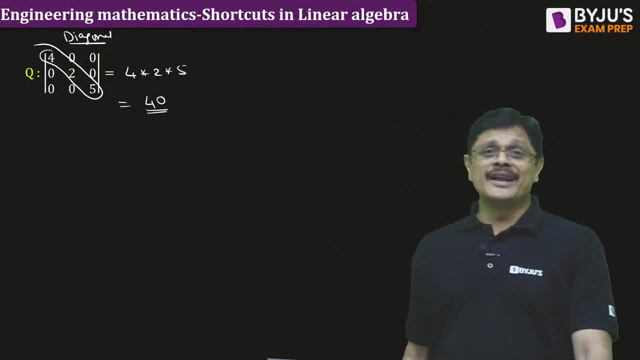 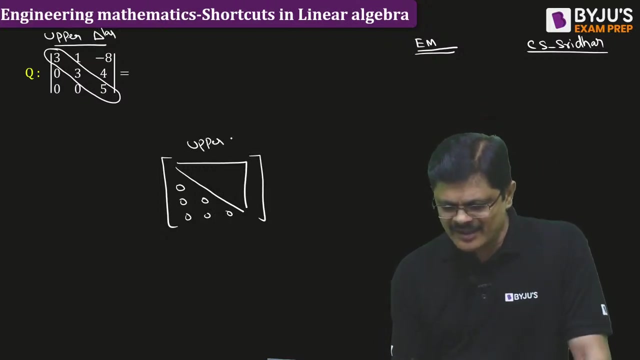 Now let us move to the next shortcut. See: upper triangular means you find elements only above the main diagonal. Below that you find all zeros. That is upper triangular. This is upper triangular. So we can say: A, I, J is equal to zero, for all, I greater than J. 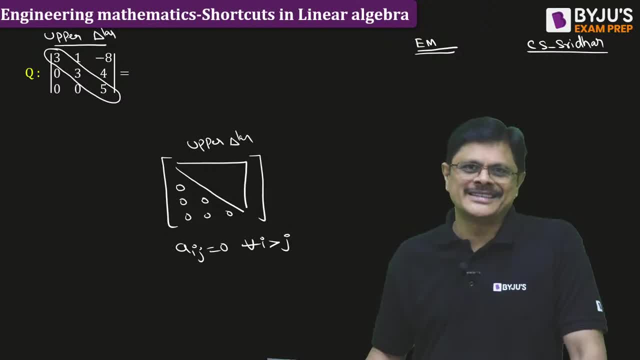 Isha Ray Chowdhury. you understand, That is how we find it. Is the idea clear? Now, lower triangular means: here we have elements. See, actually, the condition is these fellows must be all zero, These all must be zero. That is the condition. 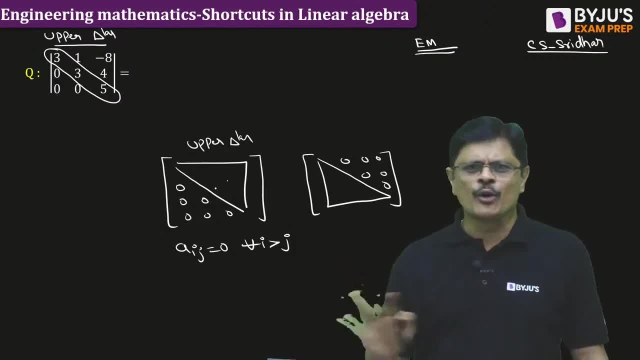 Here you may have some zero, some non-zero, Anything, no problem. But this is the condition Here: A, I, J is equal to zero for all I less than J See. actually, if you see it is 2, 1.. I greater than J, then it is zero. 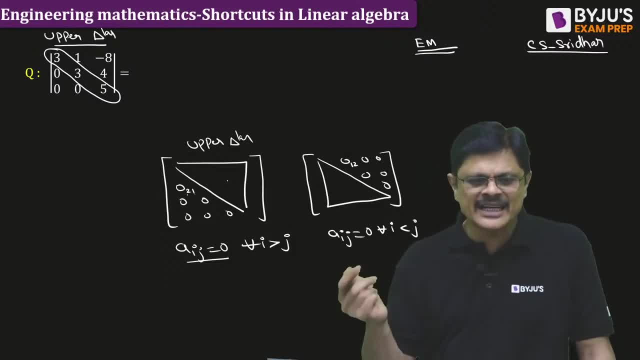 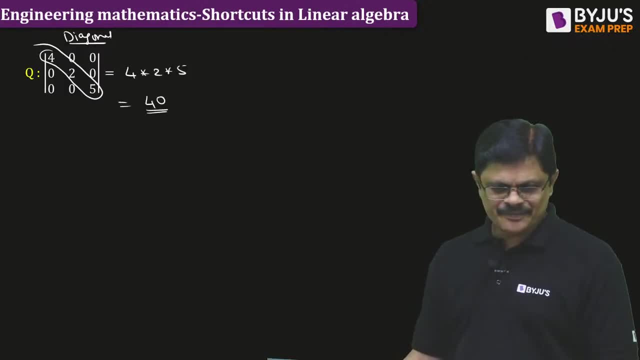 Here it is. you see, it is 1,, 2.. i less than j, then it is 0.. Like that. So what is the answer? Okay, Ganapati Mahi, you just started. I think you answered this question 45.. 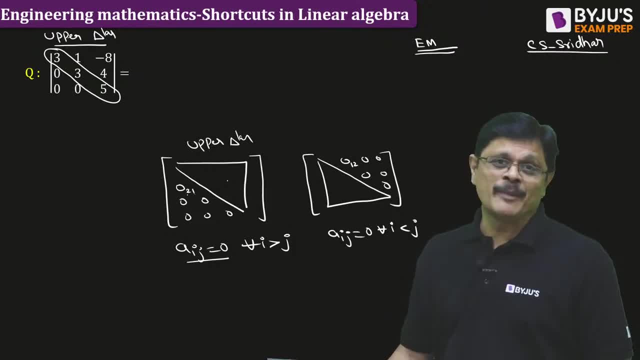 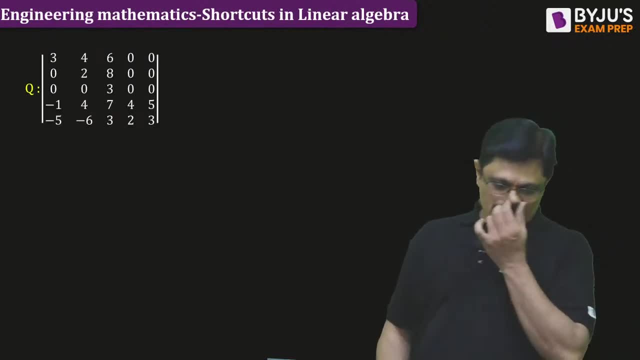 Very good. There was one more secret. The password for this PDF is given little earlier, Nice. Now let us see this particular one. It is neither upper triangular neither lower triangular. What is this? Something new? See, I will give you one very interesting trick. 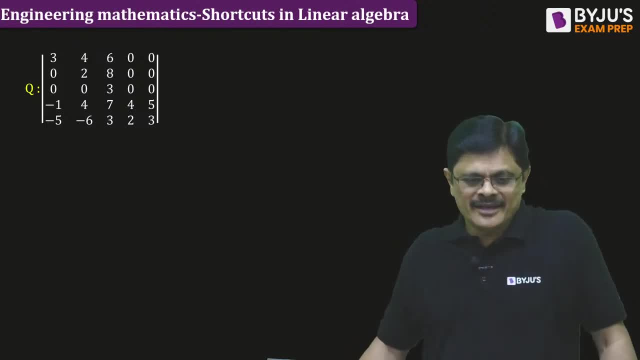 Please remember it is called block diagonal matrix technique. It is called block diagonal matrix technique to find determine my difference. See generally. if it is not in that format, you can use row operations or the column operation to reduce to that particular format. 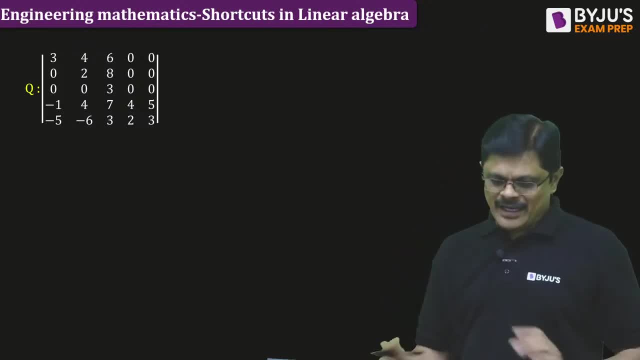 My friends See, generally, if it is not in that format, you can use row operations or the column operation to reduce to that particular format. My friends, Right sir, Now what we do for this particular technique is we need to get this particular format of matrix. 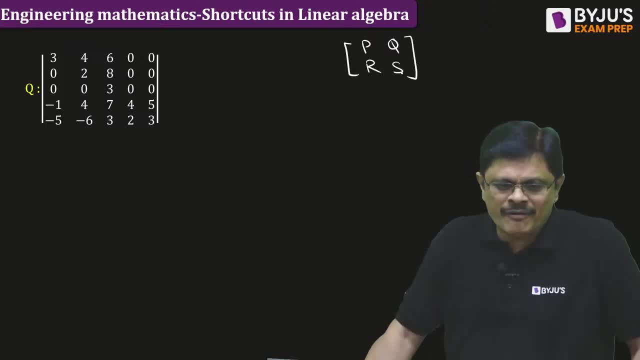 My friends, We have to get this particular format of very good Pranapol, Pranapol, don't reveal secrets before I teach, Okay, Otherwise they feel that I am copying from you Right, Clear Now what is this? 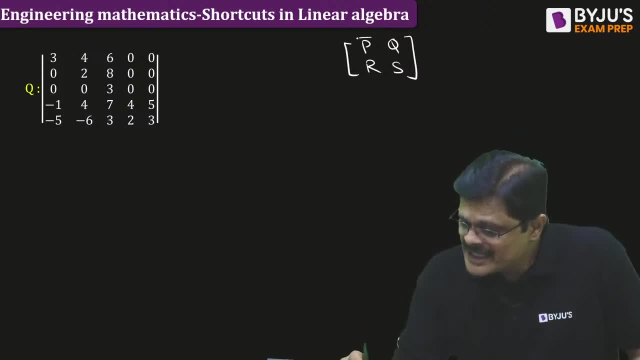 This is PQRS. In this we have to make this P square matrix, S square matrix. How to make P and S square matrix. sir, You can divide this here, Or see, if you divide it here, what happens. 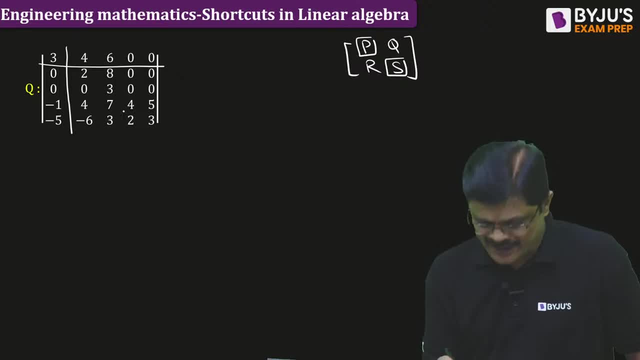 P is 1 by 1 matrix, This S is 4 by 4 matrix. Or if you divide here, If you divide here, P is 2 by 2 and S is 3 by 3 matrix. my friends, 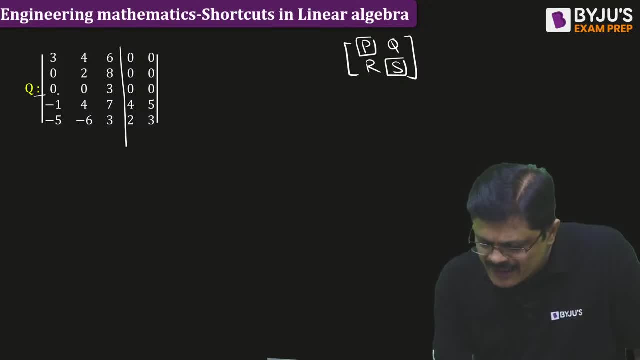 Or if you divide here, P is 3 by 3, S is 2 by 2. So you can only make these divisions, my friends. That is P 1 by 1, S 4 by 4.. 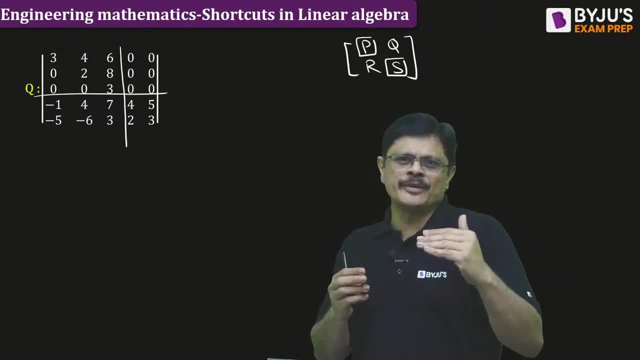 P 2 by 2, S 3 by 3.. P 3 by 3, S 2 by 2.. P 4 by 4, S 3 by 3.. S 1 by 1.. These are the divisions possible. 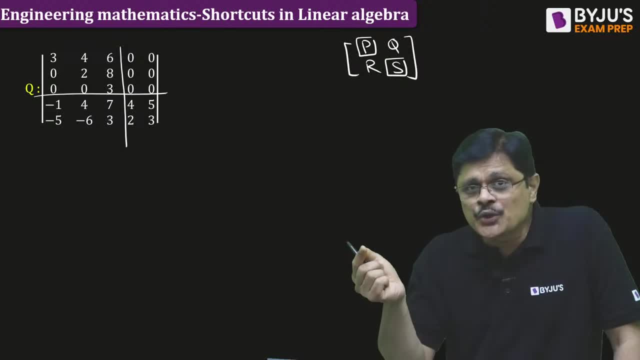 And after that, either Q or R or both must be equal to 0. Either Q is 0, or either R is 0, or both Q and R equal to 0,. my friends, If it is Q 0, then we call it as lower triangular block. 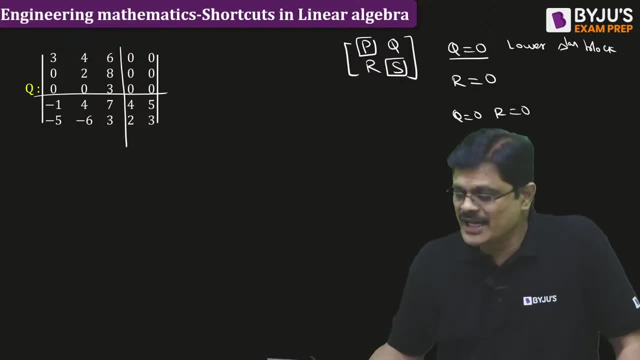 What is it called Lower triangular block matrix If R is 0.. If R is 0,, then we call it as upper triangular block matrix, And if both Q and R is 0, then we call it as diagonal block. 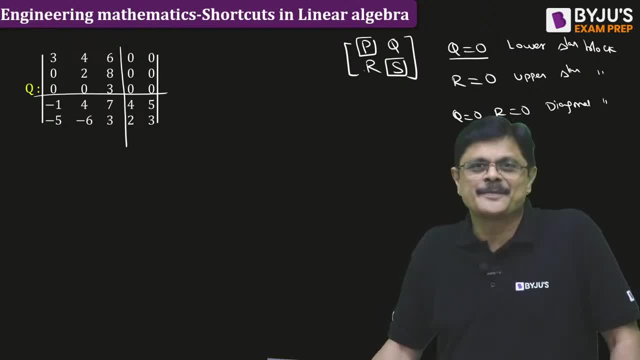 What is it called Diagonal block matrix, my friends? And in this particular situation, if it happens, then determinant of this is simply given by determinant of P into determinant of S. You can find determinant just by finding determinant of P and determinant of S. 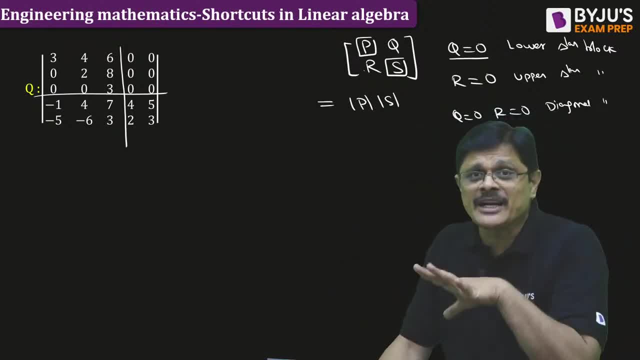 But that division is very, very important And while doing that particular division, Either Q or R or both must be equal to 0. Till that you have to continue this particular division. And this is the division which actually gives me the block. diagonal form, lower triangular block. 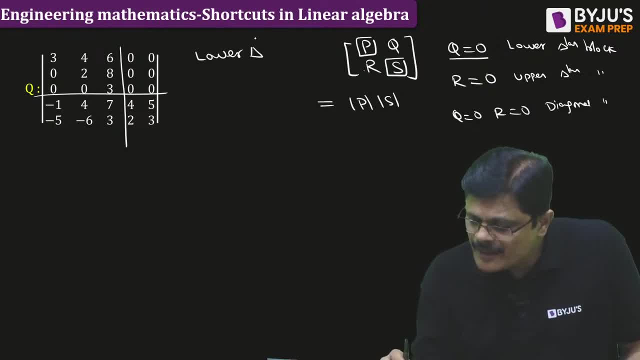 What is it? This is a lower triangular block. So once it is lower triangular block, what happens, sir? The determinant of this matrix, The determinant of this matrix is simply Determinant, Determinant of this upper triangular, that is, P part. 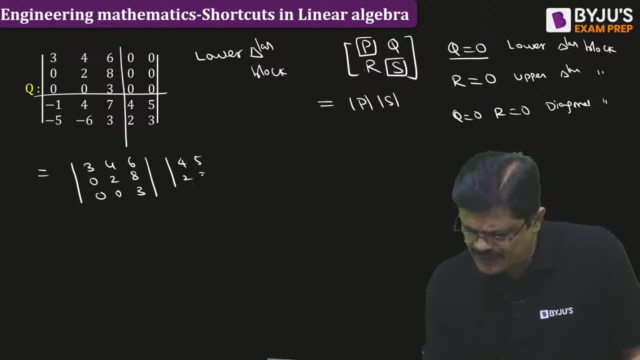 And determinant of this small fellow that is 4, 5,, 2, 3.. So find determinant of this and determinant of this, you will get the required answer. You will get the required answer. Very good. So because here it is upper triangular matrix, determinant of this is direct. 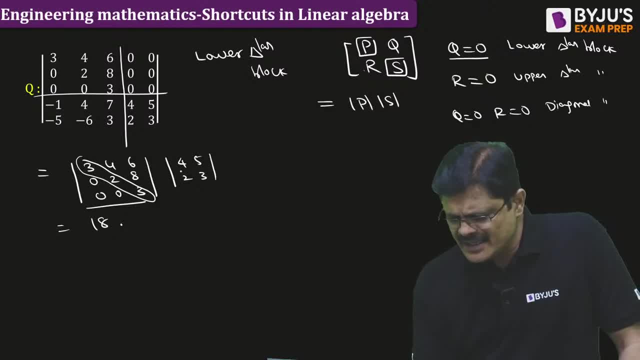 3, 2, 6, 6, 3 is 18.. And this is 4, 3 is 12 minus 10 is 2.. So the answer for this problem is 36 matrix. So answer for this problem is 36,. my dear friends, 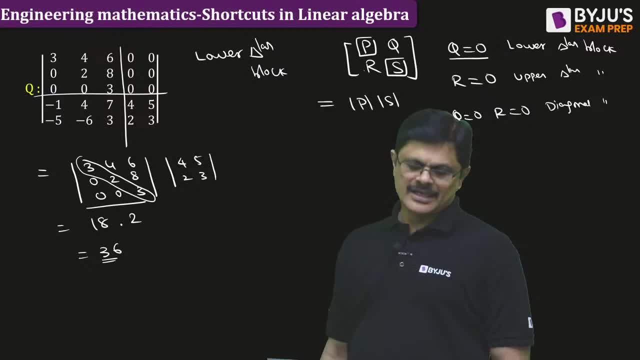 Yes, sir, 36 is the answer. Super, You can also try different versions. sir, Whenever you are having this big matrices, try to convert them into upper triangular block or lower triangular block or diagonal block. my dear friends, It will help you in solving determinant fast. 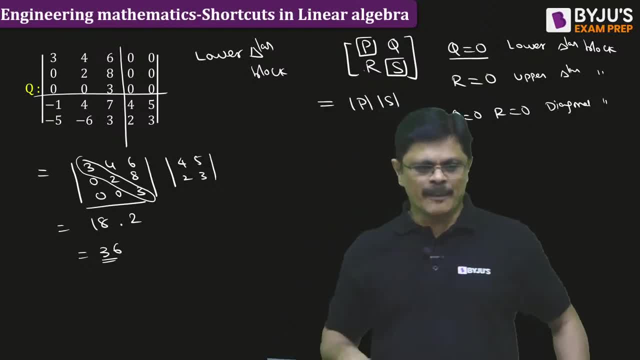 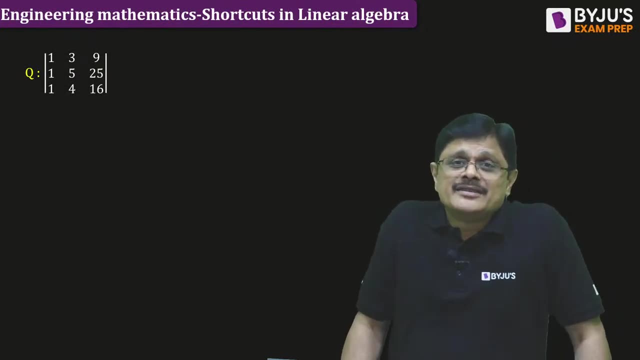 That is the trick. yeah, shortcut for big matrices. Generally people ask me, sir, If they give big matrix, you have to do that. Am I clear? Now there is a wonderful technique which is given by Vandermans. 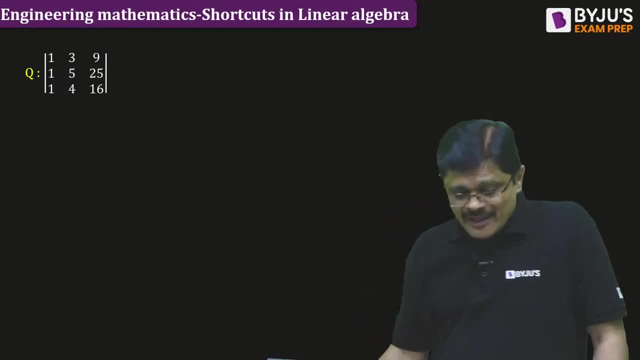 It is called Vandermans determinant. What is it called Vandermans determinant? See, actually, if you see your 10 plus 1, I mean 10 plus 1,, 10 plus 2, you will find many more forms, my dear friend. 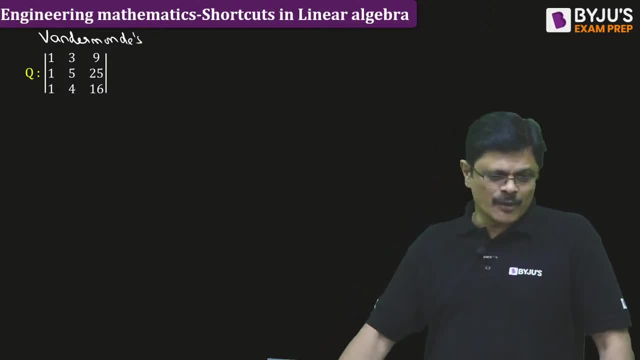 But this is 1.. This is 1 of the important form. my dear friends, This is 1 of the important form. See, the idea here is for Vandermans form. this would be the form, sir. Here we have 1,, 1,, 1.. 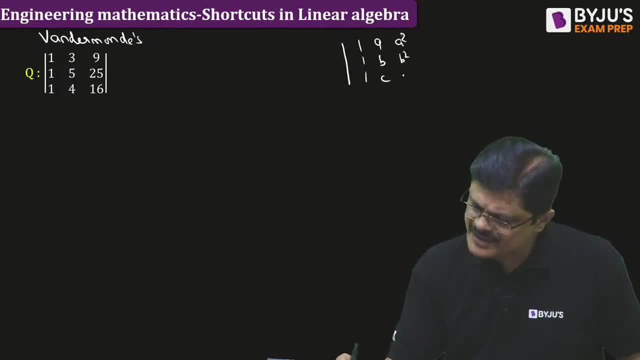 Some a, b, c will be here The square of. that would be here, my dear friends. Or the 4 by 4 form is 1, 1, 1, 1, a, b, c, d. here the squares, here the cubes. here, my dear friends. 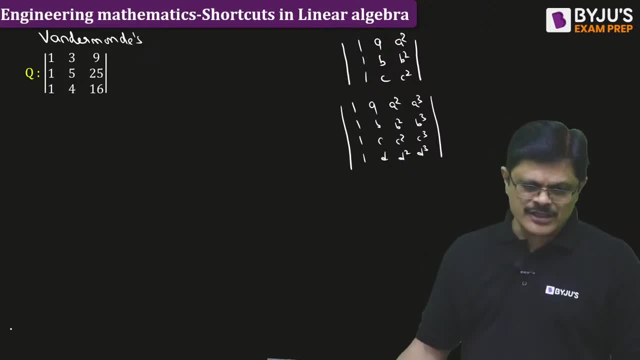 In any case, you can find determinant, of course, by direct method also. some people are doing like Shashie, Shashie or Shashie. What we need to do is you fix a, do just b minus a and c minus a. 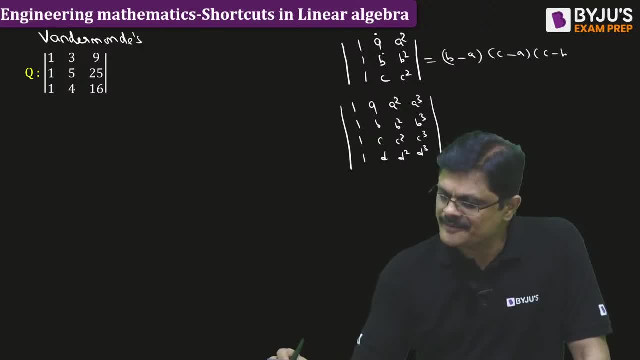 Done. Now fix b. do c minus b. Here also you can do the same thing. Fix a. subtract a from all other fellows, like b minus a, c minus a, d minus a. Then what do you do? 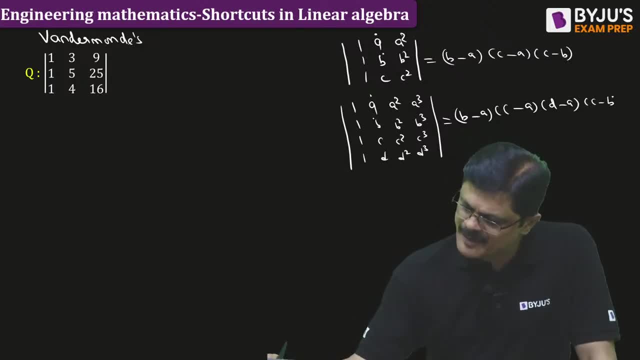 You do fix b. subtract all other fellows, that is c minus b. Am I clear? c minus b? d minus b. Am I covering it? Am I covering it? No right, Like this: d minus b. Now fix what. 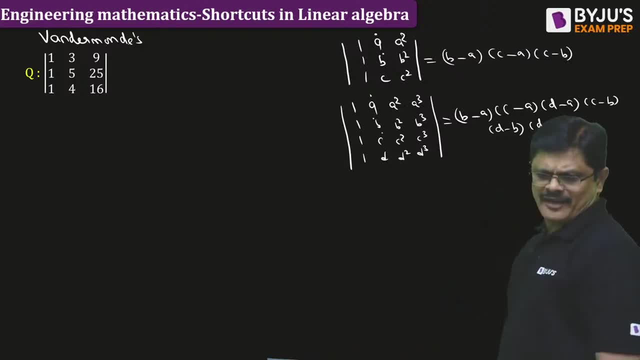 c, Then do d minus c. So this is a shortcut, very, very wonderful technique. This can be generalized to 3 by 3,, 4 by 4,, 5 by 5,, 6 by 6,, 100 by 100,, 1000 by 1000 also. 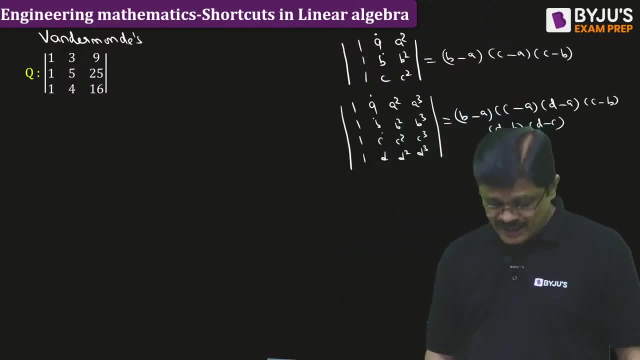 That is a beautiful form. here I didn't. That is the beauty here identified by difference. Am I clear? So that is a beautiful technique. by difference, That is a beautiful technique, So here you can simply do it. What is it? 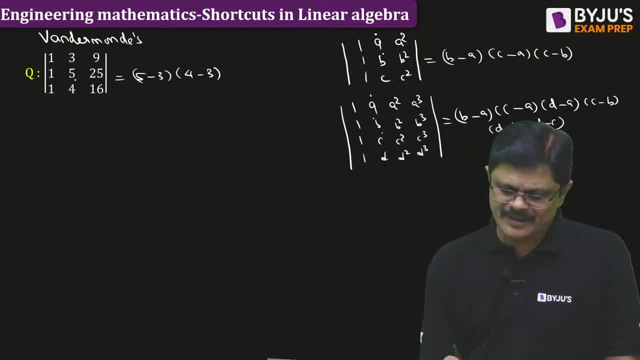 5 minus 3,, 4 minus 3,, then 4 minus 5.. And that is the answer for this problem by difference. Please do the simplifications and get the answer Right. So what is the answer, sir? 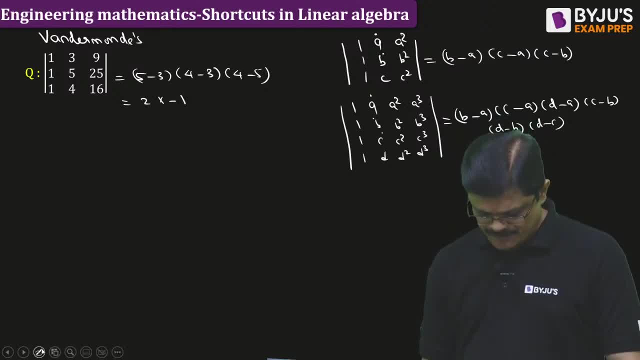 2 into minus, sorry, 1 into Minus 1, which is minus 2.. Very good, Try this as homework, my dear friend. Try this as homework, my dear friends, All of you, try this as homework. 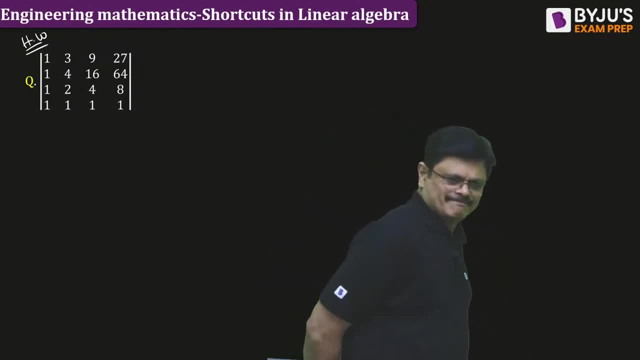 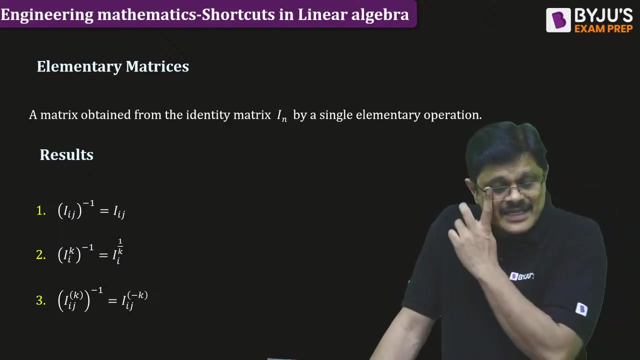 Please try this problem as homework problem. The next one: See, there are something called elementary matrices. See, these are the matrices which are obtained. These are the matrices which are obtained by doing single row operation or single column operation on identity matrix. 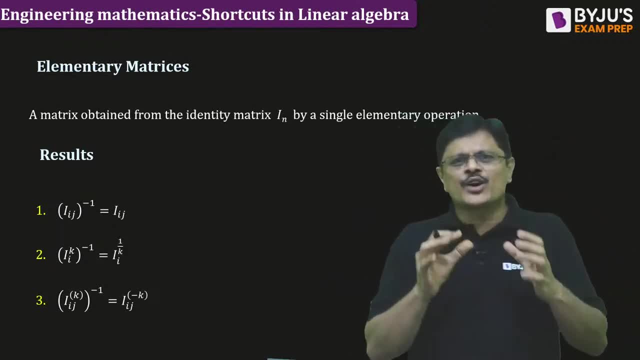 That is on identity matrix. if you do single row operation, yeah, single column operation, then you get this value. Such matrix is called elementary matrix, And if you know it is elementary matrix, I can find its inverse within No time. I can find its inverse within no time. 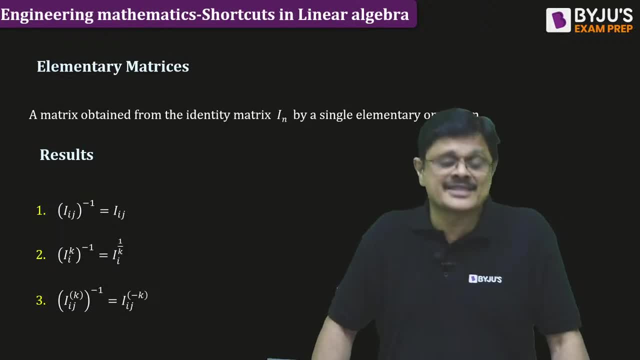 My difference: there were three to four questions asked in gate based on this directly inverse. You don't have to do adjoint by date, sir. My difference: you don't have to do this adjoint by date formula Directly. you'll get the answer for the inverse. 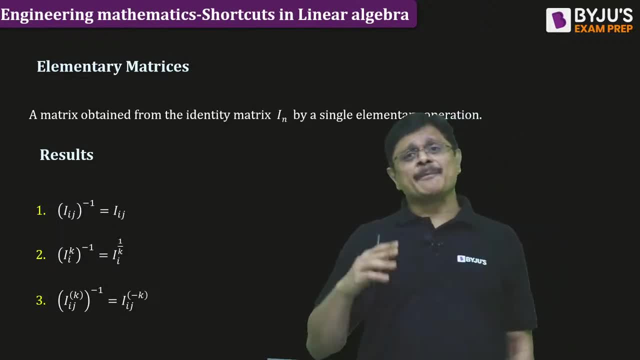 My difference. OK, so a matrix is which is obtained from identity matrix by using a single row operation. Single row operation means interchanging of two rows Right, Or multiplying a row with a non-zero constant or adding a constant multiple of other row. 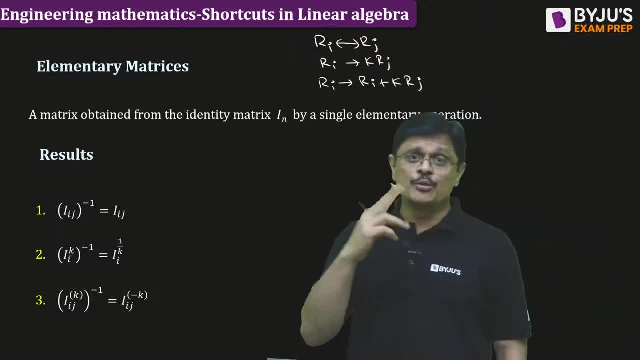 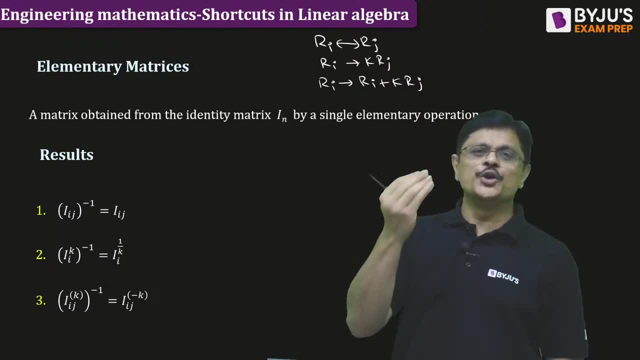 Any one, any one. only, You can't do more than two, OK, more than one. You can't do two or more, You have to do exactly one row operation. The new matrix which is obtained from identity matrix is what is known as elementary matrix matrix. 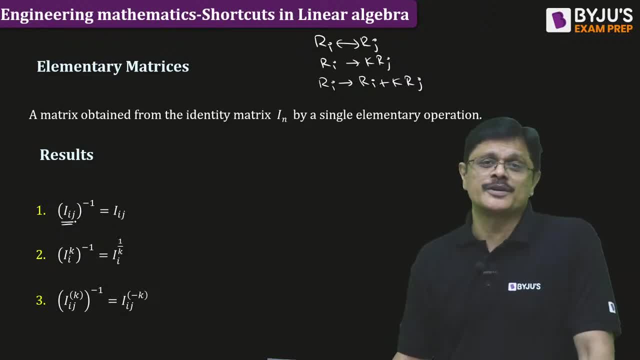 Now, if it is obtained by interchanging of two rows, The inverse is exactly same as the given matrix. It is obtained by multiplying a row with a non-zero constant. Wherever that k is there, you just write one by k there. 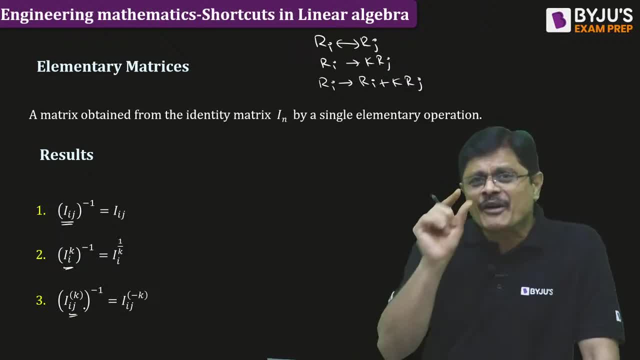 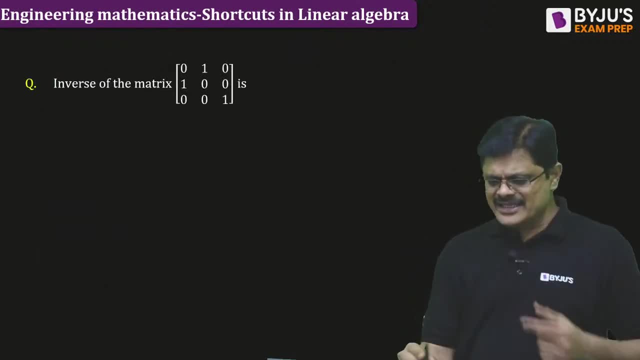 It is obtained by third row operation. Wherever you find that k, you just make it as minus k. You will get the answer. So if you apply that, I can tell that. suppose this is the matrix A. For this matrix I say: inverse is same as A. 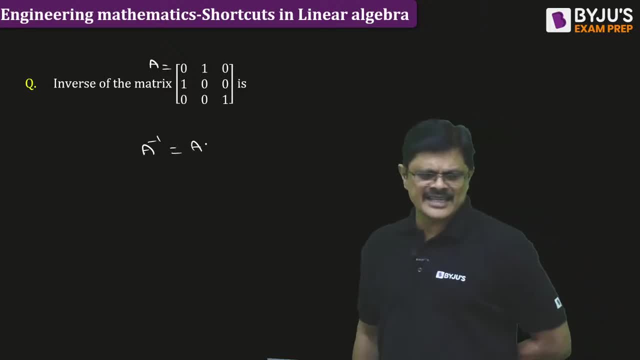 For this matrix, I say: inverse is same as A, same as a. for this matrix, I say: inverse is same as a. why? because this is obtained from, this is obtained from my identity matrix by doing slapping of first and second rows. by doing slapping of first and second rows, I got this. therefore, inverse of this matrix is directly. 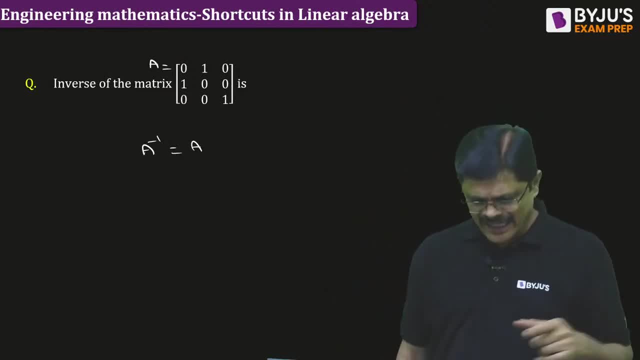 here I do not do any adjoint, I do not do any determinant directly. I know the answer: a you want, you can verify. if it is obtained by swapping of two rows, then it is what I, elementary matrix, and for this elementary matrix, inverse is directly itself. that is the first rule. 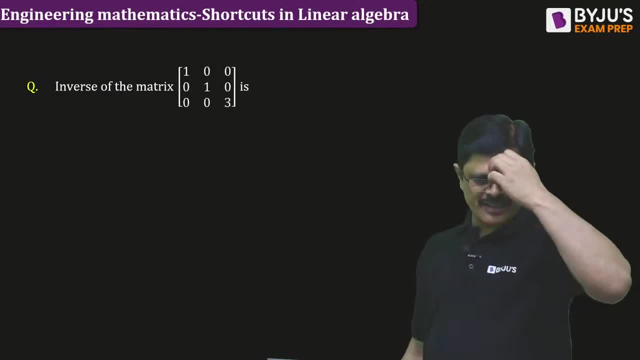 now look at the second one, sir. now look at the second one, my defense. hello sir, good morning. what is inverse of this matrix? what is inverse of this matrix actually? here we can also consider this as diagonal matrix. for diagonal matrix inverse is main diagonal elements. you revert or you, what you call, reciprocate the main diagonal elements. 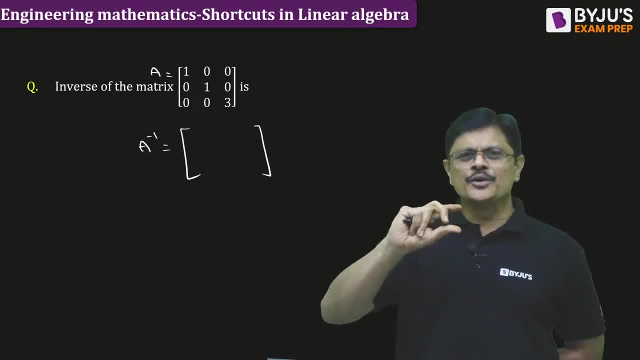 you are going to get their that idea. you can use. so here, one by one, by three, you can do it and you can get the answer for this matrix. you can get the answer for this matrix. what is inverse of this matrix? this my difference. Yes, yes, Wherever 3 is there, you have to replace 3 with 1 by 3.. 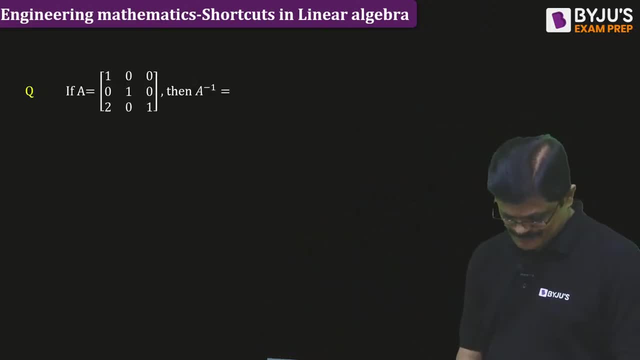 That is it. One more interesting fellow. One more interesting fellow. What is inverse of this? See, for this they ask this question directly in gate. I write the answer just like this: 1, shown you, shown you, Shown you. 1, shown you Where 2 is there. I just 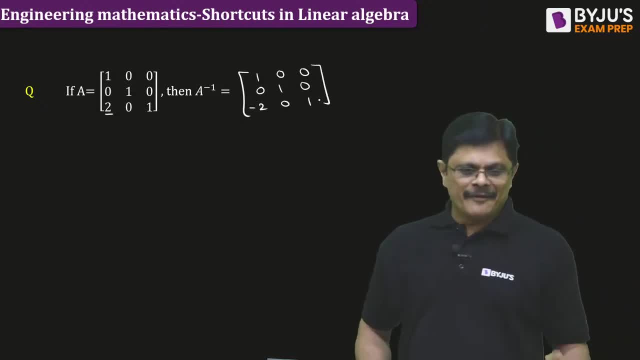 put minus 2, 0, 1.. Within 1,, not even 1 minute, sir, Within 1 step, you can get the answer Just by observation. you can get the answer for this Just by observation. What is the? 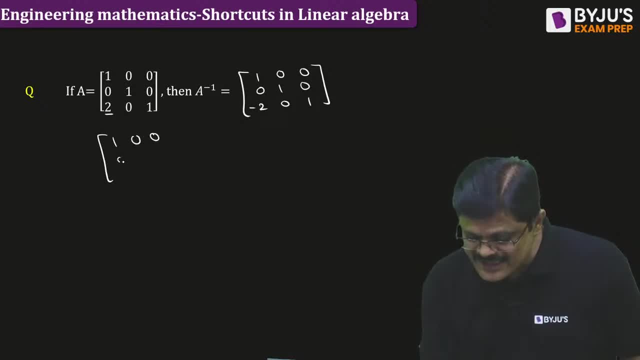 observation needed. This matrix is obtained from identity matrix. On that I do that. rho 3 is rho 3 plus 2 times of rho 1.. Then I get this matrix A, Then I get this matrix A. If you can able to do this observation, you get the answer. 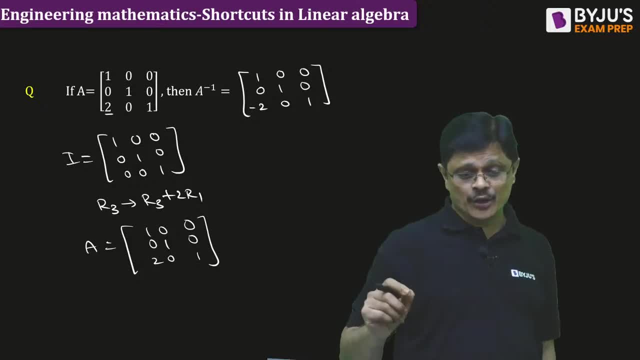 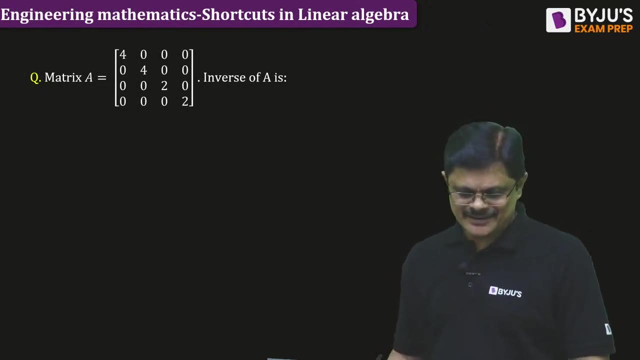 Your answer is ready. Your answer is ready within no time, my dear friends, Within no time, my dear friends, Hope you understand. Is the idea clear, Wonderful? Now, this is a general result. What is inverse of this matrix? 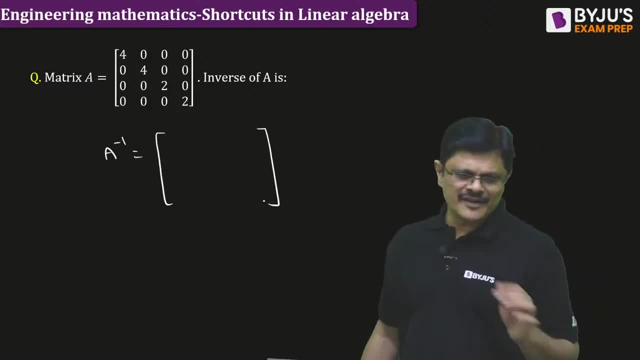 What is inverse of this matrix? What is inverse of this matrix? So, 1 by diagonal. So whenever it is diagonal matrix, inverse is very simple, sir: 1 by 1 by 4, 1 by 2,, 1 by 2.. Of course determinant should not be 0. That is product of main diagonal. 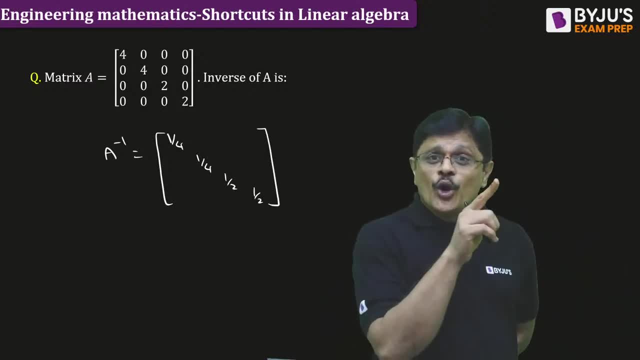 should not be 0, or in other words, no diagonal element should be 0.. No main diagonal element should be 0. That is the condition. What is that 1 by 64 Babu? What is that 1 by 64 Babu? 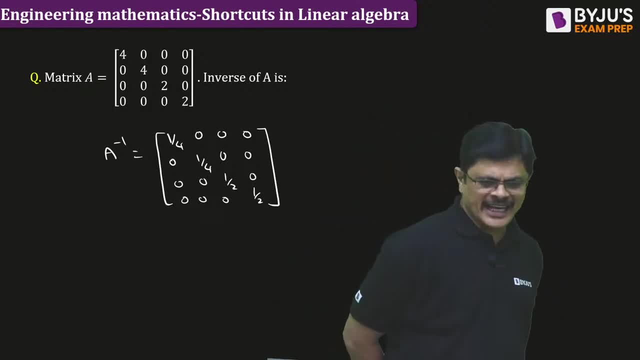 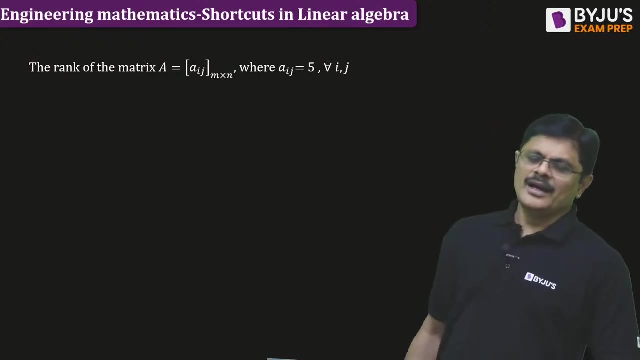 Are you giving determinant of this? A inverse? Are you giving determinant of A inverse? Okay, maybe Nice. Now let us see some interesting ideas for rank of a matrix. Rank of a matrix is number of non-zero rows in echelon. form of a matrix. Rank of a matrix is number of non-zero rows in echelon. 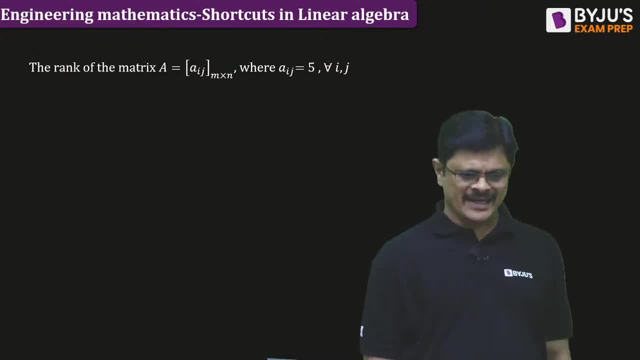 form of a matrix. So here, if you are having this particular matrix where all the elements are same, When all the elements of the matrix are same, actually, if you write this also, you get, like this: 5, 5 and so on, 5,, 5, 5 and so on, 5,, 5, 5 and so on, 5. Suppose if all the elements 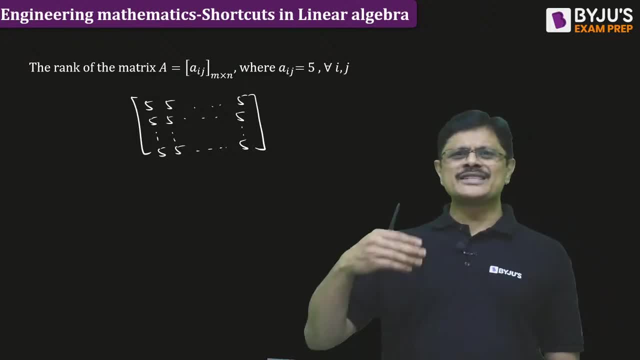 are same. what you can do is because they are all same rows. all the rows are same. You can actually do row 3, row 2 is row 2 minus row 1, row 3 is row 3 minus row 1, instead of doing it. 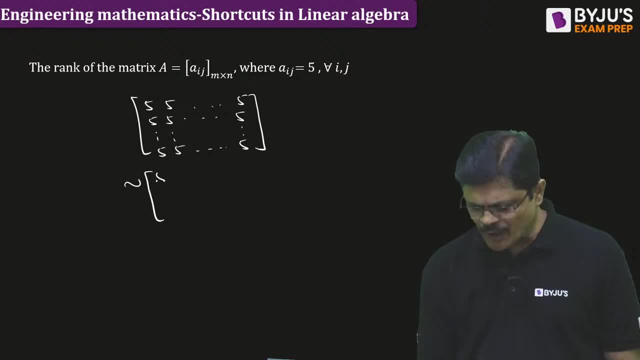 because obvious, We observe that and what we do is we hold one row, that is, we keep one row and make all other rows 0.. Make all other rows 0.. See, actually internally we are doing this row operation, only Internally. we are doing row operation only Internally. 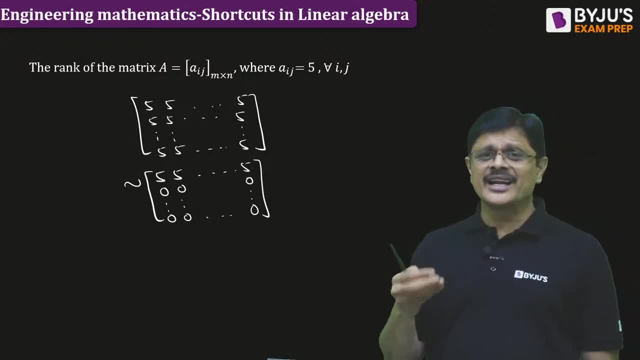 you are using row operation only Internally. you are using row operation only. I mean clear, but by observation what I am doing? Rows are all same. Keep one row, make all other rows 0.. And what is it? It is echelon. 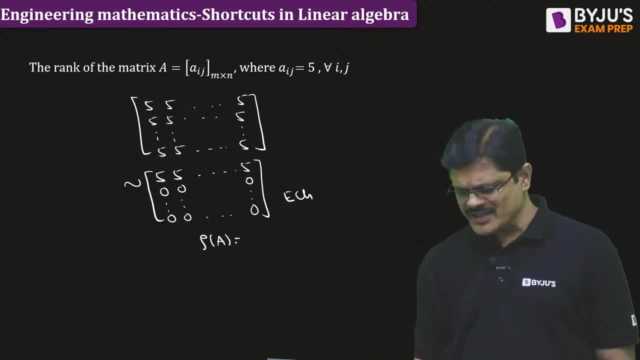 form. How many non-zero rows are there One. so rank is 1.. So whenever you find all the elements are same, rank is 1.. Whenever you see all the elements are same, rank is 1.. Rank is 1.. Say sorry to other rows. Keep one row. say sorry to other rows. 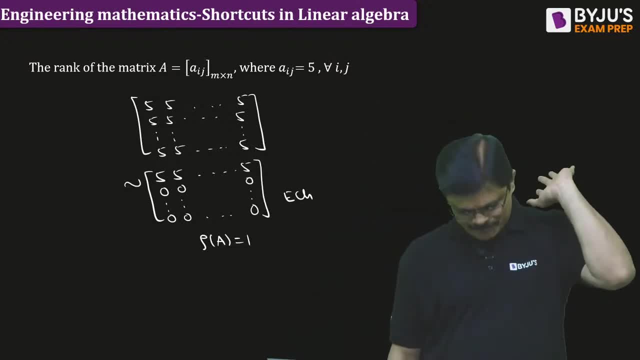 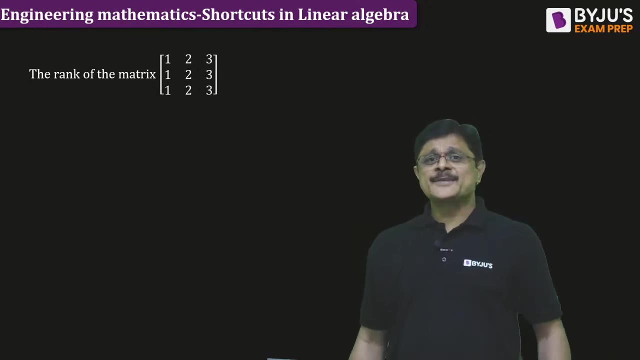 Ek row ko bachao, baaki rows ko bhagao. Okay, Right, Clear, Clear to you all. Hope you understand. Aur ek situation hai, isme kya ho raha hai. all elements are not same, but all rows are. 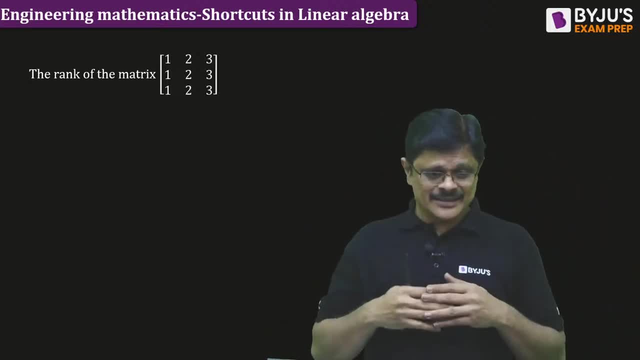 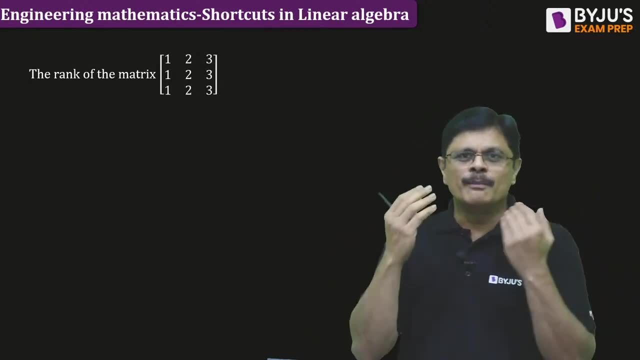 same Rows are identical. Jab rows identical banjate hai, isme bhi ek row ko bachao, baaki rows ko bhagao, Yani 0 banao. Keep one row and say sorry to other rows. Say sorry to other rows, Keep one row, say. 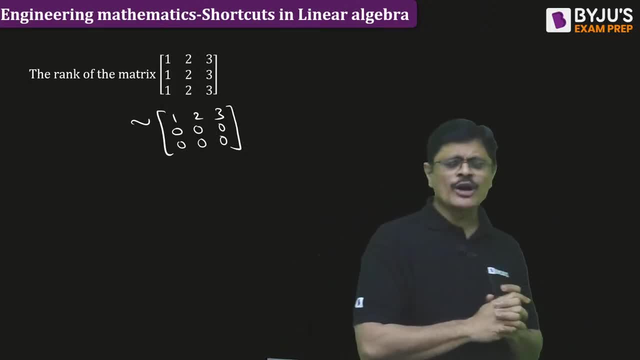 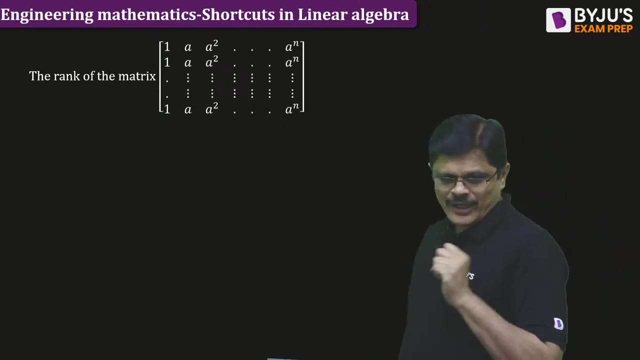 sorry to other rows, Ise kya hoga. Echelon form aa gaya hai. You got echelon form and rank of the matrix ho gaya hai: 1. Super. This was gate question long, long ago once upon. 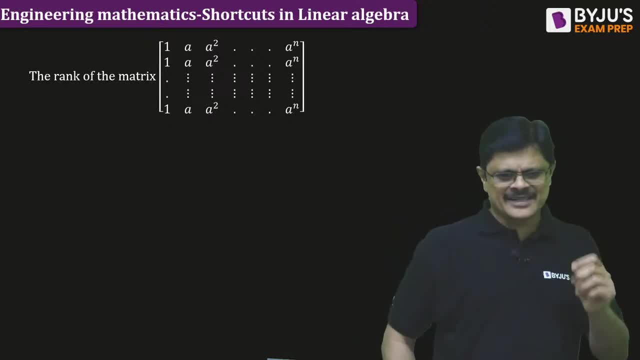 a time. Okay, And what is the rank of this matrix? What is the rank of this matrix? Rank of this matrix is 1.. See, here also all rows are identical. So rank of a is 1.. Ek row ko bachao baaki. 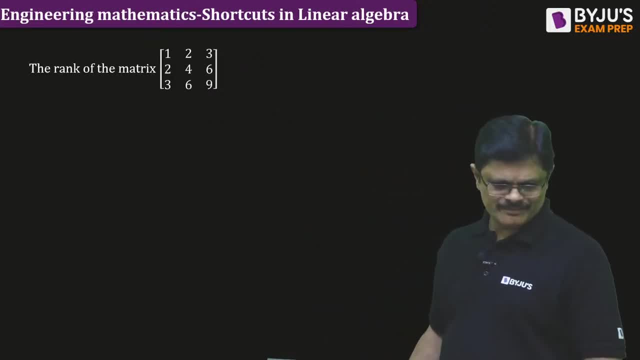 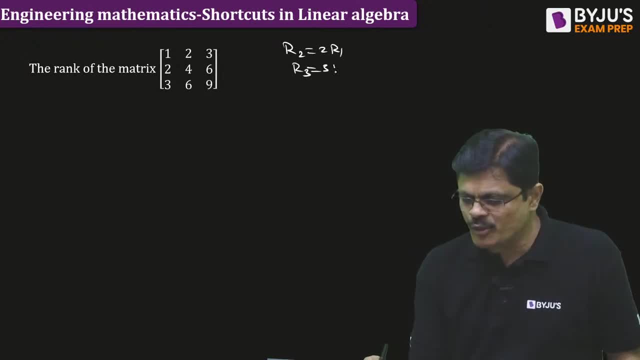 two times of row one third row is three times of row one. so whenever you see rows are proportional, see, i'm saying all the rows are proportional. see, some people misunderstand this. if they find two rows are proportional, they apply this. that is bomb blast my dear friends. okay, you will be the. 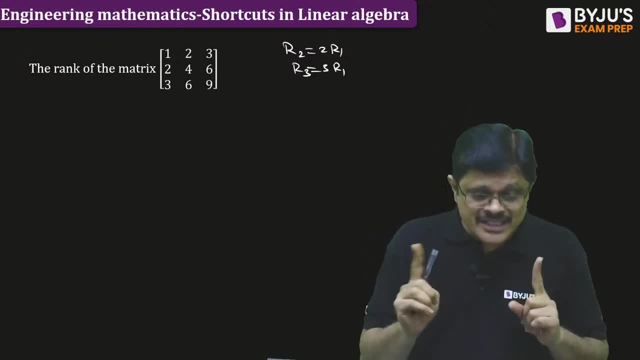 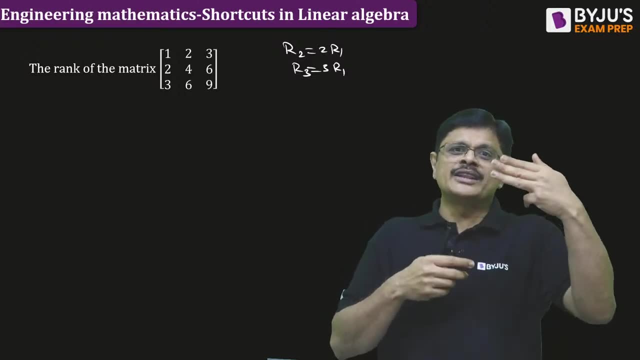 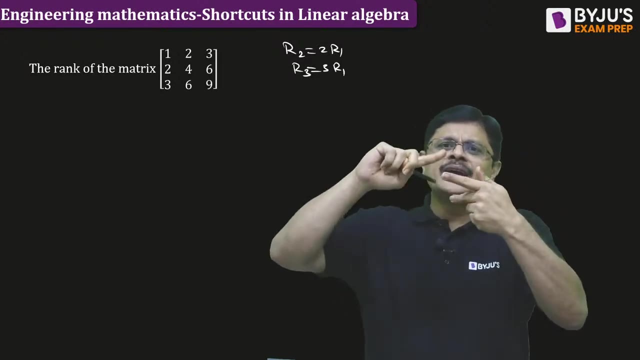 biggest victim. please remember, don't do such things. when i say rows are proportional, means all the rows are proportional, not one, two. suppose only three rows are proportional. suppose it is five by five. three rows are proportional. two rows are not proportional in this three. keep one and make others zero, but don't mess up with the other rows which are 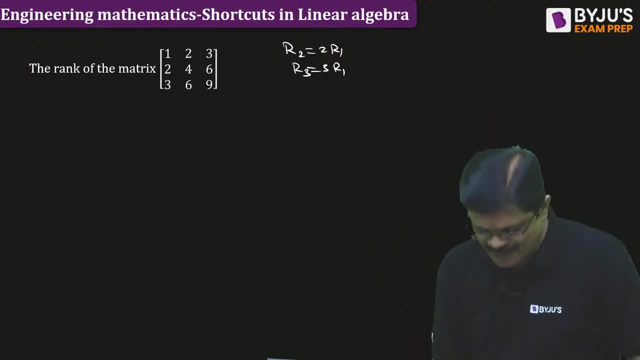 not proportional, not depending on these fellows, am i clear? ah, you'll go to the nearest jail. so what happens? keep first row and make other rows. hope you understand like that. so rank will be still one. my dear friends, these are all shortcuts for rank. now the eigenvalues, eigenvectors. 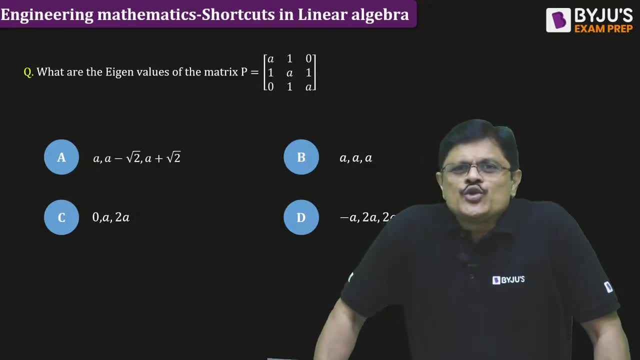 eigenvectors. there are so many properties. actually those who understand the properties, all the problems from eigenvalues eigenvectors are mostly like shortcuts. the properties are shortcuts for eigenvalues eigenvectors. the most famous properties: trace of the matrix is sum of eigenvalues and determinant of the matrix is 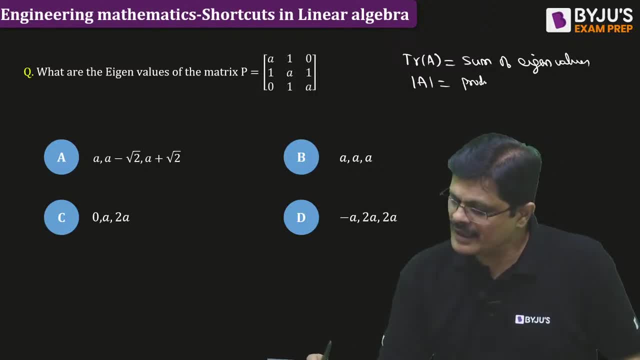 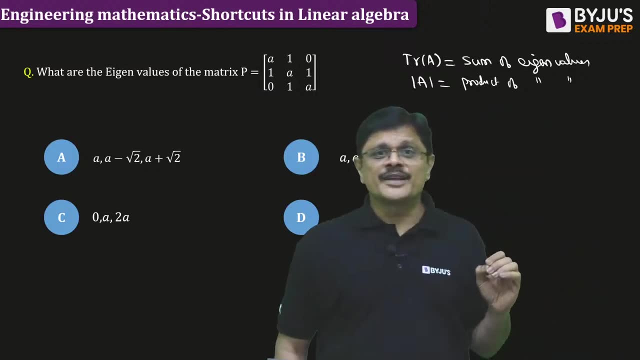 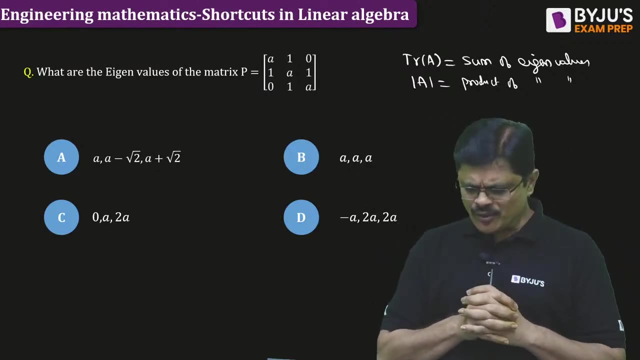 What Product of eigenvalues. Trace of the matrix is sum of the eigenvalues. Determinant of the matrix is product of the eigenvalues. So, those who understand this, how you get 3 to 5 Babu, What is that 3 to 5? For previous problem, or what Susharsthi showed you? which? 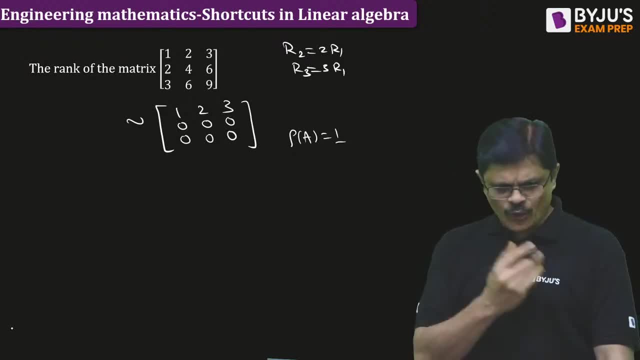 problem you are doing. I think you are doing slowly. You are doing things very, very slowly, Nice. So what happens in this particular case, my dear friends? What happens in this particular case? Rank of the matrix. What is rank of the matrix, my dear friends? I? 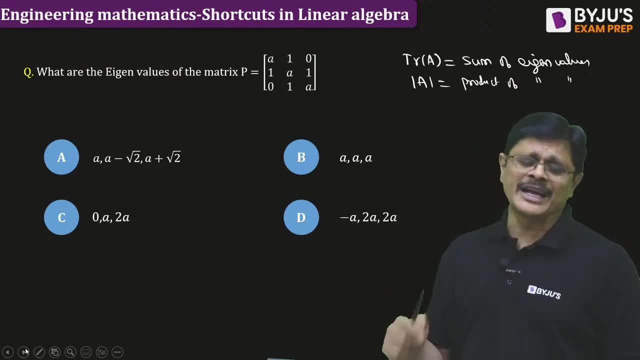 am sorry, Not rank, I am sorry. What is determined? I mean, what about the eigenvalues of this matrix? It cannot be 3 to 5,. sir, A, A, A are given now. So suppose you have 3 to 5.. So what happens in this particular case? You have 3 to 5.. 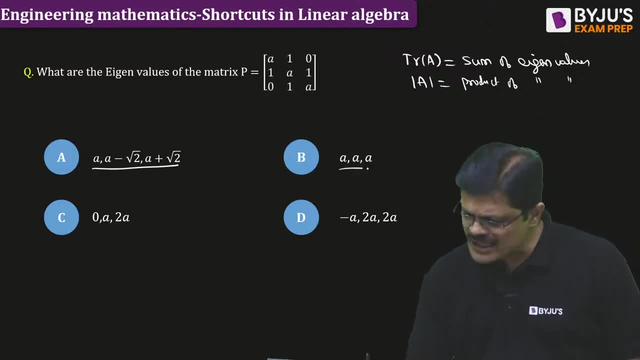 Suppose if these fellows are eigenvalues. if these fellows are eigenvalues, their sum must be equal to trace. And what is trace of this matrix here? Let us find what is trace of this matrix. Trace of this matrix is 3a. What is determinant of this matrix? The determinant: 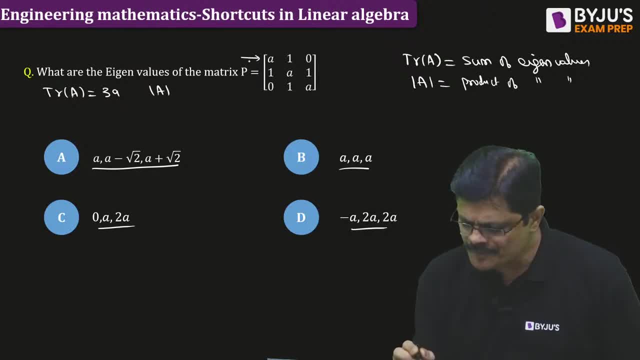 it is better to expand along the first row. So what is it? a into a square minus 1 minus 1 into a, That is a cube minus 2a. That is your determinant, my friends. a cube minus 2a is the determinant. So if these fellows are eigenvalues, their sum must be equal to 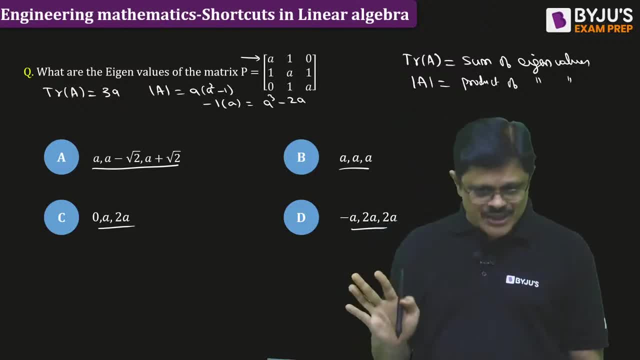 3a and their product must be equal to a cube minus 2a And if you see, product of these fellows is 0, so it is ruled out. Product of these fellows is minus 4a cube. therefore, this is ruled out, Product of these fellows. 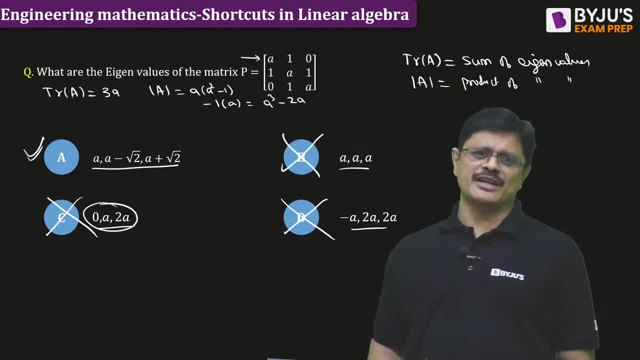 is a cube. this is ruled out. only this fellow satisfy that, that is, their sum is equal to 3a. if you add them, you are going to get 3a, and if you multiply them, you get a cube minus 2a, my dear friends. a cube minus 2a, my dear friends. so correct option is a, and this is wonderful. 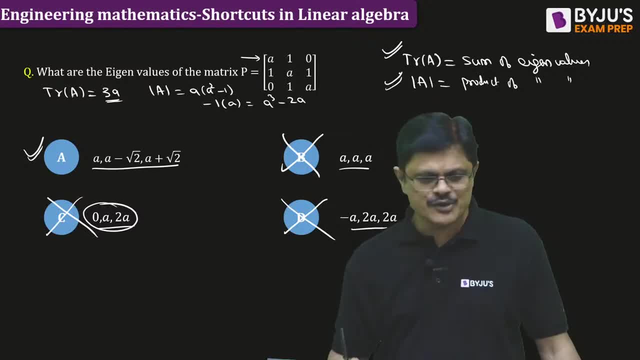 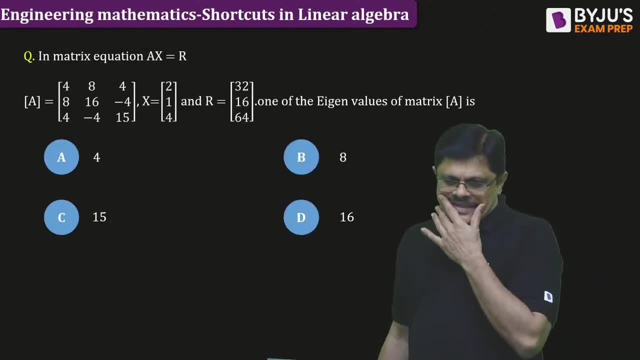 technique and for that this is the most beautiful result which we are going to use. this is the most beautiful result which you are going to use. see, in eigenvalues, eigenvectors. people always apply properties, but they forget the main rule, that is, the definition of eigenvalues and eigenvectors. the definition of eigenvalues. 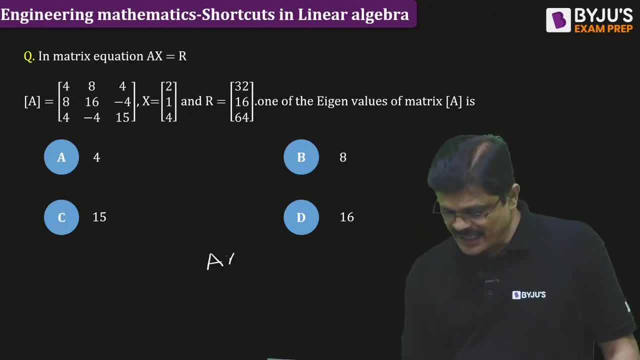 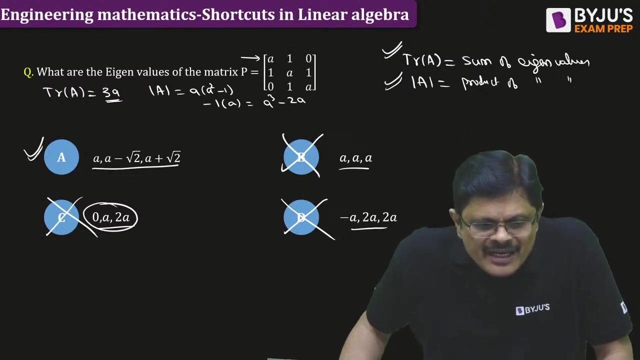 eigenvector. they forget. and the definition is: a x is equal to lambda x. this is the most important definition, my dear friends. so this is actually the definition of eigenvalues. eigenvector. dear ravi shankar krithi, if you want to find eigenvectors for each eigenvalue, you have to 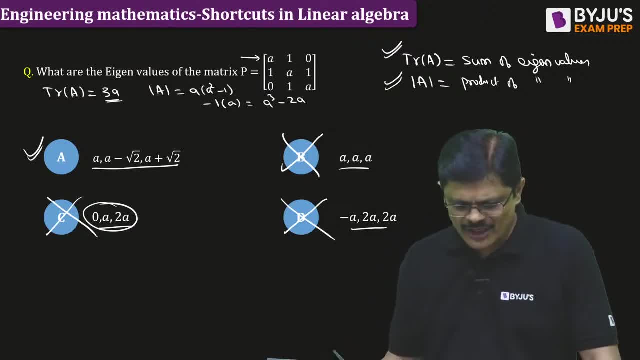 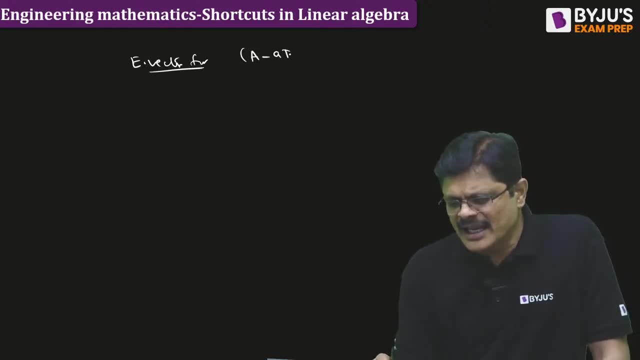 separately solve the problem. am i clear? you have to separately solve the problem. for example, if you want eigenvector for a, you have to solve a minus a. i into x is equal to g, which is also similar to g, which is 0, and then you have to One minus one. nx Does 0 and 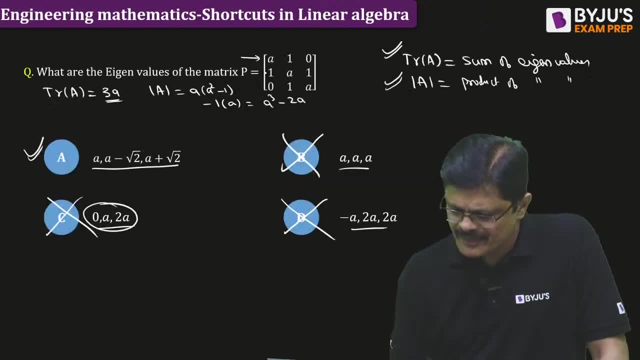 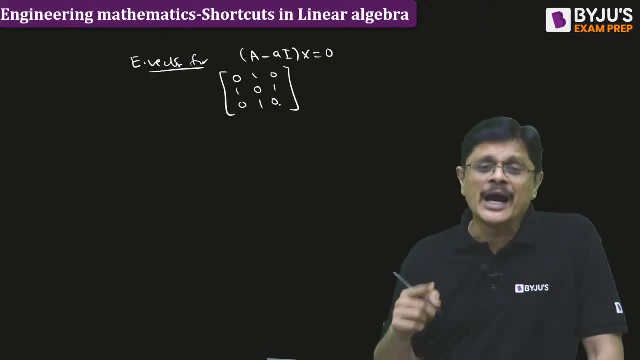 zero plus 0 equal to 0. that is homogeneous linear system you have to solve. so that would be something like 0 0 0, 1 0, 1 1 0 1. so this, if you simplify, you have to get Ledger vector. 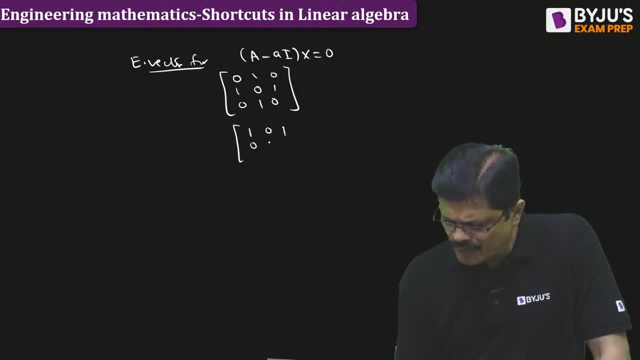 so far. so far you can get the eigenvector very easily. these two are identical to one of them. you can make 0, you can take to top of it, you can make one of these rows: zero n is equal to 3.. So number of linearly independent. what do you call dimension of? 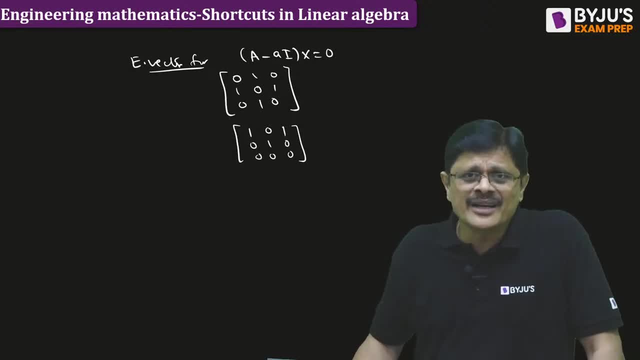 the null space will be equal to n minus r, that is 1.. Only one eigenvector is possible. So these are the basic variables you are going to get. So free variable is z. Let us take z is equal to alpha. So if you write the first equation you get x is equal to alpha, y is equal. 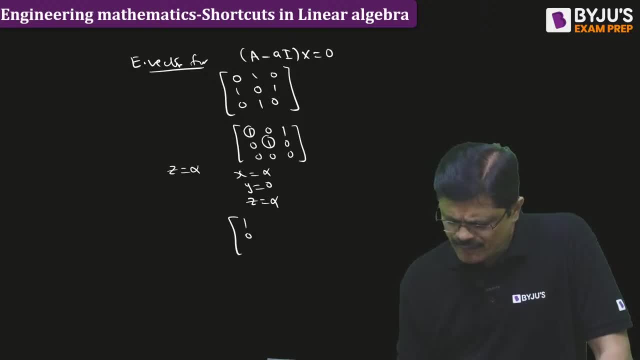 to 0,. z is equal to alpha. With that you are going to get 1, 0,. 1 is one eigenvector. Similarly, this is eigenvector for a, For a minus root, 2. also you have to do the procedure: A plus root. 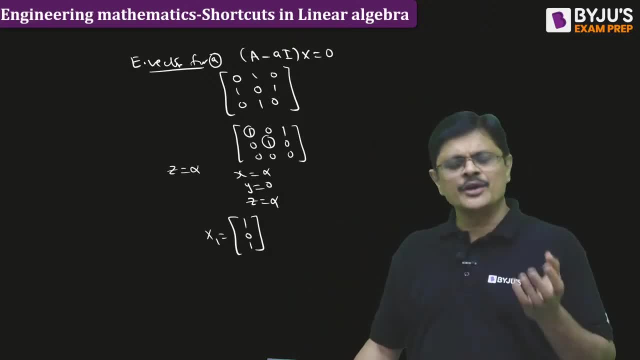 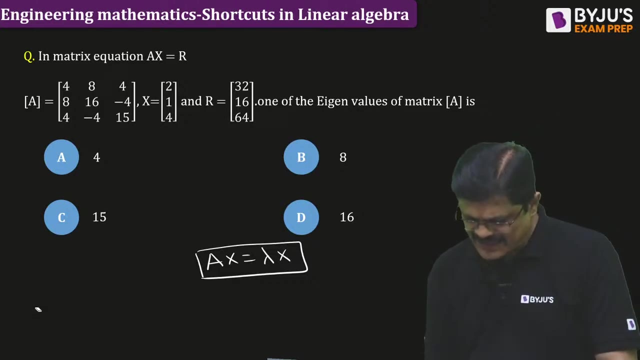 2. also, you have to do the procedure, my friends. By that procedure you are going to get the answer. By that procedure, you are going to get the answer. Am I clear? It is not that it is difficult time taking process, That is nothing more. Now, never forget this basic definition of. 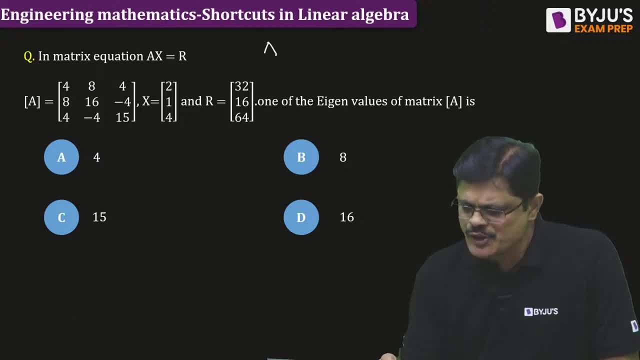 eigenvalues, eigenvector, my friends. So first thing which we should know is a x is equal to 0. So if you write the first equation you get a x is equal to 0.. So if you write: 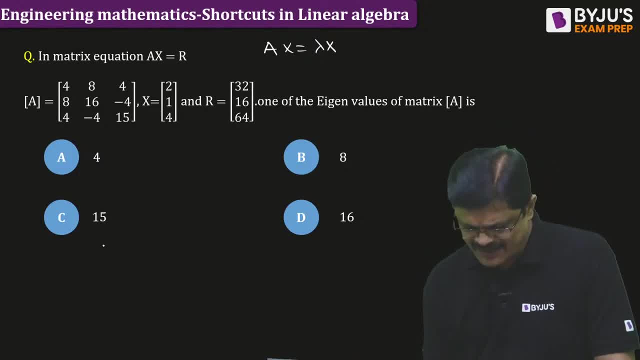 the second equation you get a x is equal to 0. So if you write the second equation, you get a x is equal to 0. So if you write the third equation, you get a x is equal to lambda. x is the definition. So here a x is given, So a why to write a again, sir? Let? 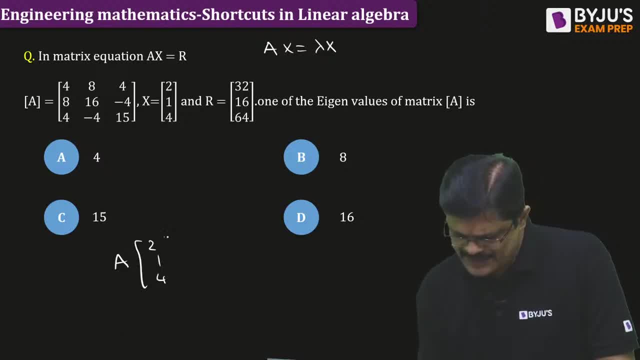 me just write a. only a into x is equal to r, But r can be written as: by taking 16 common, you can write it as 2 and 4.. By taking 16 common, you can write it as 2 and 4.. That. 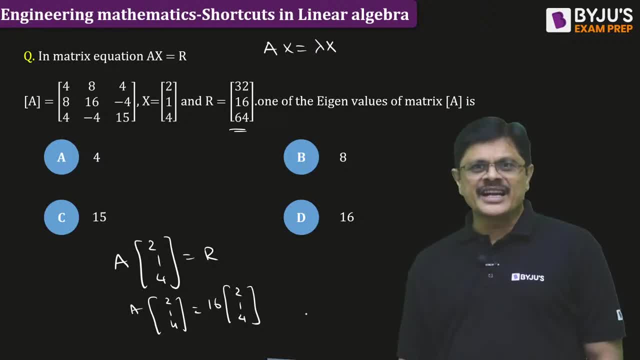 means a x is given by a. So in this definition we are going to get, a x is equal to 2 and 4.. AX is equal to 16X. That means eigenvalue is 16,, my dear friends. Eigenvalue is 16,, my dear friends. 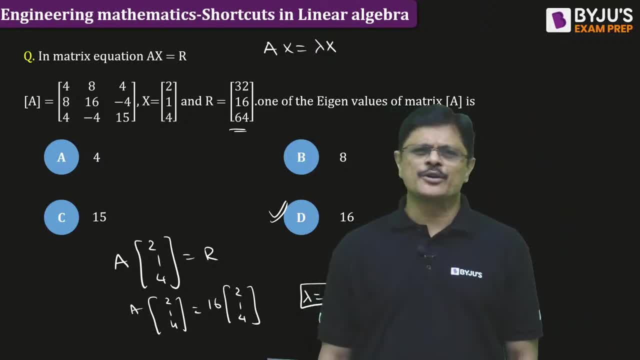 Am I clear? See, it is a very silly, simple problem, basic question, But still, people do many mistakes in this, my dear friends. That's why I just taken this very, very simple problem here. That's why I taken very, very simple problem here. 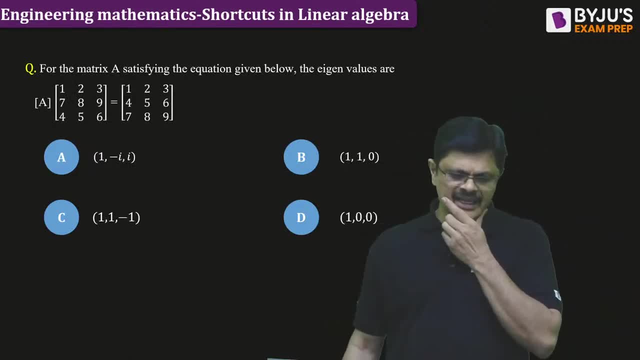 Now this is wonderful question which was asked in GATE. Can you tell me the answer for this? Can you tell me the answer for this? He says: matrix A into this matrix is equal to another matrix. Then what about the eigenvalues of A? 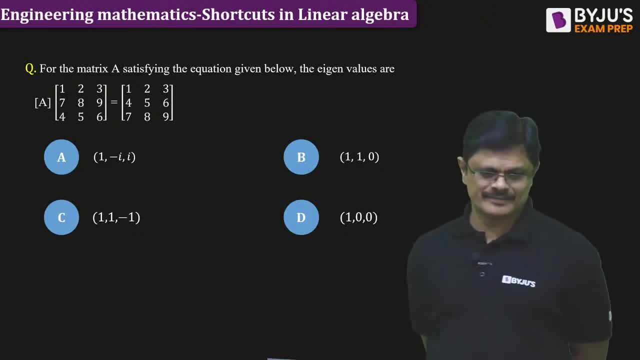 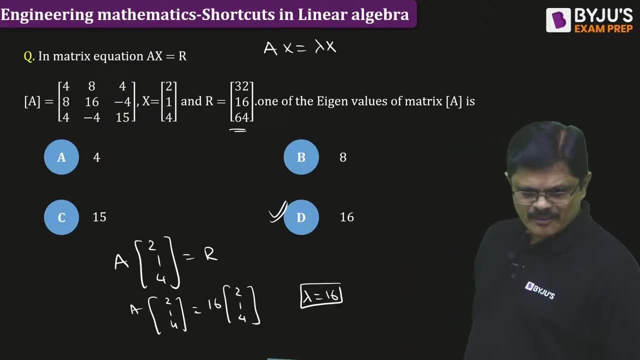 A is not given, sir, A is not given. D is a wrong answer. Is it for last one, Kumari? is it for last one? Last one, 16.. But this one, what is it? What about the answer for this? 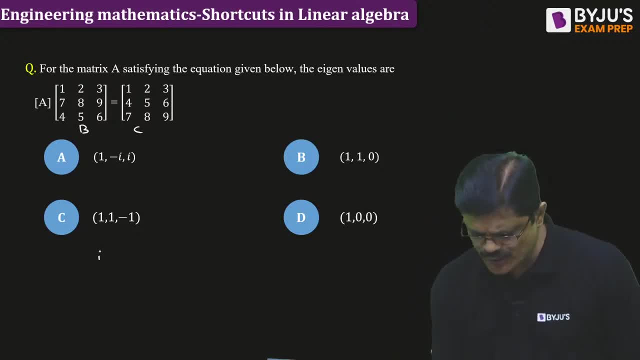 So for time being, let us call it as B and let us call it as C, sir. So you got A into B is equal to C. You got A into B is equal to C. you have Let me tell you one very interesting story here. 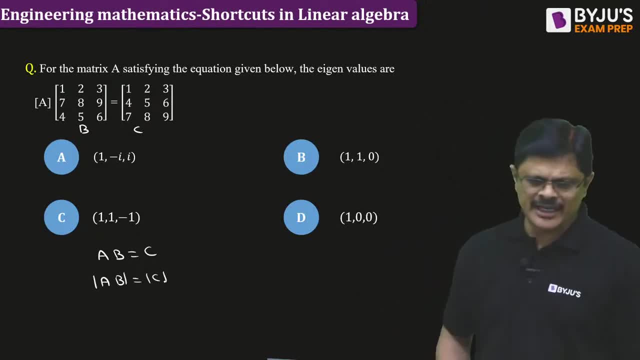 Det A- B is equal to det C. If I apply determinant A, B is equal to det C. But you know, determinant of A- B is equal to det A. into det B, That is equal to det C. Ravi Kumar Kiriti. 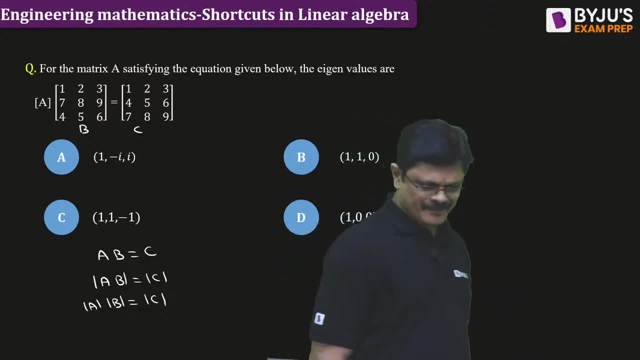 it is wrong answer for this. A is wrong answer. A is wrong answer. Now, if you observe B and C, what is, My dear friends, if you observe B and C? Actually, if you observe, C is obtained by interchanging two rows of B. 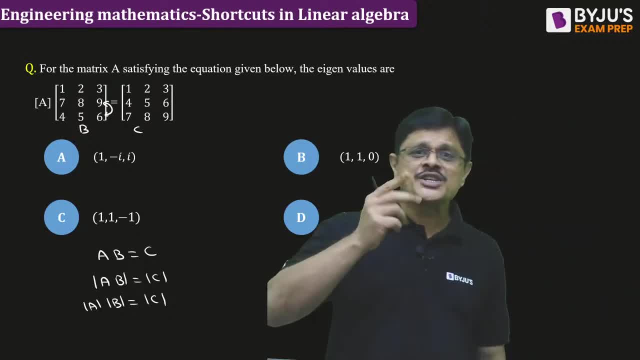 C is obtained by interchanging two rows of B. What happens if you interchange two rows? What happens to determinant if you interchange two rows? What happens to determinant if you interchange two rows? That is, on matrix B, if I interchange second row with third row? 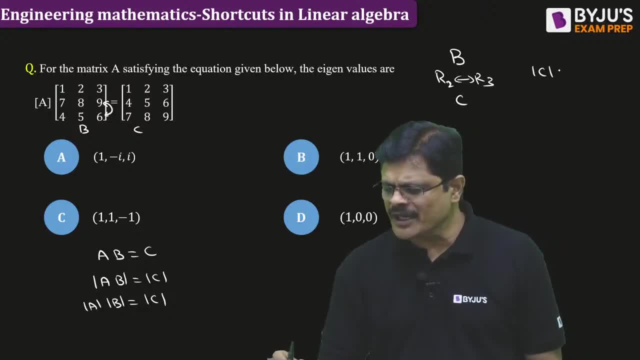 Then I got matrix C. Then what can you say about determinant of C, my dear friends? What can you say about determinant of C, my dear friends? No, Pranap Paul. When you interchange rows, determinant sign will change. Determinant sign will be minus. 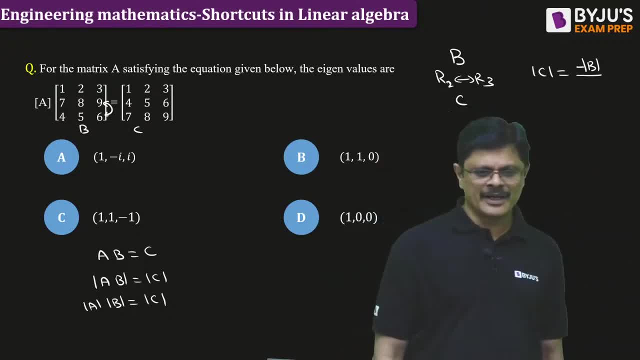 Negative sign: Payash Kumari. good Pranap Paul. what happened here? Minus Minus B. So we know that determinant of B and determinant of C are minus of each other. That means what Determinant these two cancel with minus 1 sign. 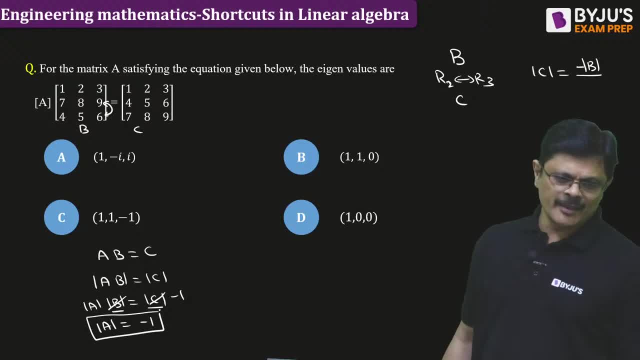 So determinant of A is minus 1.. Determinant of A is minus 1.. Now, determinant of A is minus 1 means you know that determinant of A is product of eigenvalues. Product of eigenvalues. So identify if these are eigenvalues. 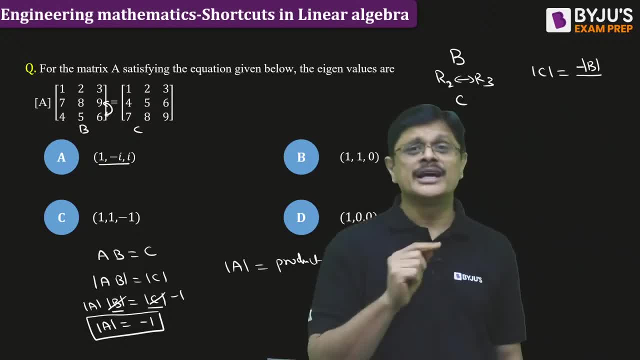 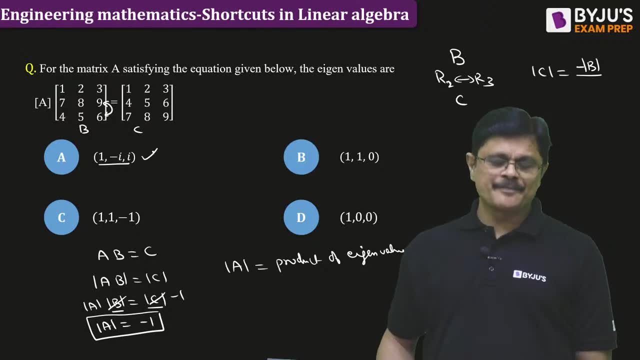 Their product must be equal to minus 1.. If these are eigenvalues, their product must be equal to minus 1,, my dear friends. So product of these fellows is what, sir? Minus I square, Minus I square is plus 1.. 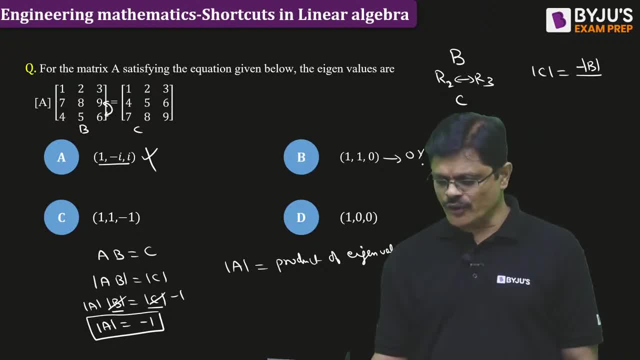 So this is wrong. Product of these fellows is 0.. So wrong. Product of these fellows is minus 1.. And product of these fellows is 0, wrong. So correct answer is option C, my dear friends. So the correct answer for this problem is option C, my dear friends. 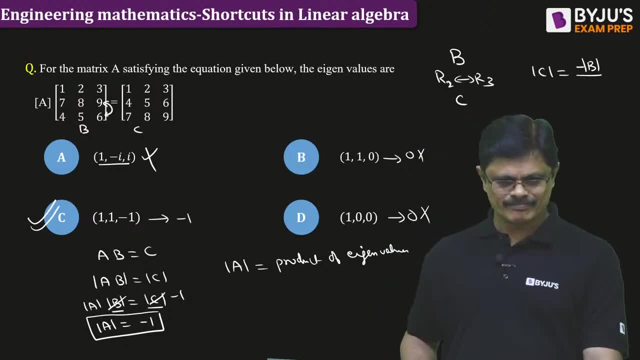 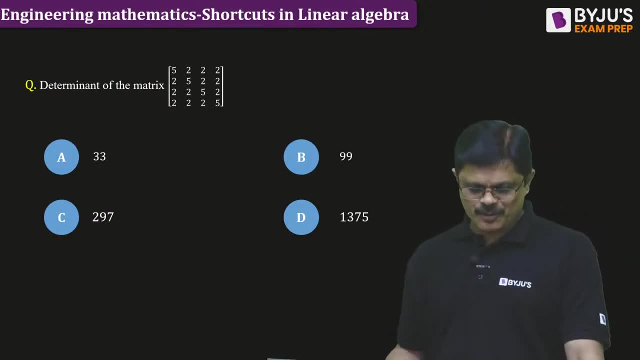 Next problem: What is determinant of this matrix? What is determinant of this matrix, my dear friends? See, we are having a matrix which is a 4 by 4 matrix. What is determinant of this? Of course, you can use our regular techniques. 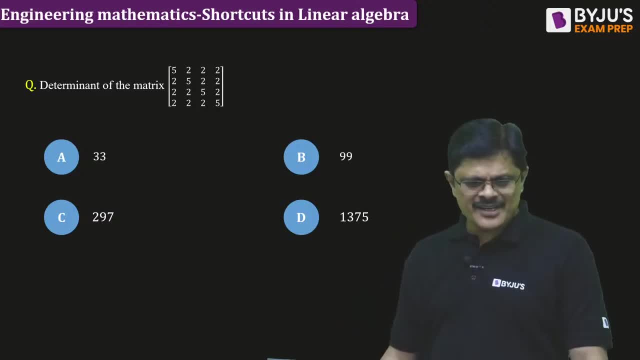 but there is. there is one very interesting way to handle this type of problems. let me explain. you can write this matrix like this: because all of diagonals are tuner, so make main diagonal sort of 0, but that needs you need to get main diagonal: 3 0 0, 0, 0, 3 0, 0, 0, 0, 0, 0, 3, 0 and 0 0 0, 3 sub. okay, so by 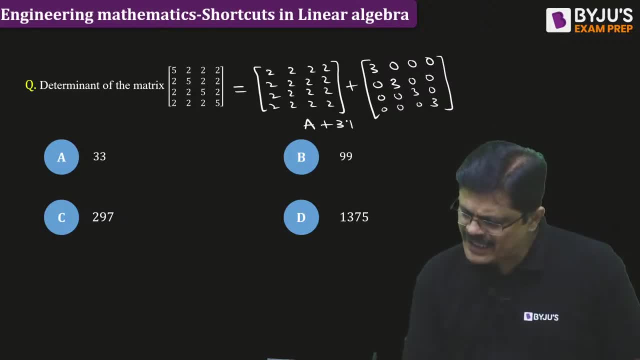 this: what happens? suppose you call it as a, this will be 3. I my difference. okay, suppose? okay, let us call it as B. let us call it as. what happens? let us call it as B- original matrix. let us call it as a. actually, there are some. 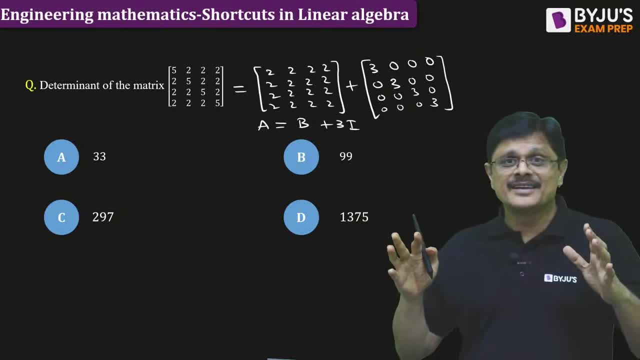 very interesting result. if all the numbers are ones, if all the numbers are ones and it is a n by n matrix, one eigenvalue will be n and remaining eigenvalues will be 0. so for this matrix, the eigenvalues are 4 0 0 0. my difference: for this matrix, the eigenvalues are 4 0 0 0. therefore, 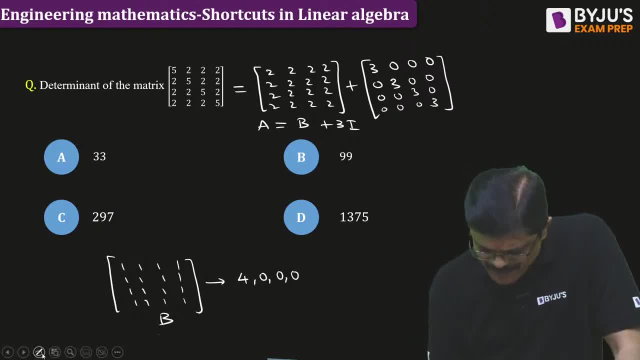 suppose you call it as some B. you call it as some B, then I can call it as some 2 times B. my difference this is 2 times of this. so for 2 B, what will be the eigenvalues? for 2 B, the eigenvalues will be 2 times of this, that is 2, 4, 8, 0, 0, 0. so 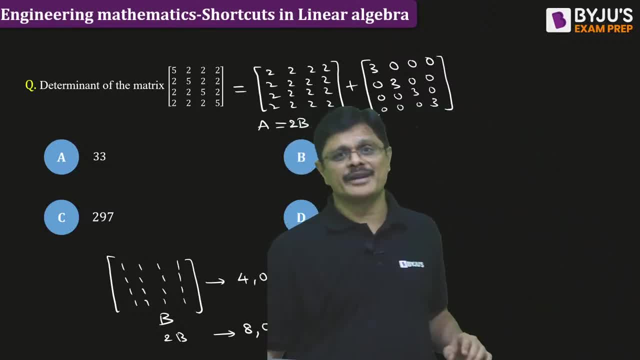 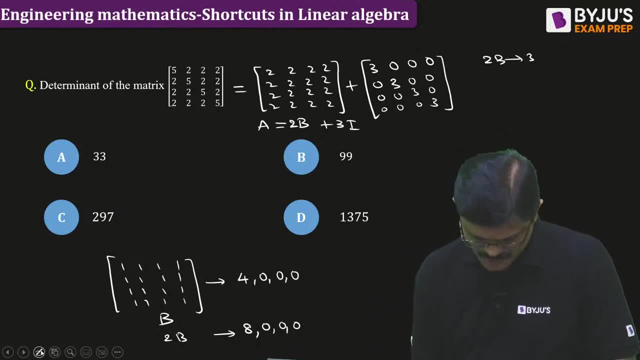 eigenvalues of 2 B will be 8 0 0, 0 by difference. now, once you know the eigenvalues of 2 B, you know eigenvalues of 2 B plus 3, I sorry, 2 B plus 3, I eigenvalues. 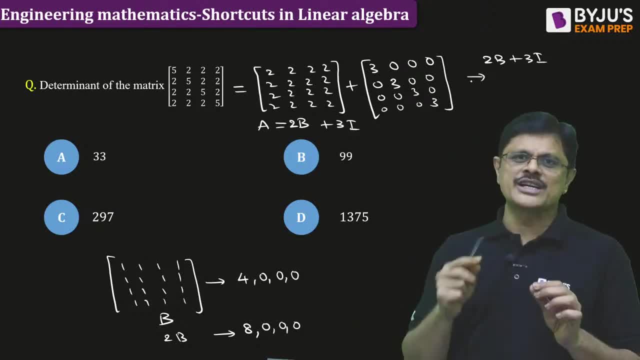 we know, sir, what about the eigenvalues of this? for every eigenvalue just add 3, that is 8 plus 3, 0 plus 3, 0 plus 3 and 0 plus 3, so the eigenvalues are 11, 3 and. 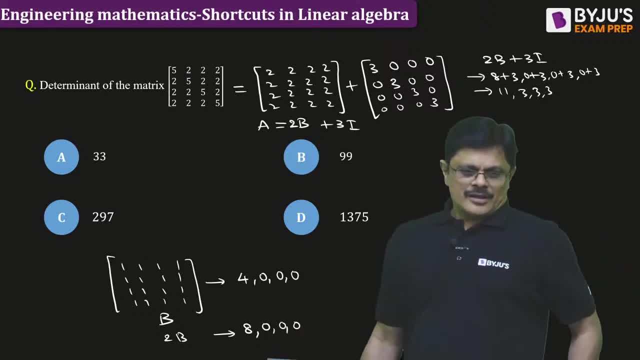 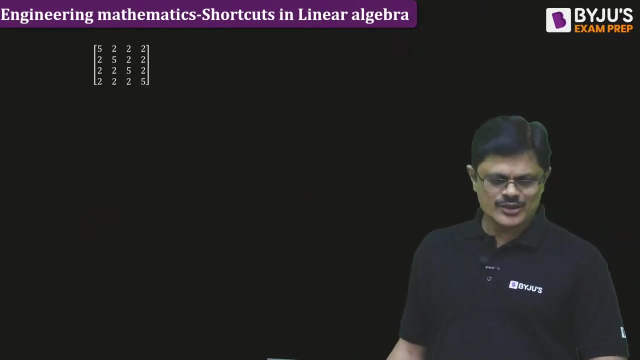 3 and 3. yes, those are the eigenvalues. and he's asking: determinant means product of the eigenvalues. determinant means product of the eigenvalues. you just find product of the eigenvalues- my difference. you just find product of the eigenvalues, my difference- 2, 9, 7, super very good. so that is the idea for this. 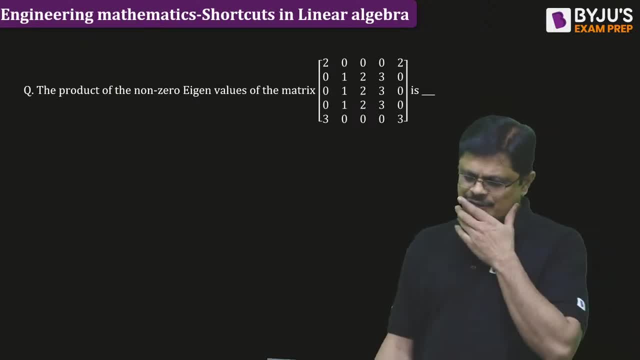 type of problems? my difference. there is one more very interesting question: what is product of non-zero eigenvalue of this matrix? my difference. see, I'll give you a shortcut here whenever you find this type of relation. you see, here we have some 3 by 3 matrix, the corresponding elements in the remaining 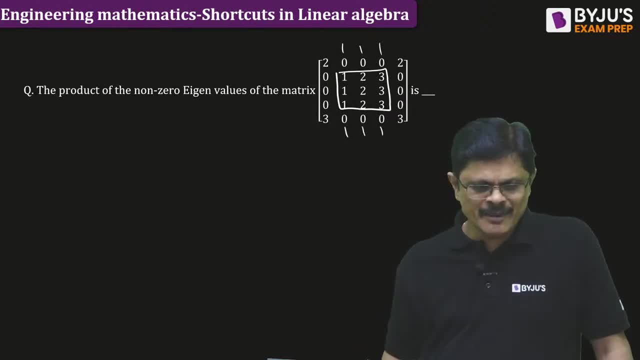 form are zeros corresponding elements in the remaining form. why I change it the numbers? mr Ashok Ashok, I know gate question. I change it the numbers. notice, forgive the mistake. sorry, sorry, sorry, and you can find it, but my difference, whatever you want, it changes by distribution. 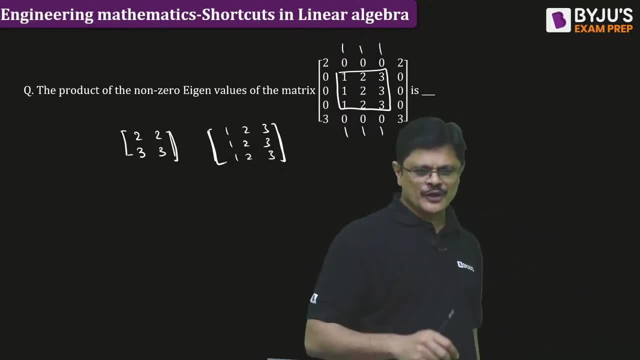 of this matrix separately and product of those fellows will be your answer. okay, i think you already answered properly. even i don't know the answer, sir, i just changed the numbers. it may be correct also, ashok, it may be correct also. don't worry now for this. what are the eigenvalues for this? what are the eigenvalues, sir? 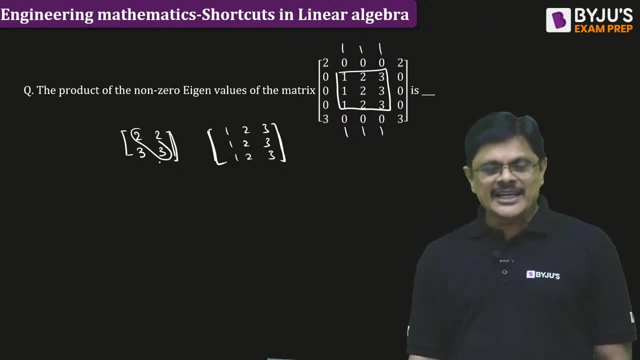 because rows are proportional. determinant is zero, so one eigenvalue is zero. the other eigenvalue is five, so zero. five are the eigenvalues here. because determinant is zero, one eigenvalue is zero. some of the elements in each row is six, that means one eigenvalue is six and third. 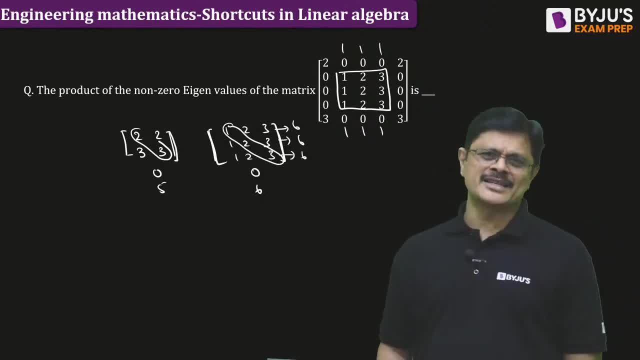 eigenvalue, because some of the eigenvalues must be equal to trace. zero plus six plus some third eigenvalue is equal to six. so what should be the third eigenvalue? third eigenvalue is c. therefore, the product of non-zero eigenvalues will be: the product of non-zero eigenvalues would be: what's a six into five, which is thirty. 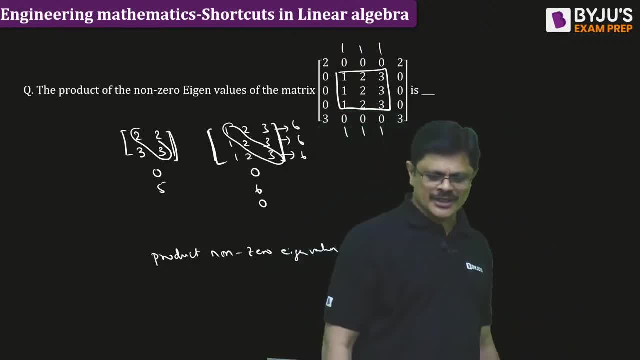 okay, sir. so we covered some interesting shortcuts today. next time we'll try to see some more. my difference, yes, product poll- super. hope you understand. mr ashok, the questions can be changed. sometimes it's not just get questions. if you understand, get questions. questions can be very easily changed. 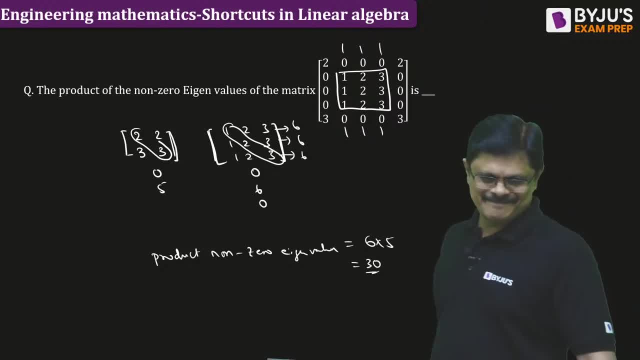 otherwise we have to fix ourselves to get questions. only see, you can do row operations for finding determinant, for finding echelon form, for finding eigenvalues, eigenvectors. don't do it. for finding eigenvalues, eigenvectors, don't do it. which one you want me to repeat, mr? 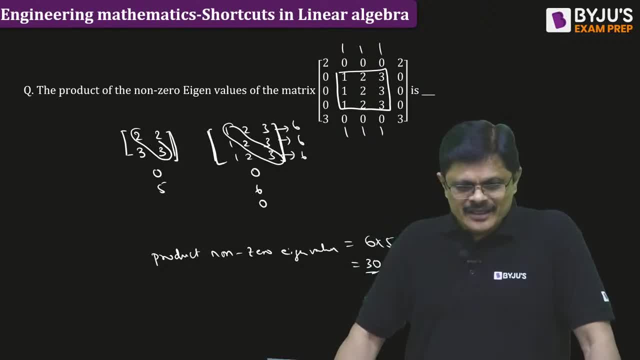 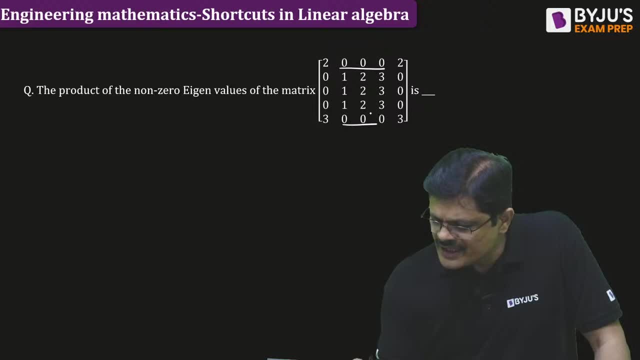 ؟? which one? you want me to repeat this problem. you want me to repeat: see, here, you are having zeros here. so this part is independent of remaining part x. this part is independent of remaining part. what you can do is you can take this as one matrix. 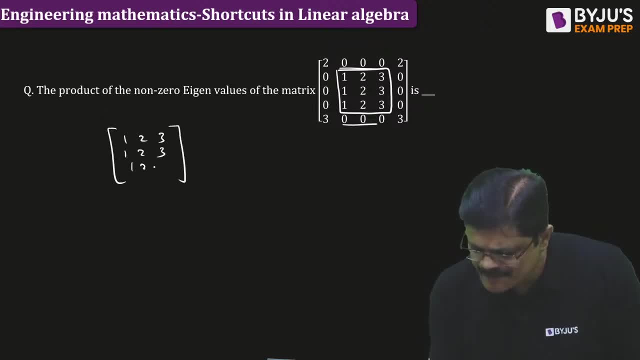 that is the intermediate fellow, as one matrix. the outer part, that is two, two, three, three, that is one matrix, here is matrix. So just find eigenvalues of this problem, eigenvalues of this two matrices. my difference See here, because determinant is 0,. determinant of this fellow is 0, 0 is. 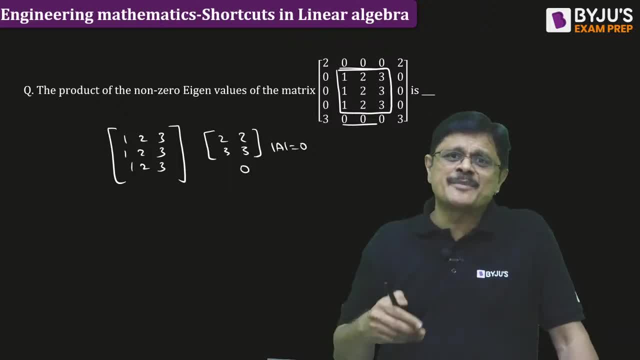 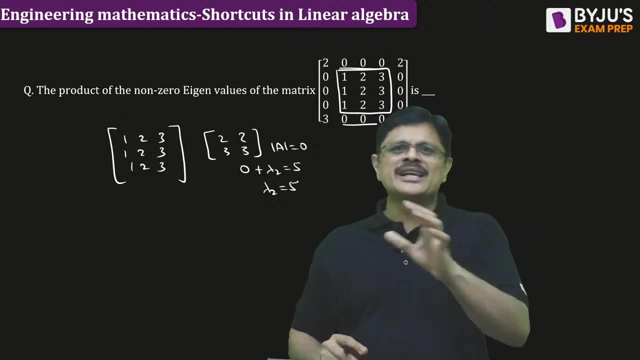 the eigenvalue and some of the main diagonals must be some of the main, that is, trace of the matrix must be some of the eigenvalues. So trace is 5.. So 0 plus lambda 2 must be equal to 5. means what is lambda 2? that should be 5.. So one eigenvalue is 0 means the other. 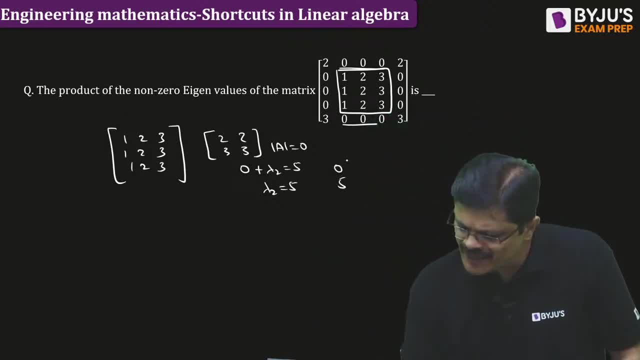 eigenvalue must be 5.. One eigenvalue is 0 means the other eigenvalue is 5. here And in this particular problem, determinant is 0 means one eigenvalue is 0.. Sum of elements in each row is 6 means. that is one more interesting shortcut. If sum of elements in each row or 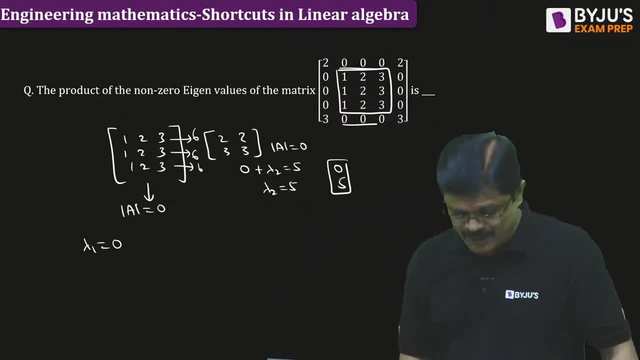 each column add up to the same number. that same number is eigenvalue. So because of that, 6 is another eigenvalue. Now the most important thing is that if you want to solve this problem, you have to find out this very important thing: lambda 1 plus lambda 2 plus lambda 3 is equal to some of 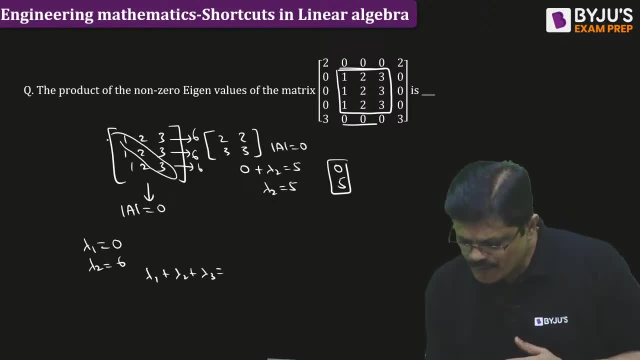 the eigenvalues must be trace. what is trace? 1 plus 2, 3, 3 plus 3, 6. So here it is 0, here it is 6.. So what should be lambda 3.. So lambda 3 is also 0.. So the eigenvalues for: 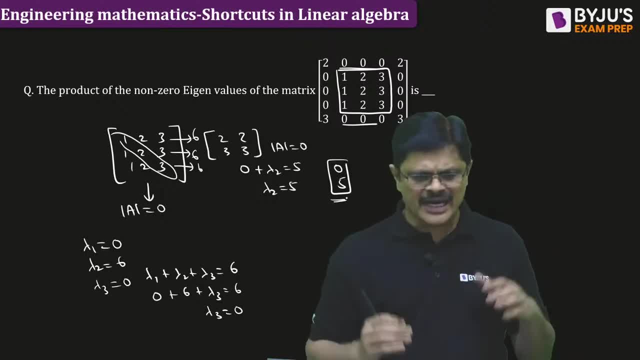 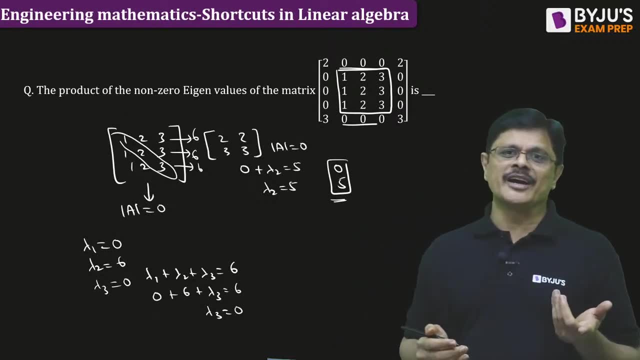 this are 0, 6, 0,. eigenvalues for this are 0, 5.. So what does it mean? the non-zero eigenvalues are 5 and 6.. eigenvalues will be 5 into 6, which is equal to 30 by default. So product of non-zero. 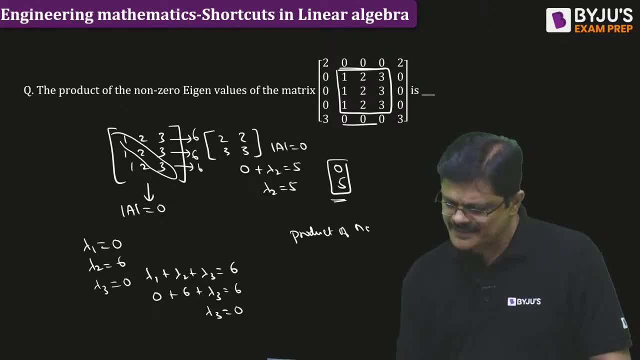 eigenvalues would be product of non-zero. eigenvalues is 5 into 6, that is 30. Hope you understand, So I am stopping here. I thought of doing this shortcut for LU decomposition also, maybe some other time, sir. okay, because I have one more class, So no problem, we. 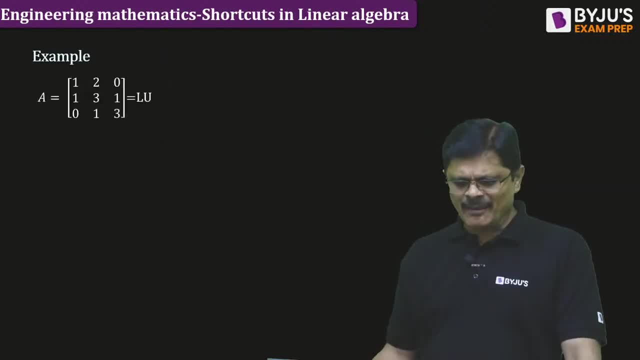 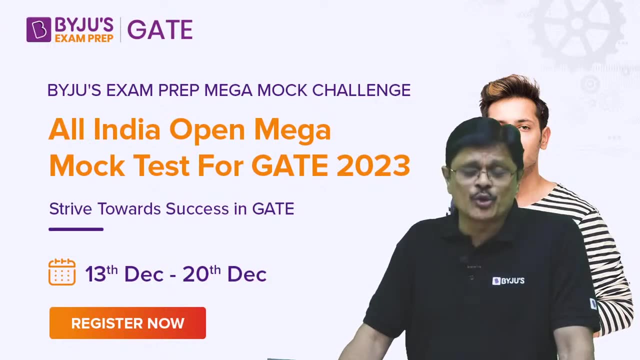 will be coming again, again. So this time I will come up with some shortcut, next time, And you all can take this: All India Open Mega Test for GATE 2023.. It is up to 20th December, my dear friends. okay, The solutions also will be provided in the recorded form. 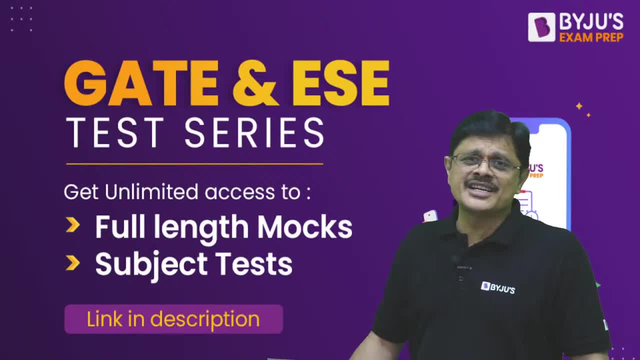 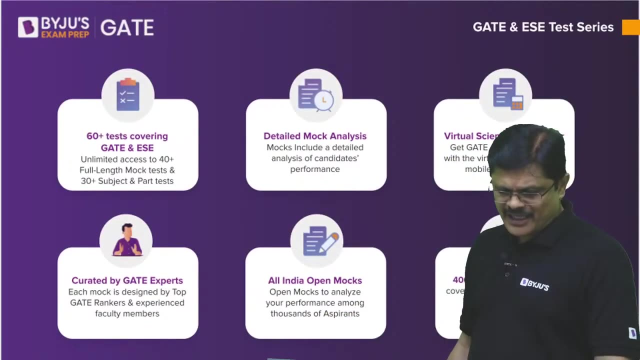 Or live form. my dear friends, Then we have this GATE test series for all the serious aspirants, which is, you know, having full-length mock test for all the subjects, Unlimited access. you can get it And link is in the description. Okay, these are all the details of that particular. 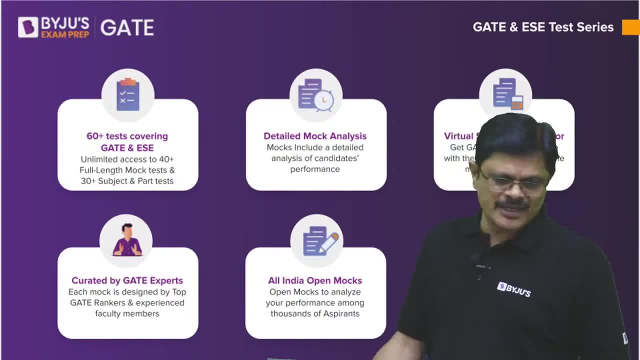 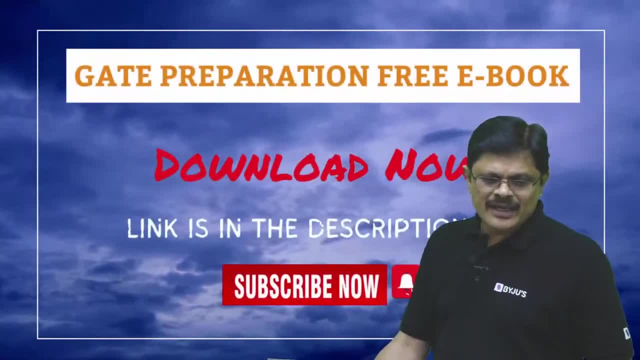 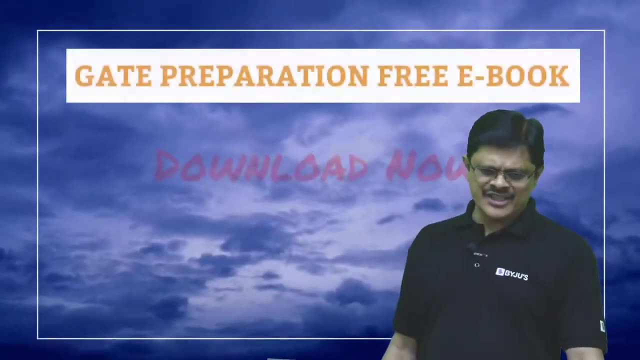 GATE mock test. my dear friends, Okay, sir, thank you very, very much for attending the session And you are also having this free e-books which are available in your. yes. yes, it is there for EC, For all the branches. it is there, Ravishankar Kriti, It is there for all branches. Actually. 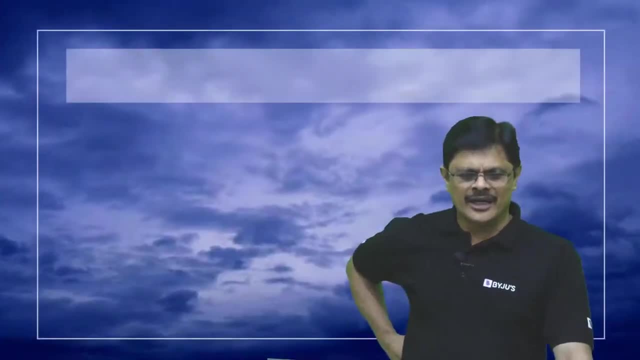 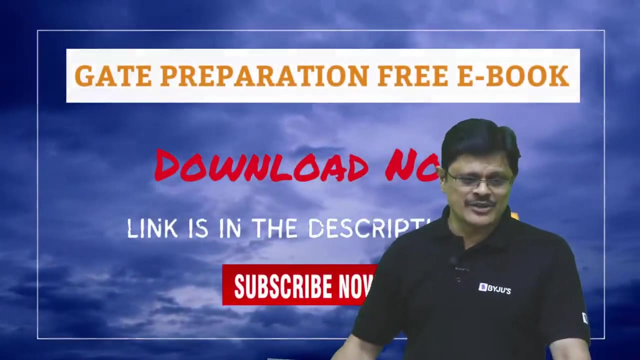 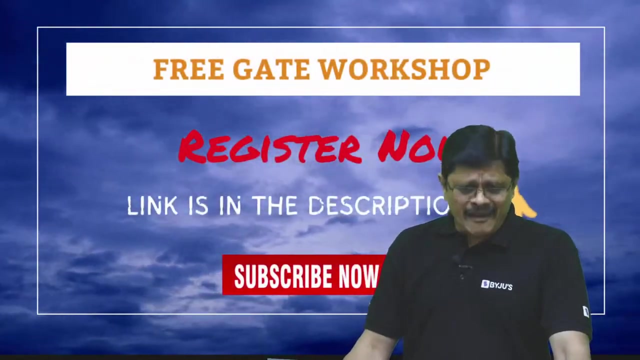 earlier. I done once this LU decomposition shortcut. it is available in your Byju's exam prep YouTube channel. You can see LU decomposition by Sridhar sir in Byju's exam prep where I discussed that completely Here. I just want to quickly recap that. okay, So you are all having.